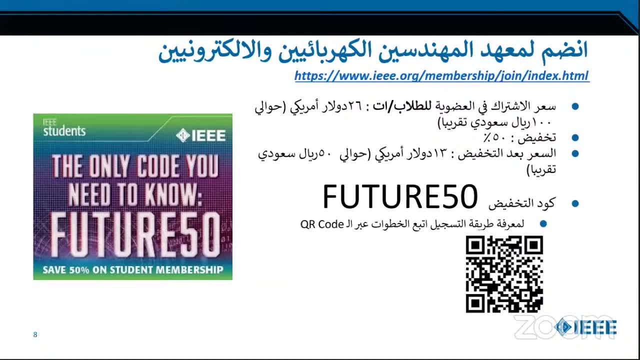 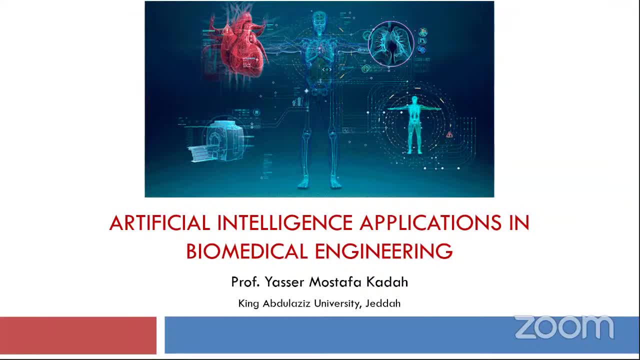 Okay, do you want me to start right away? Take your time, Prof. Okay, let's start, Inshallah, so we don't get late. First of all, Bismillah ar-Rahman, ar-Rahim. 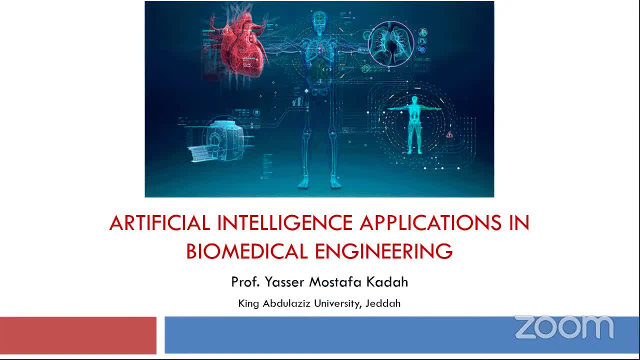 Assalamu alaikum, Our goal today from the seminar is to take a general idea about artificial intelligence, especially in its applications related to biomedical engineering, which is related to health care and other things like that. There are many things that are unique to the application. 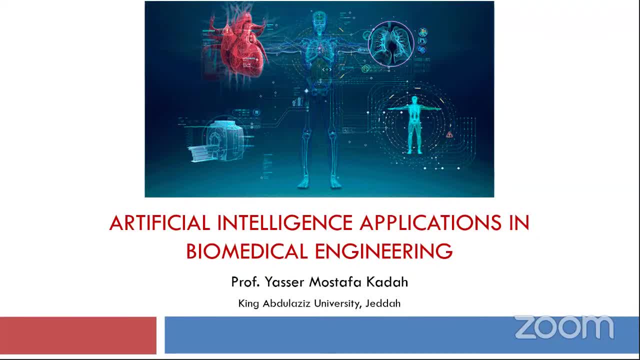 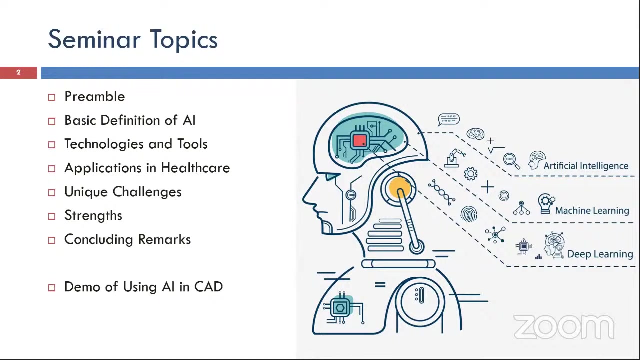 of artificial intelligence for our area. so we have to focus on it, so that, when we enter the subject, we can understand it and appreciate the limitations, so that we can benefit from the ultimate benefit of technology. Inshallah, I will start at the beginning preamble: some ideas. 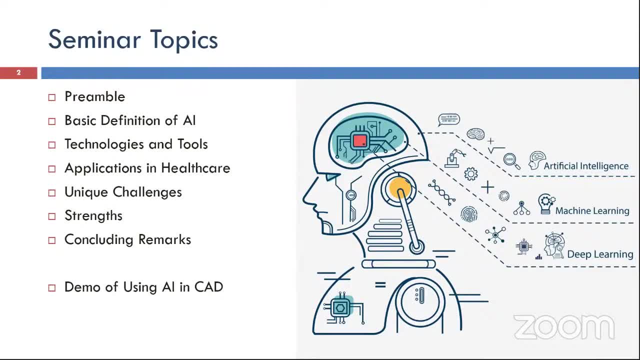 I just want you to have these ideas before we start talking about the subject. They are simple and unique ideas, but you will find them interesting when you start to see the slides. We will talk about the basic definition of AI. We will talk about the technologies and tools involved in this area. 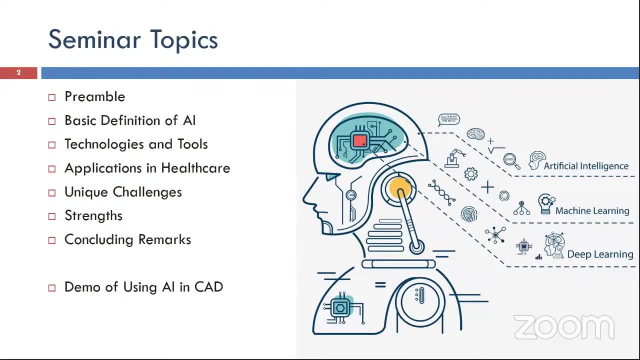 We will talk about the particular applications in health care. We will talk about the particular applications in health care. We will talk about some of the unique challenges that have to do with the technology itself: the legal framework of technology, the regulatory aspects of technology. 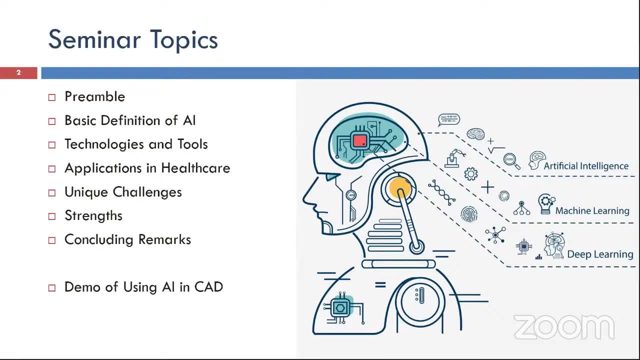 We will talk about the strengths, which are the strengths that have to do with the applications in our field, And, in the end, we will talk about concluding remarks. I don't know if the time will allow it or not, but I was hoping to do a demo of how we use AI. 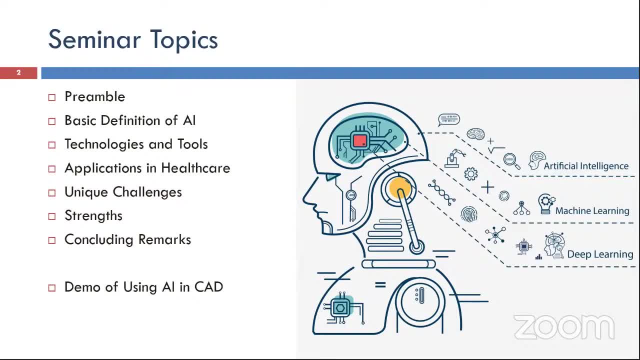 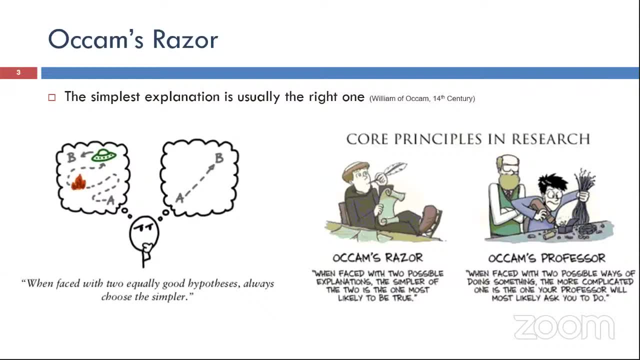 to do the research And then we will do a computer-aided diagnosis. At the beginning, as I said, I want to talk about things that have nothing to do with the subject, but you will feel its importance when we start talking about the details of AI. 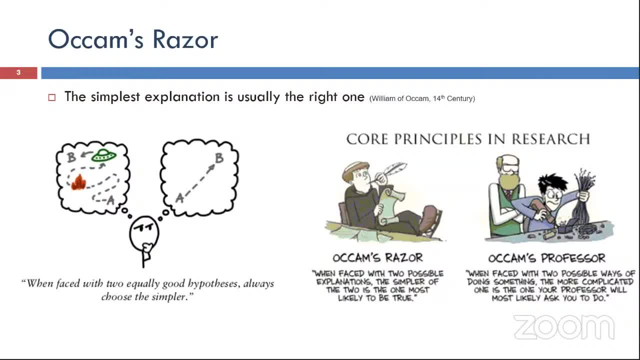 There is a very nice concept called Occam's Razor. Occam's Razor simply says: the simplest explanation is usually the right one. The famous saying is William of Occam. that was in the 14th century Basically the basic idea. when faced with two equally good hypotheses. 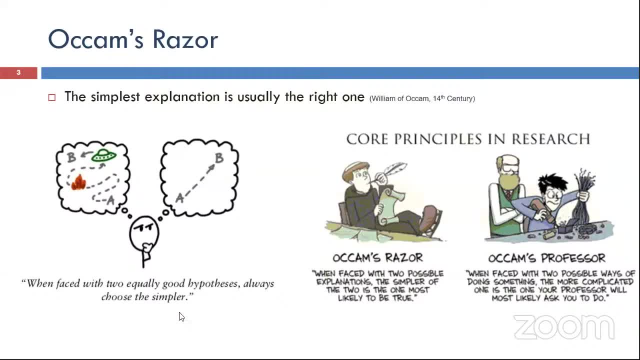 always choose the simpler one. Unfortunately, in the field of scientific research, we will find that sometimes people act contrary to this concept. You will find, for example, some students in the United States, students of research in the United States. they saw the Occam's Razor and suggested that there is something called Occam's Professor. 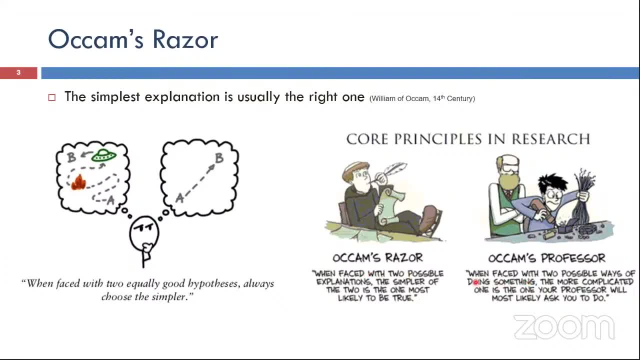 Occam's Professor is completely the opposite of Occam's Razor. He says: when faced with two possible ways of doing something, the more complicated one is the one your professor will most likely ask you to do Okay. So of course we are talking about. 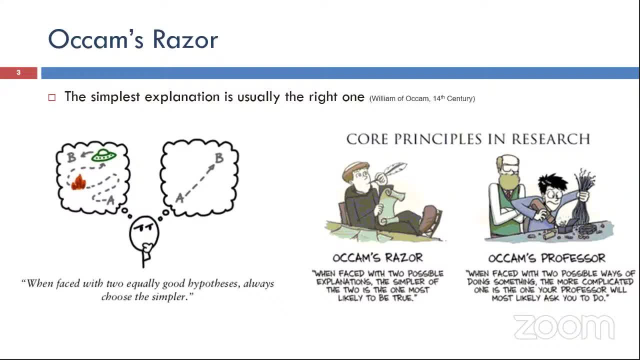 unfortunately, in the field of scientific research, you will find that people are busy making the technique look complicated, although actually, if we think about focusing on the problems, this would be much better and we can come up with simpler solutions and we can apply them. 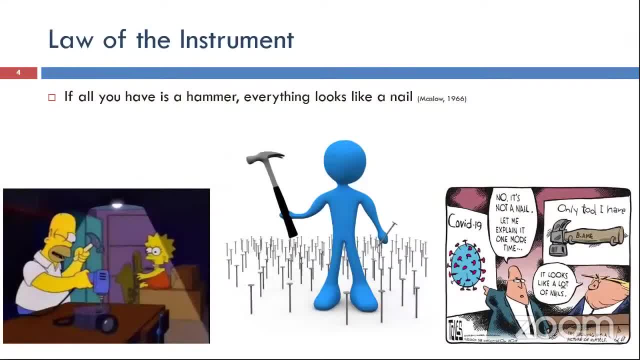 Thank you very much. There is also a very nice saying called the law of the instrument, Saad. they call it the law of the hammer. Okay, This sentence tells you a very simple thing: If all you have is a hammer, everything looks like a nail. 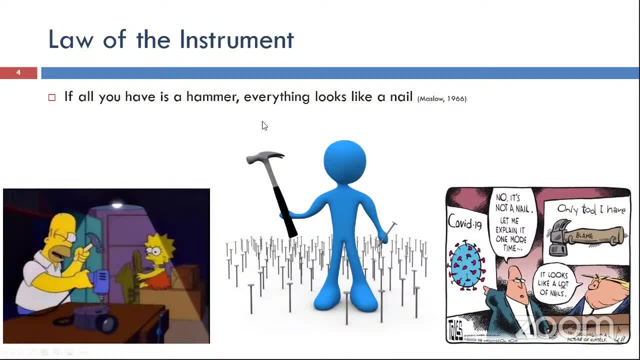 Okay, If you don't have anything else- I mean a hammer in this shape- you imagine the whole world solving with the tool you have. There is nothing else, or there is nothing else that you cannot use this tool, Okay. 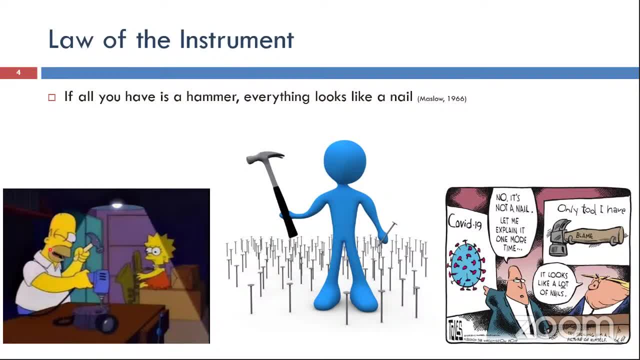 So, for example, we see, even in the in the American cartoons, for example Homer Simpson, for example, he fixes the camera, So he uses the hammer to basically open the camera, to fix it basically. Of course, the next thing you see is that the camera is made of pieces. 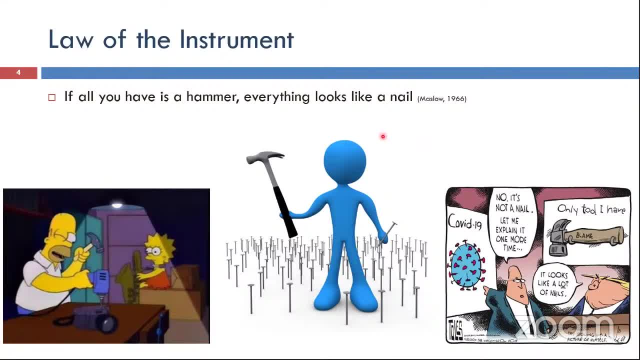 But with respect to COVID-19, I mean one of the things that has to do with the same concept. this is a scientist who explains to Trump. he explains to him about COVID-19.. So Trump says it looks like a lot of nails. 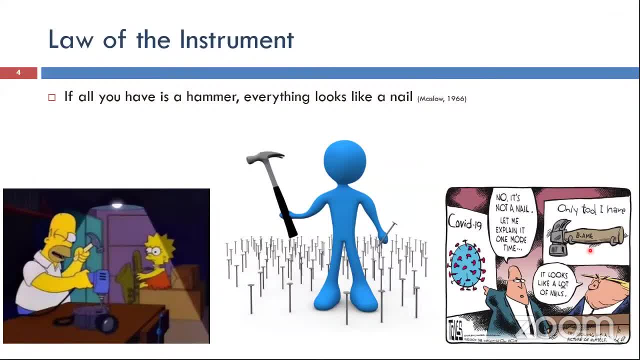 Okay, Because basically he has, he has one tool which is basically the hammer. Okay, So, basically, when you look at COVID-19, he sees nails basically. So he tries to understand: no, it's not a nail. 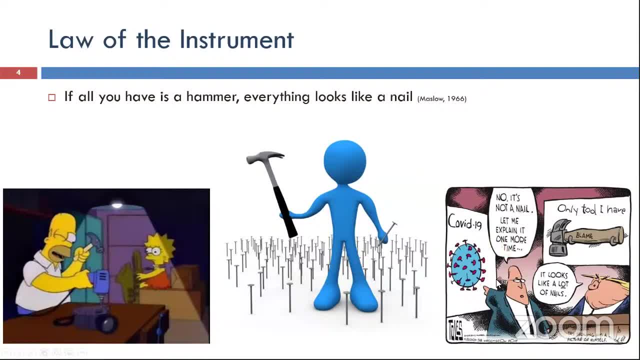 Let me explain it more one more time. Okay, So sometimes you will find that, unfortunately, when you find, for example, that someone heard about AI, for example, you will find that everything he thinks about is how we use AI. 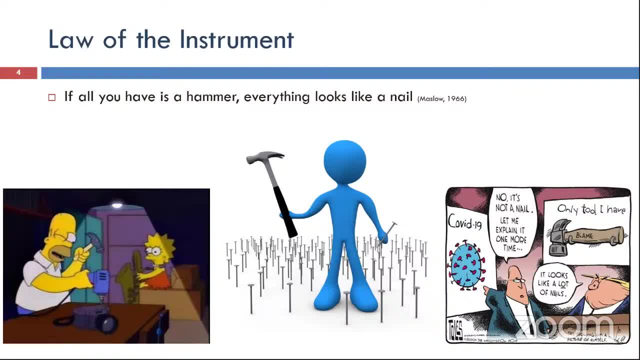 Okay, We use it in A. this is the point. I mean, he has decided that the tool is AI. Okay, Okay, So what is the problem? Okay, Although we, as engineers and as people who work in research, 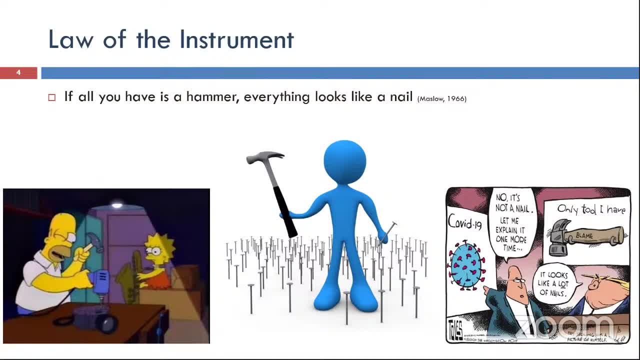 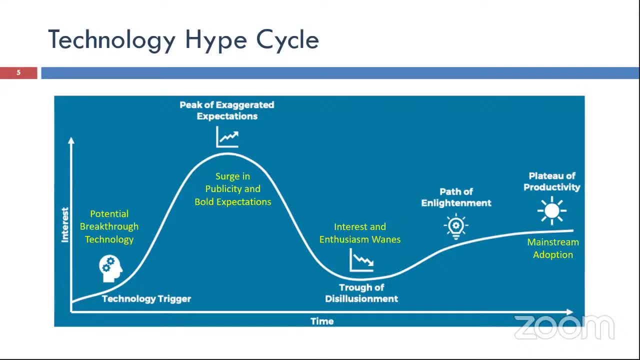 we should be centered around the problem, not around the tool. Another one of the nice things that you like to hear about before we start talking about AI is something called technology hype cycle. Hype means exaggeration in expectations. Okay, You will find that technology begins. 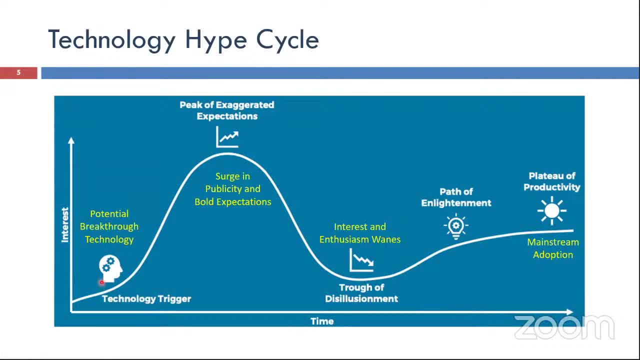 not only technology, but AI. we talk about how it begins, potentially the breakthrough of technology. Someone will suggest something that looks like it offers solutions to a lot of problems. This is what we call the technology trigger. After that, there will be hyping for this technology. 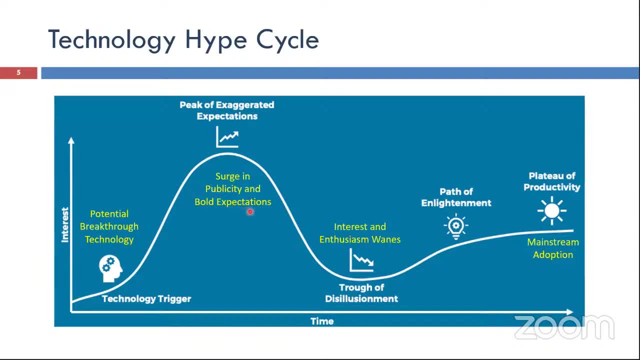 There will be a surge in publicity, There will be bold expectations, expectations that this will do everything. Technology will do everything. It will fix the environment and it will do the, the and people will not need to think, and everything Okay. 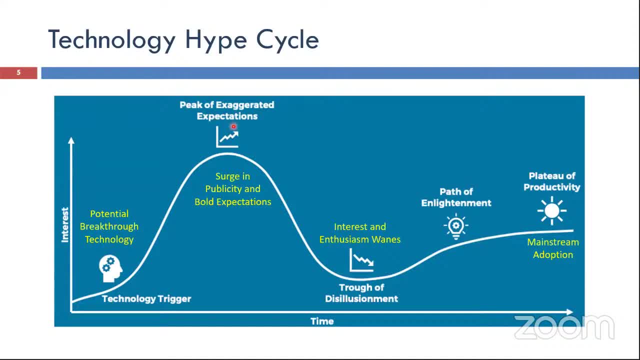 So this is what we call the peak of exaggerated expectations. After that, people, and little by little, you will start to notice that technology has not achieved what it is supposed to achieve. You will start to realize the actual limitations of technology. 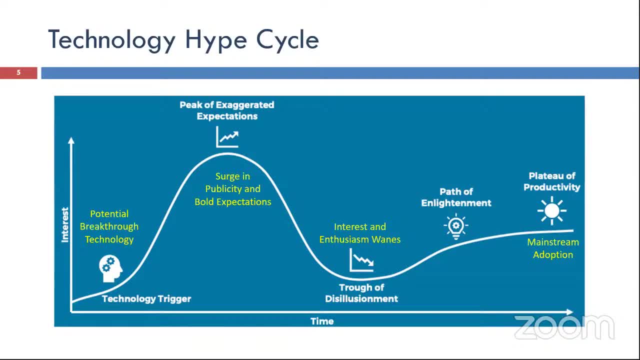 At first, people see the potential, not the limitations. After a while, you will face the limitations. Unfortunately, this will lead to something called a trough of disillusionment, Which is the trough of disillusionment. Okay, People are free from the illusion that this tool does everything. 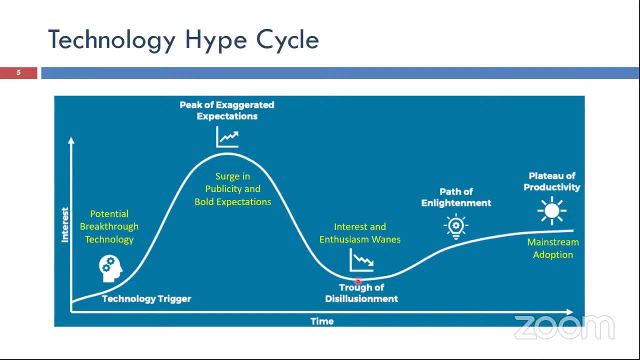 Of course this point of course can be. I mean, there are some technologies. actually, at this point it really ends. But in fact, if there is a technology that is really worth it, people will continue it. they will start to realize the limitations. 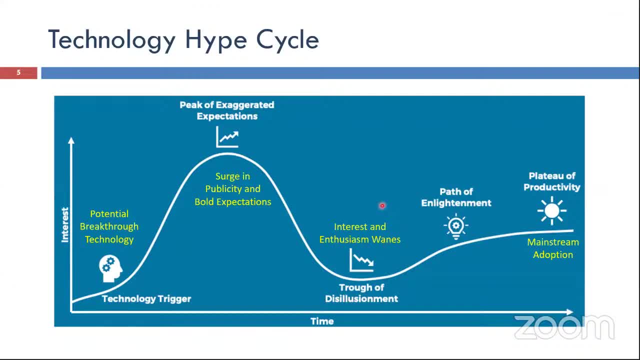 they will start to deal with it. Okay, Although there is an interest and enthusiasm in regards to this technology, it starts to decrease a lot. However, people who understand it well, they will start to take these limitations. they will start to deal with it. 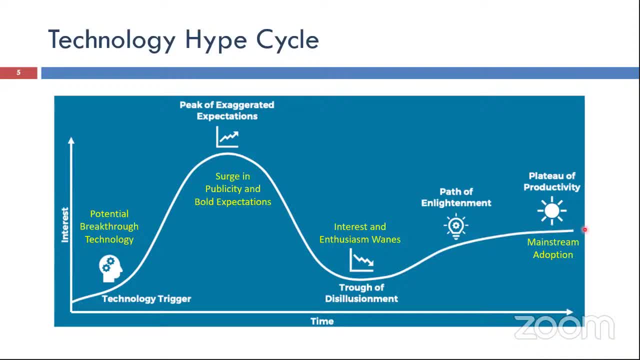 and little by little, they will find that there is an interest until, in the end, we reach a steady state value. we call it the plateau of productivity. This is what we are talking about, which is the mainstream adoption. I mean there are products in the world. 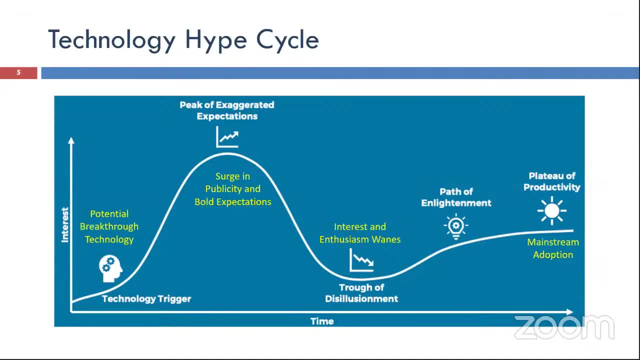 useful that use this technology, but it has not reached the exaggerated expectations and, at the same time, it has not reached a point where people are convinced that this tool does not do anything, and basically, this is the point where the technology is stabilized. 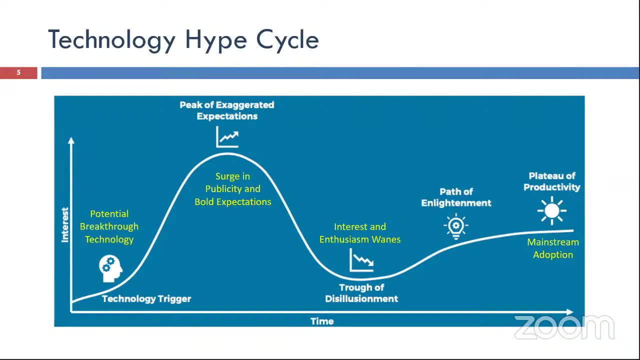 So it is very important that when we talk about any technology- any technology, I am not just talking about AI- we know where we are from this cycle. When you hear about something, a lot in the mainstream media, you hear about it in the news. 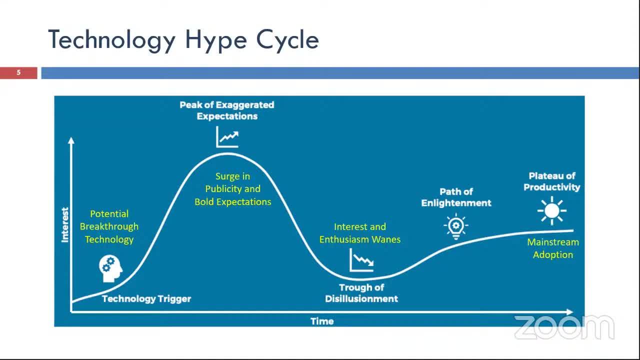 you hear about it in the newspapers, in the things that are not technical, you will know that you are most likely here in this part, Okay, Okay, Where are we in terms of AI? We will see this in a little detail. 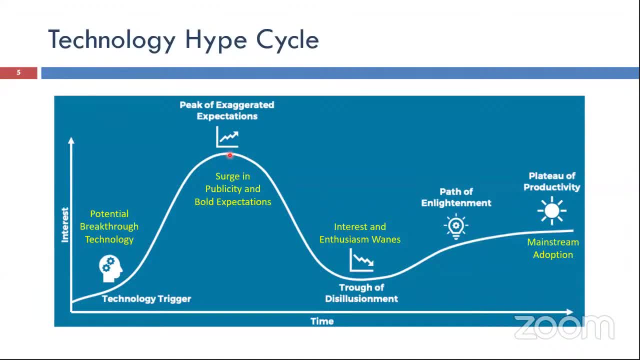 but if you ask me where we are in terms of AI, you will see this point here. I am in a place where there is a second role above me. I can tell you that we are above in the second role in terms of AI. 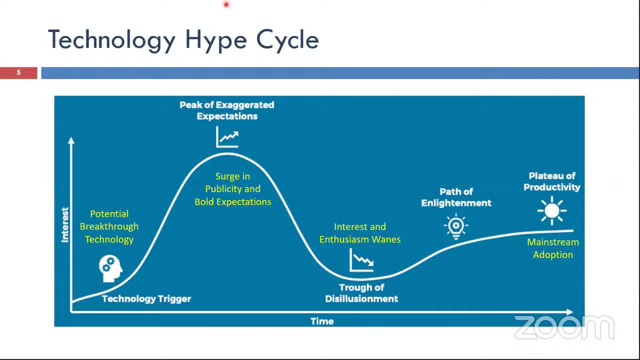 We talk about AI that it does everything. AI does not know. it cannot do everything. As we will see, there are many limitations. We have to deal with the limitations of AI so that we can actually reach the end that we will have production. 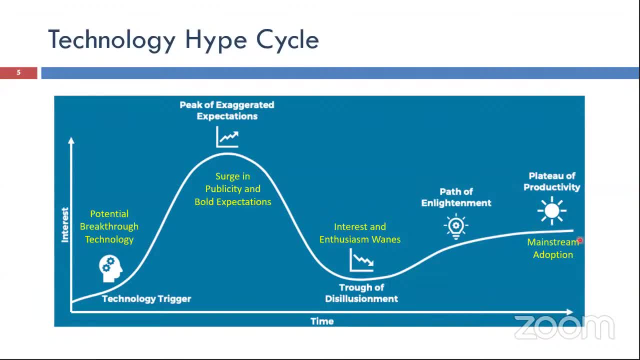 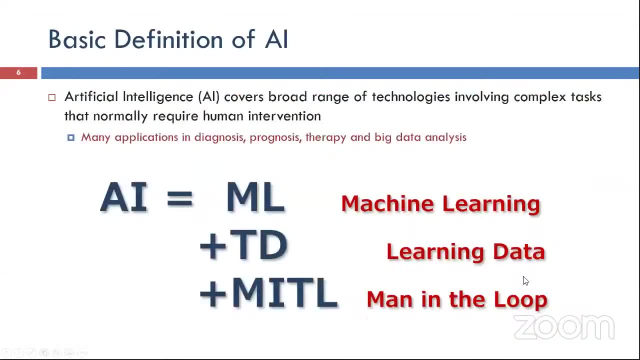 production of things that can be useful and we can reach the technology that is the main stream adoption. Let's start talking about AI. Basically, artificial intelligence is a broad range of technologies involving complex tasks that normally would require human intervention. Of course, we are talking about many things. 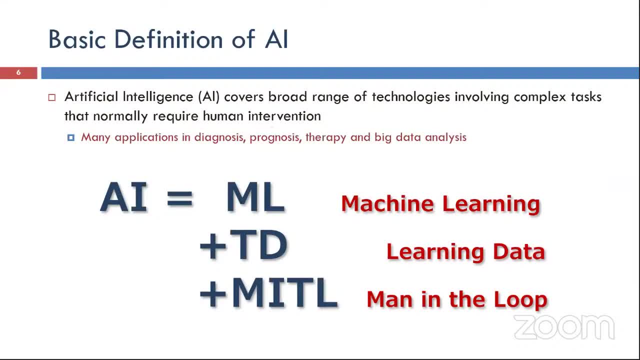 This is, of course, a little bit of an empty definition. Let's take an equation. There is a very small equation that we have found and it is indeed very logical: AI is a machine learning plus training, data plus man in the loop. What is machine learning? 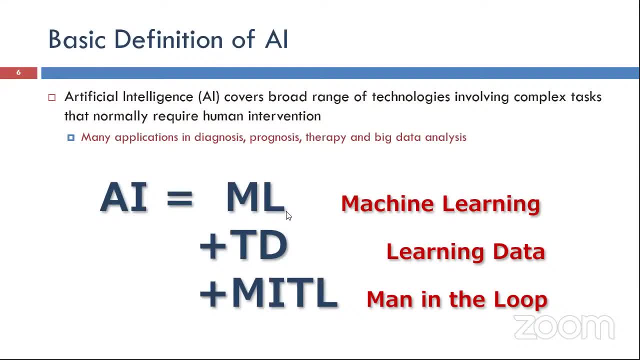 It is the techniques that allow you to learn the machine. At the end of the day, artificial intelligence will not be on a living person, it will be on a computer. You must have machine learning methods that allow you to learn this machine in a certain way. 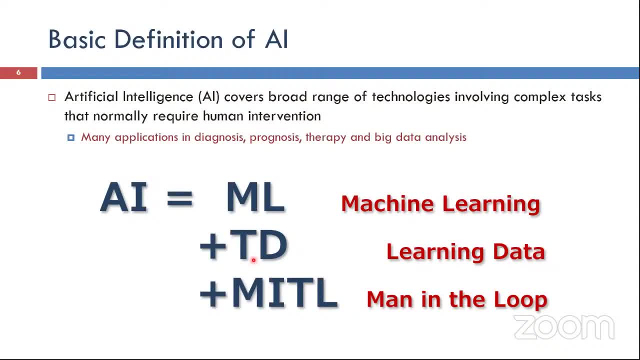 Training data or learning data- basically, as we will see in a second, is the most important thing in life, And we will find that there are some of the biggest names in AI. They tell you that your AI system is as good as your data. 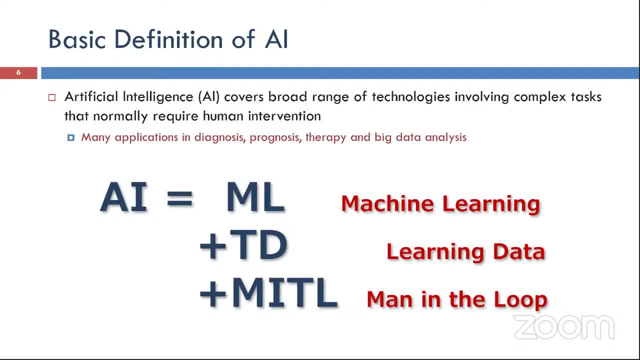 Although you may have the best machine learning technique and then you may have the best computing platform, but really, because the data you have is short, you will find that you have a problem because your system does not perform well. Man in the loop must be the person who takes care of things like this. 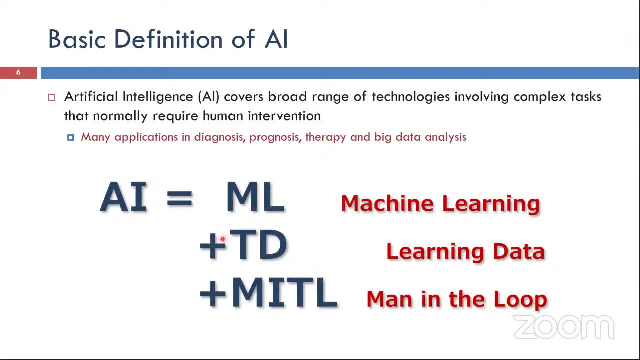 The data will not come alone. It must be prepared in a certain way and it must be filtered in a certain way so that it does not enter wrong data. as we will see in a moment, The machine learning techniques must be done by a human. 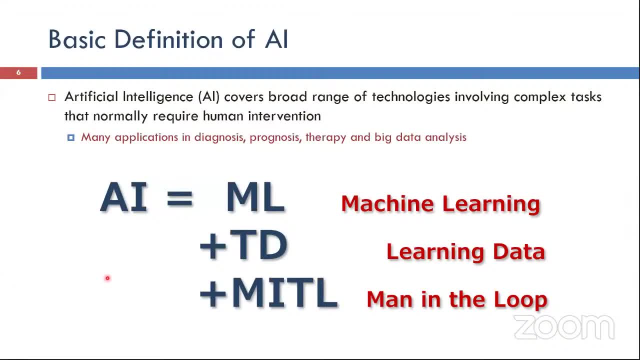 Basically a human. without the presence of a human, the machine will not be able to learn. If you you heard about the people who talk about the machines that taught life, people did not think about it. The way of learning the machine in this way is a trial and error. 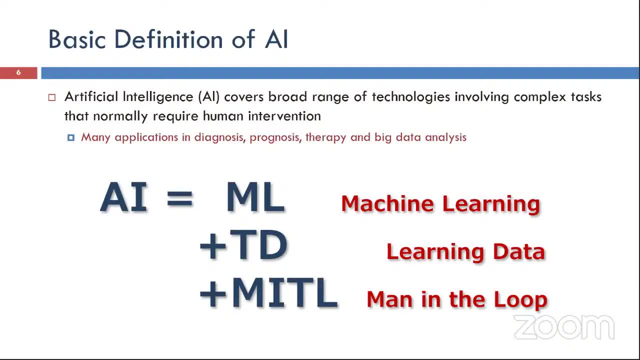 Basically, you have anything in the world. I mean, it is a set of possibilities You have, for example, if you want to move, you want to use, for example, a drug you want to use, as we will see. 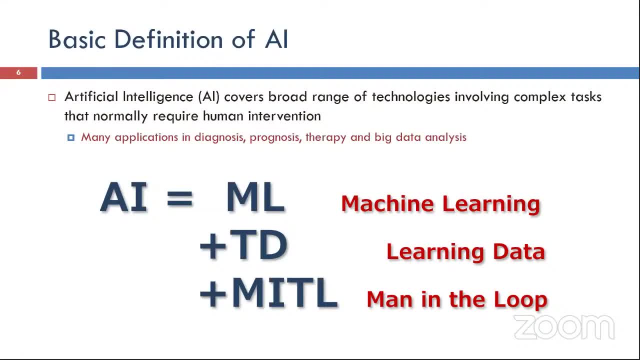 we also want to use, for example, a vaccine, a COVID-19 vaccine. okay, You have a set of components, you have a set of chemical components. Basically, anything you do, any vaccine you do, is a combination of these things. 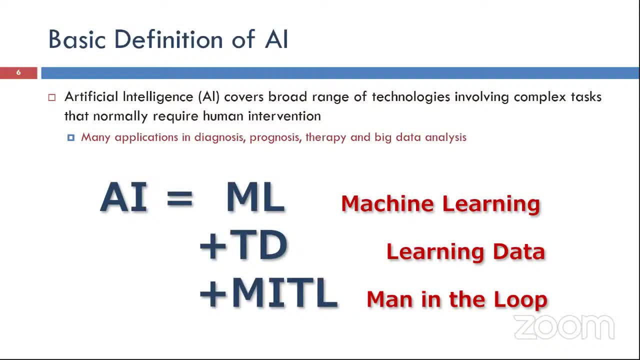 Organic material makes a certain combination for it. If you give someone a chance to try all the combinations of these things, he will eventually get to make the vaccine. So we will find the intelligence, which is the perceived intelligence of the machine. it is usually coming that the machine is trying a lot of things. 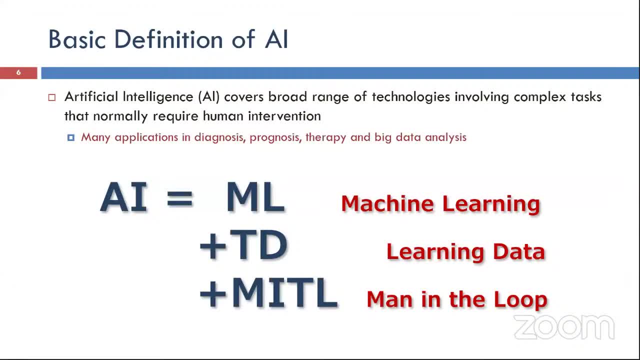 it has the ability to try a lot of things and eventually it will come out of the experiments that there is something that is working Okay. So then we are talking about something that depends on trial and error, not depends on actual higher order thinking. 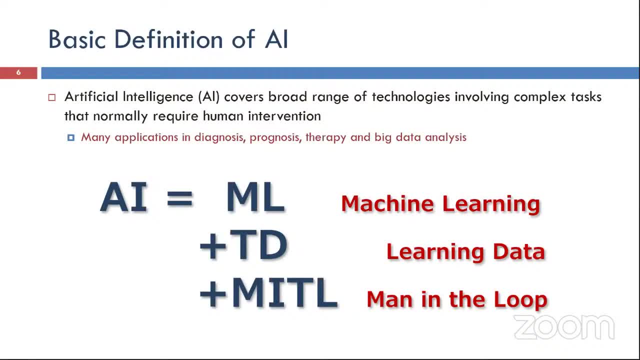 like is happening in the human brain. Okay, So this is very important: that we know that artificial intelligence must be able to do these three things. If any component isn't early, then you will have a problem. If we started with the data, 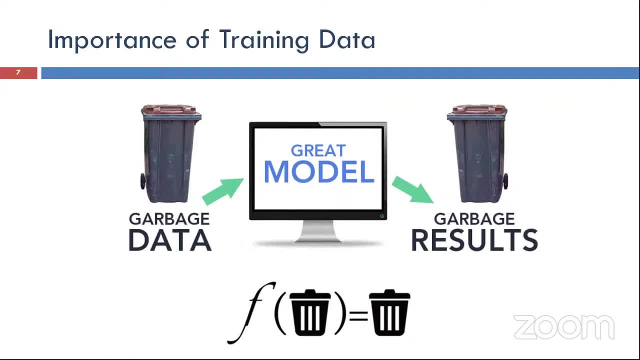 I don't want to tell you how important the data is. I mean, basically, there is one of the common sayings means garbage in, garbage out. okay, I mean, of course, it's not about the stack, it's about the last in, first out. 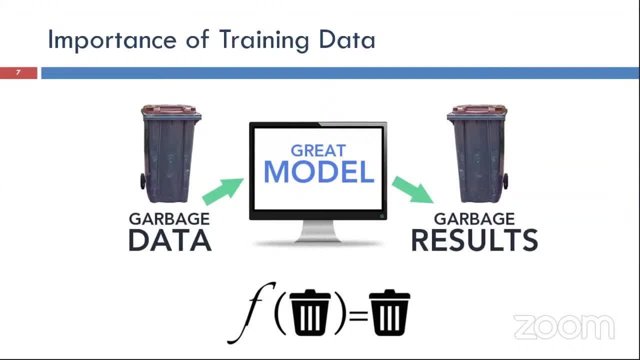 No, here it's garbage in, garbage out. If you have the best artificial intelligence machine in the world, I mean the perfect one, I mean you saw the best hardware, you saw the best software, the best learning algorithm, everything is perfect. 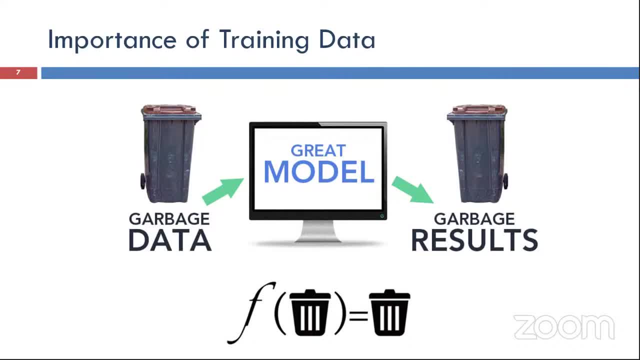 If you entered data that is not appropriate, you entered data wrong, you will get wrong results. So basically, any algorithm in general is: in the end you put it as a functional form in this way- Function basically, F of garbage is garbage. 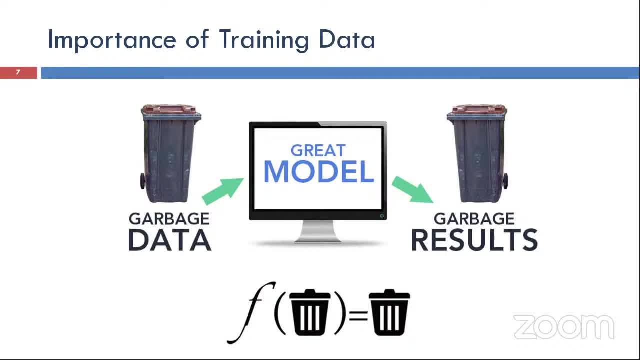 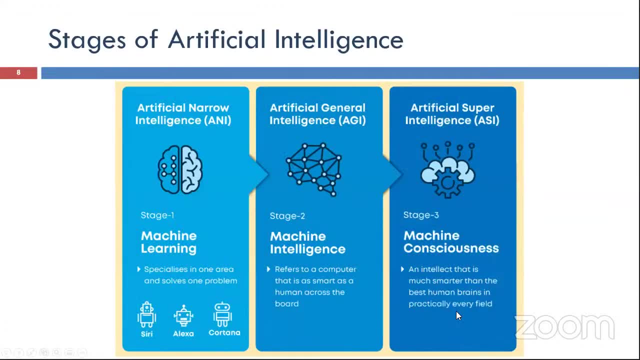 So this is extremely important. If you don't have data, or you don't have good data, you will always have a problem in artificial intelligence. So what are the stages of artificial intelligence that we are in right now? First, we have something. 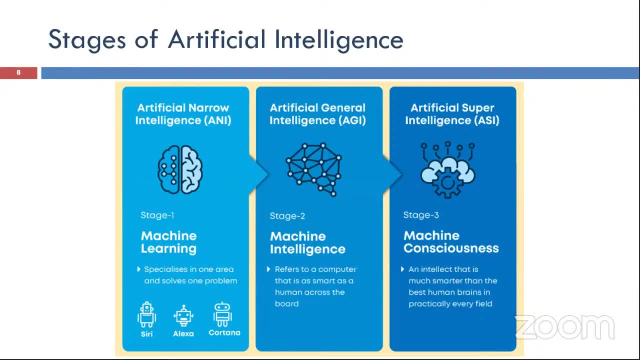 called artificial narrow intelligence. I will basically artificial intelligence in the narrow sense. Okay, This is talking about machine learning that specializes in one area and solves one problem. I mean, I'm talking, for example, if we talk about computer-aided diagnosis. 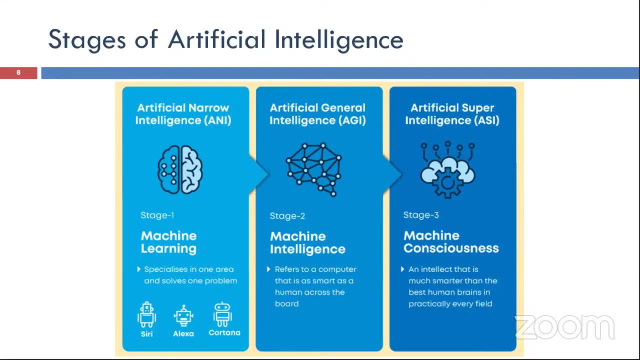 this is considered artificial intelligence in the narrow sense. Okay, Something specific, We solve a specific problem. Outside of this problem, we can't talk. Okay, I mean, it's not possible, for example, to think that the algorithm, that it knows, 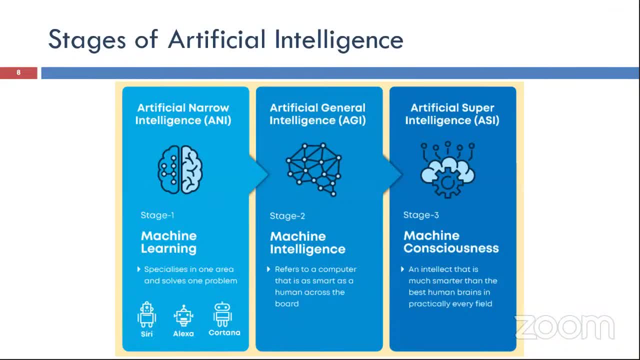 in a person, pictures, medical pictures, knows how to do, for example, a self-driving vehicle, For example. it can't do, for example, a self-driving car. It can't. They are two completely different people. So basically, 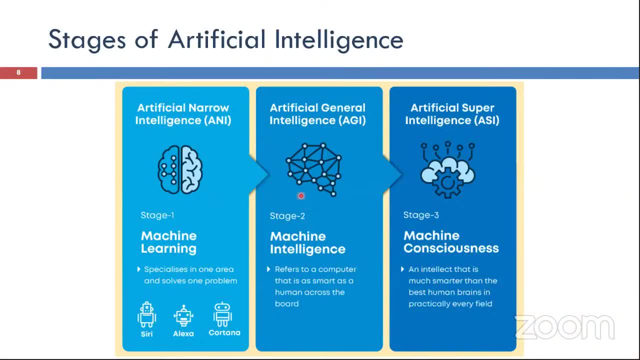 we are at the point that is here exactly. We are after that two stages. Of course the scientists' ambition is very big in artificial intelligence, But the truth, the reality of the existing technology, is that we haven't reached it yet. 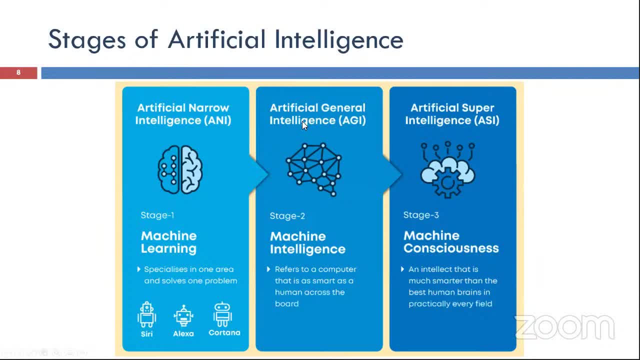 To the other two stages, The other two stages. one of them is general intelligence, The artificial intelligence, general. Okay, Which is about that? you are talking about a computer that is as smart as a human across the board. You are talking about artificial intelligence. 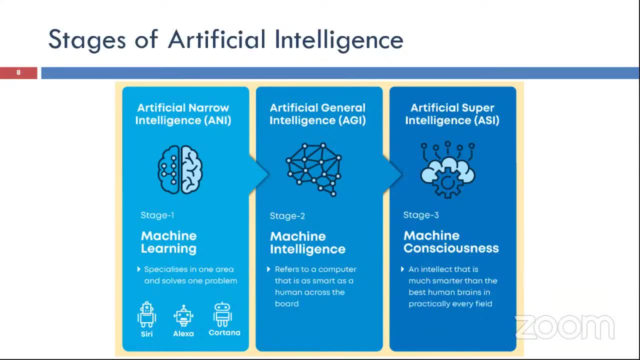 system. You can learn different things and learn them all. Okay, In fact, you won't find that there is something that you can make today? Okay, I mean, it's not possible, for example, that you are the robot that can talk to you? 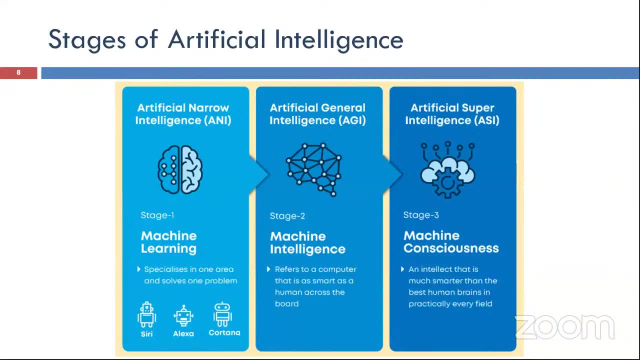 You can't tell him to teach you how to make medical pictures. It will be difficult to do that. And you can't tell him to teach you how to drive a car. It's very difficult to make him do the talking. So we are still. 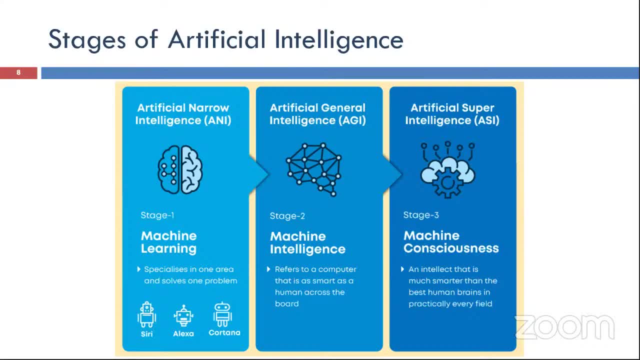 in the beginnings of artificial general intelligence. Okay, People are still thinking about some applications, But we still haven't reached to say that this stage has example products available And we can talk about it, Not even in research, The ultimate goal of all people. 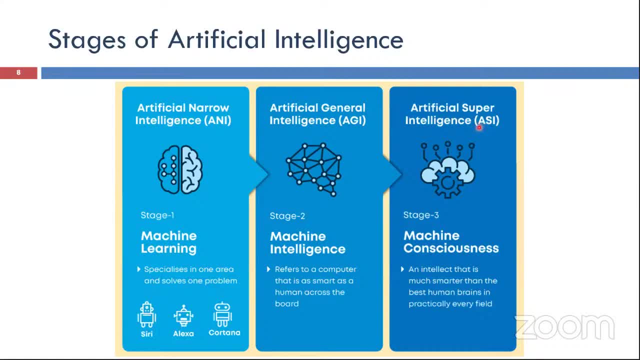 who work in artificial intelligence is artificial super intelligence. We are talking about machine consciousness. We are talking about that. the machine is aware of itself. Of course, the thing that distinguishes the human being is that he has a sense of himself When he is. 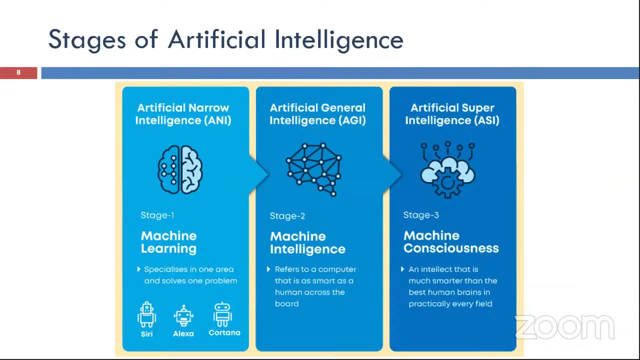 acting in a certain way. he feels that he is doing something wrong and doing something right. He feels that he is doing something wrong because he doesn't want to do it. He doesn't want people to take an idea that he is doing something wrong. 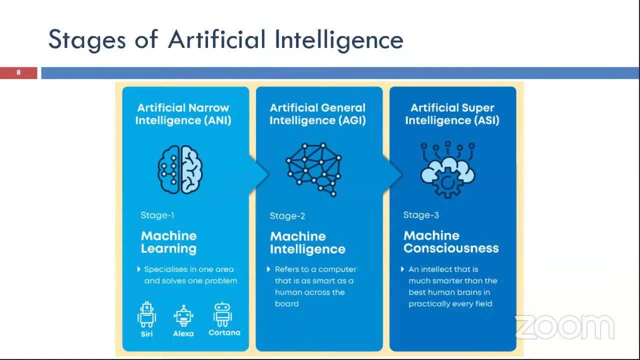 We are talking about the level of consciousness. People are imagining that in the end, eventually, the machine will have the consciousness. Okay, This is the truth. If we think about it. it is extremely difficult for a very simple reason: People 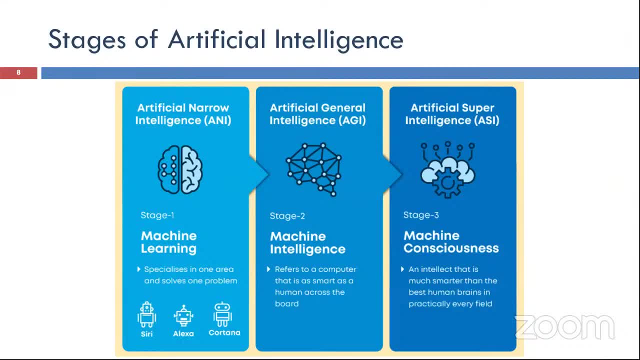 until now cannot understand the mechanism of consciousness in the human being. I mean, the research that is running in the field of the brain has not reached the higher order processing. There is still a complexity that people have not understood. The consciousness is higher than that. 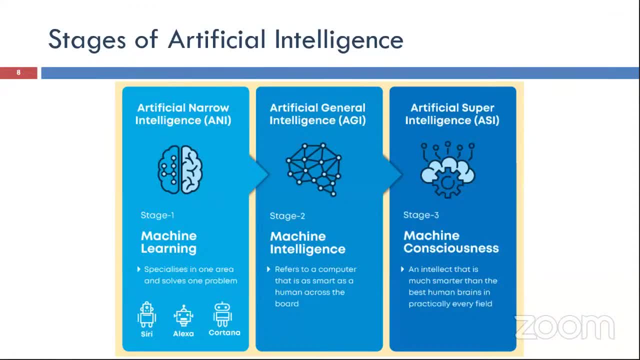 People have not understood how a person thinks and feels, because they don't feel the sensory feeling, I mean the feeling of consciousness and the conscience and the very complex things. It is extremely difficult for someone to be able to explain what is happening in the human brain. 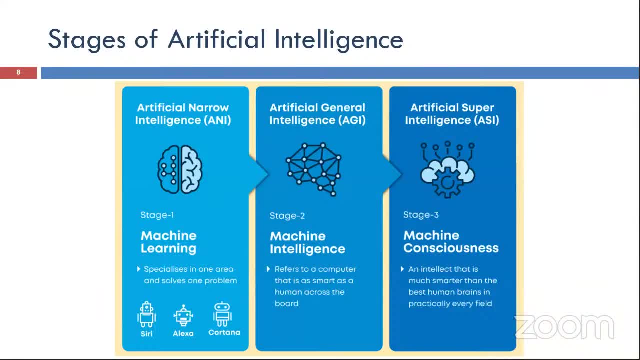 Therefore, you will always see that everything we do on earth, the artificial intelligence, is inspired by something that comes from biology. It comes from the human or from biology in general. So, without having an example in biology in order to follow it, 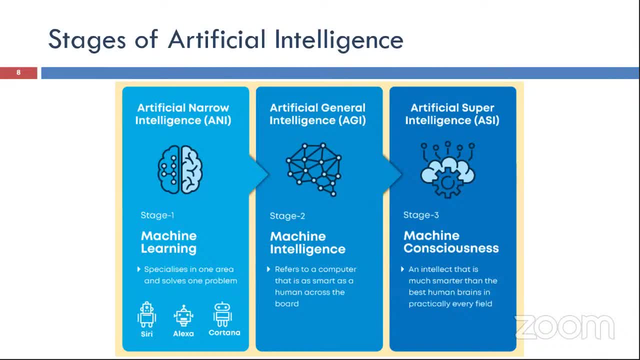 we cannot reach the machine that is made like the human. So we are talking about stage 3 that is not even in the horizon. I mean, we are not talking about it. starting with research? No, we are talking about it. that no one. 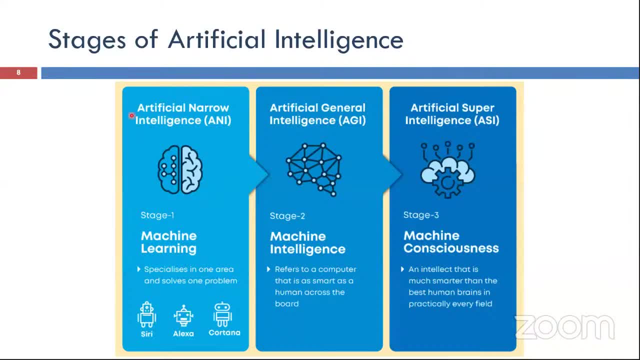 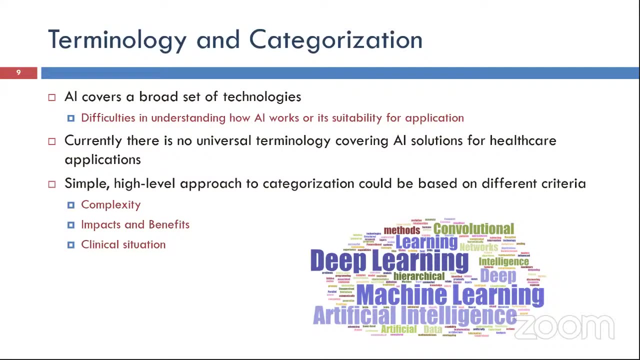 even knows how to start with it. Of course, we are talking about the narrow sense. We are talking about the artificial intelligence system that works in one particular application, that solves one problem. There is a big problem in artificial intelligence, and maybe those of you 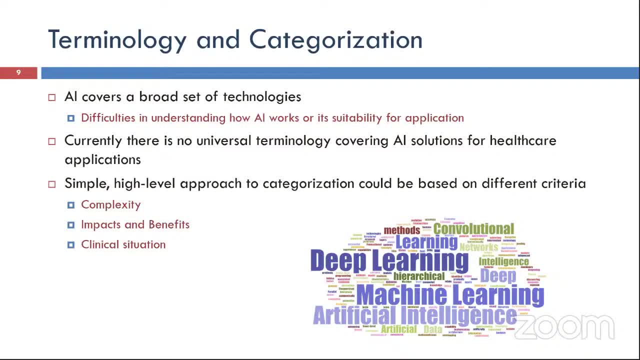 who read a little bit will find that people are talking about many names. I mean, we are talking about terminology and categorization with technology that is related to artificial intelligence. You will find people talking about deep learning, convolutional networks, machine learning. 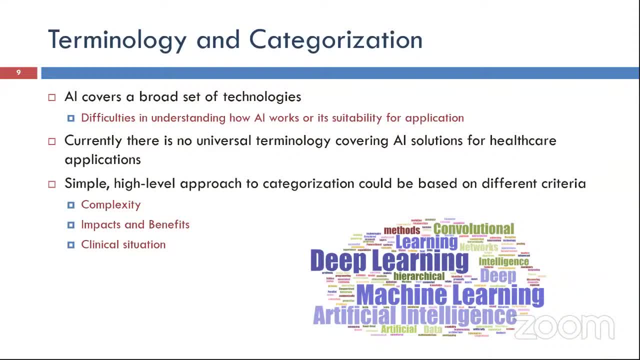 and machine intelligence. There are many names and no one will know what any of them means, So we are not talking about universal terminology that covers the AI solution until now, especially in healthcare technology. This is the real problem, because you can talk to someone. 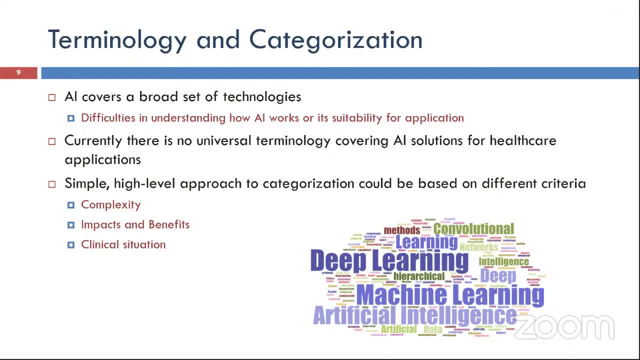 who is not familiar with it. You are talking about something and using the same terminology. Or maybe someone is talking about a different terminology than what you are doing and you think that he is doing something different. He is doing exactly the same thing that you are. 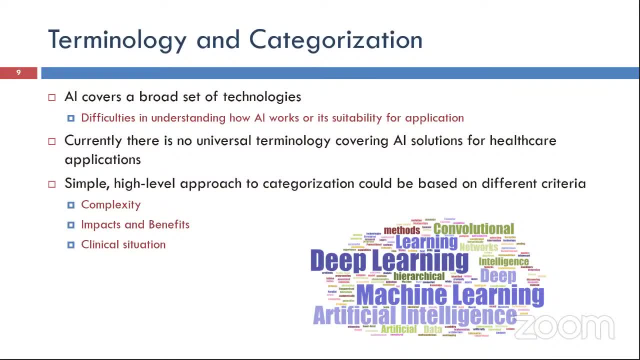 doing So, people should think about how to standardize the terminology in AI, but it still depends on the context. So you can talk about categorization in terms of complexity, impact and benefits, and clinical situation. We can take any AI system. 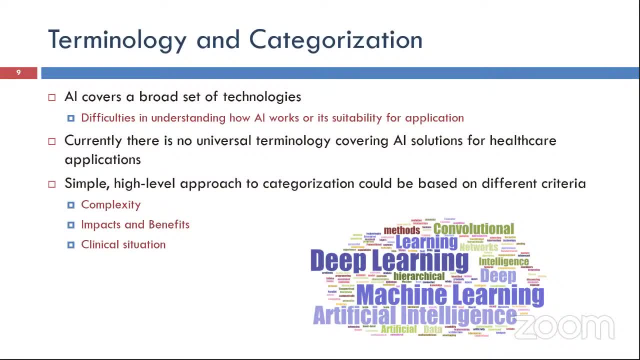 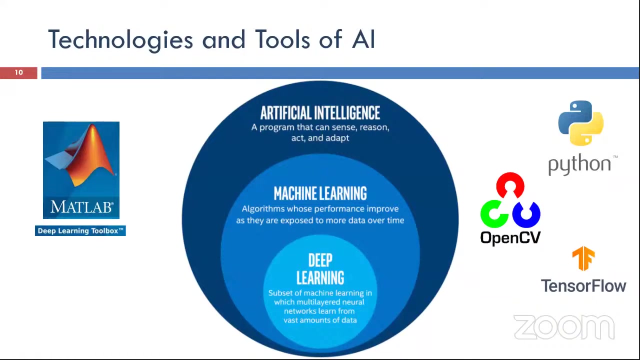 and based on these three things, we can customize it to be different from other technologies. We can distinguish the difference between the two. So if you have any questions, you can ask them in the slide. Just remember the number of the slide so we 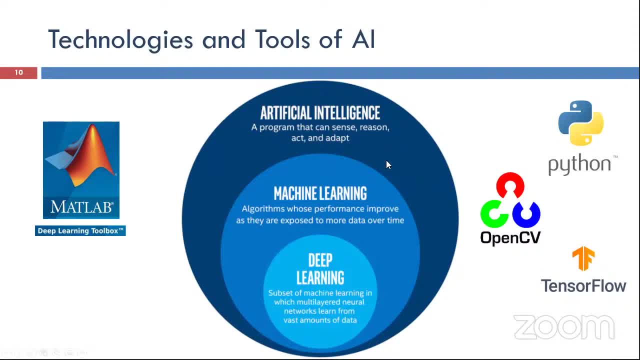 can get back to the questions. What is practically available? First, artificial intelligence contains many things. The most important thing is to know which technologies are used and whose performance improves as they are exposed to more data over time. Okay, Subclass of machine. 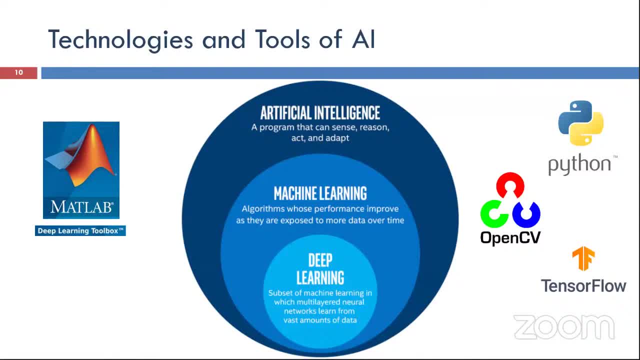 learning is deep learning. Deep learning is what makes AI spread beyond the imagination. Deep learning is a subclass of machine learning, and this is a subclass of artificial intelligence, meaning that deep learning relies on neural networks. The other important thing is that it. 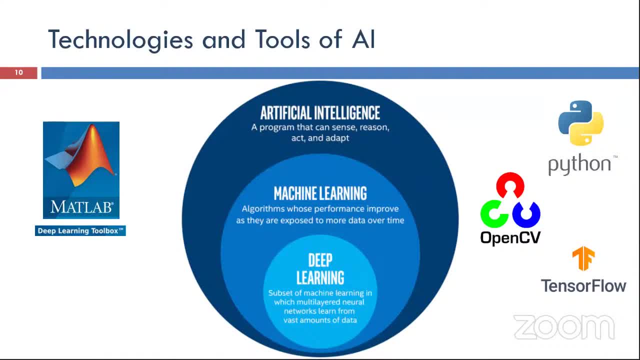 relies on vast amounts of data. Basically, it relies on machine learning, because the more data you give, the better performance you get. It relies on artificial intelligence, which is basically programs that allow you to do things that are smart and adaptable. It is 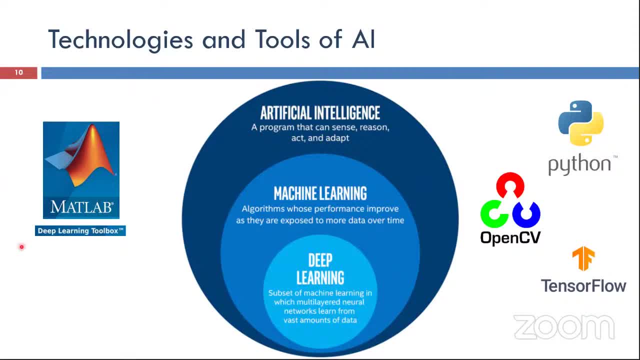 based on the data of your client. This is the best tool to do. AI is MATLAB. I will show you a demo of it when the presentation is finished. If you want to use the open source tools modules that they're able to download- all of them are for free, basically, and they're able to develop. 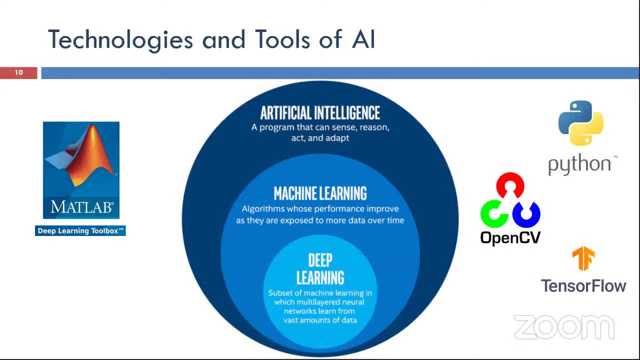 the techniques themselves. So, basically, if we're talking about deep learning, basically their main idea is brain tests. Okay, The people, as I'm telling you, don't understand how the brain works, So they try as much as they can to understand it. What exactly does it do? 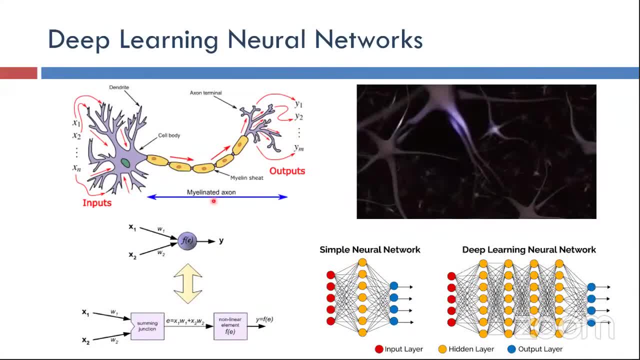 It starts with the neuron. We started this in the 80s and 90s. It started thinking about neurons. Neurons, as we took in physiology, are cells. Of course, we're talking about myelinated cells. The cell looks like this: The difference between myelinated and unmyelinated neurons. 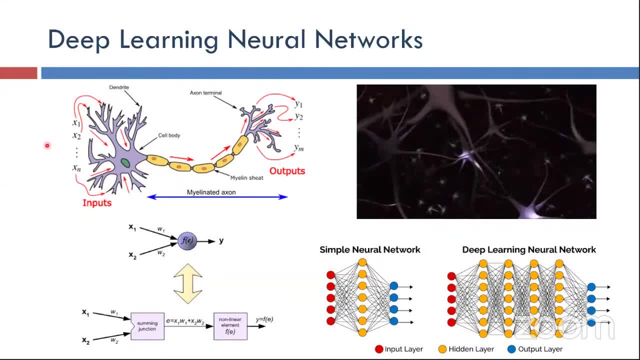 is in the speed of transmission, basically. So I have here the cell body, so I have dendrites. They're the ones that insert the input into the neuron. Processing occurs inside the cell and at the end there's an electrical pulse that moves through the axon. 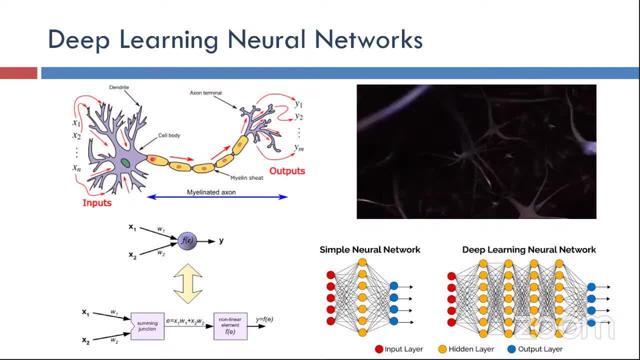 which is the tube that's in the neuron, And at the end the signal comes out through the axon terminals. This then goes to interface with another neuron through the dendrites. So the people saw this model. They said: let's put a simple model. 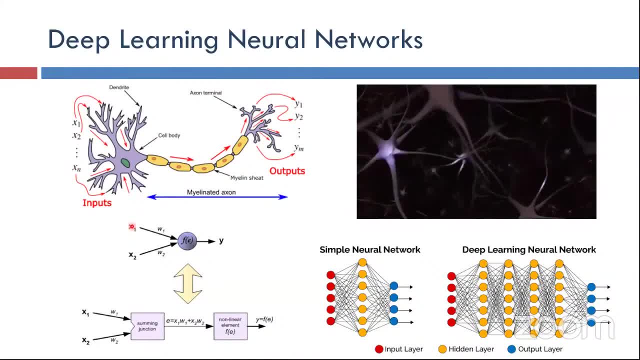 a simple mathematical model, which is a set of inputs. The inputs can change. There can be any number as I want. Each one of them has a weight Because, of course, each one of the dendrites can have a different signal path. so it does attenuation or amplification. 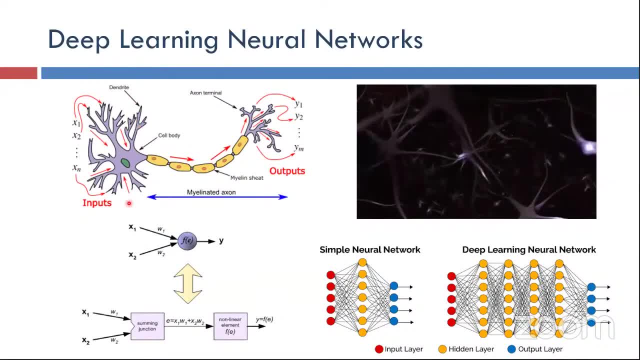 It's mostly attenuation to the signals coming through it. So each one of the input signals has a different weight. Processing happens inside the cell body and then the signal goes out through the output to the next neuron. Actually, people found that in order to do this, 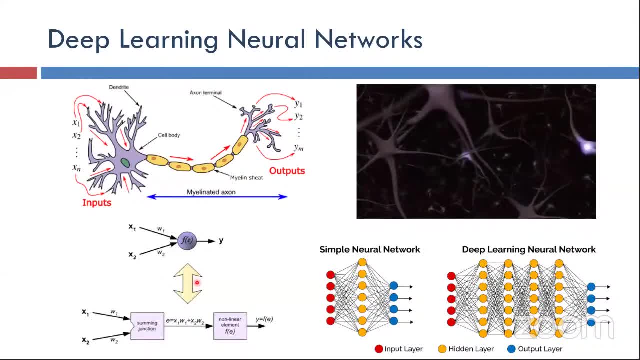 in a way that allows you to do something close to the function of neurons. Basically, you have this part here which is a summing junction, meaning the thing that came out of here is x1w1 plus x2w2.. After that, the processing that happens here must be nonlinear. 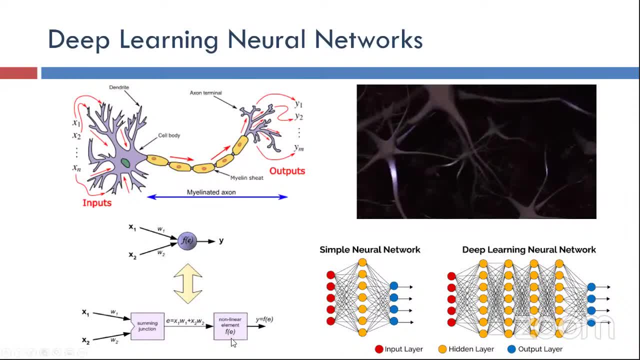 Usually people can take different forms of nonlinearity, but in general it must be a nonlinear function. This nonlinear function gives you the output at the end, which then enters the input of the neuron. again, People started to do something like this: 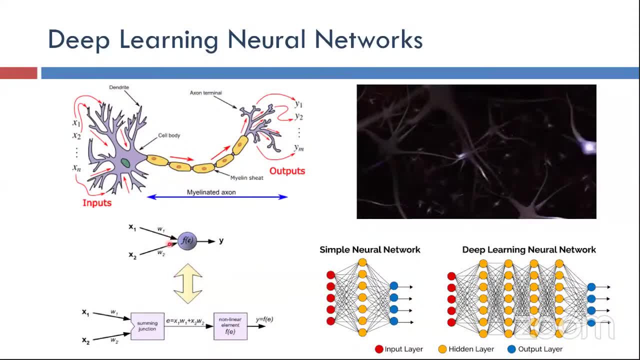 Each one of these circles is considered a model of these, which are neurons like these. We are talking here about the input layer, the output layer, and you have something here: anything in the middle between the input and output. we call it this layer. 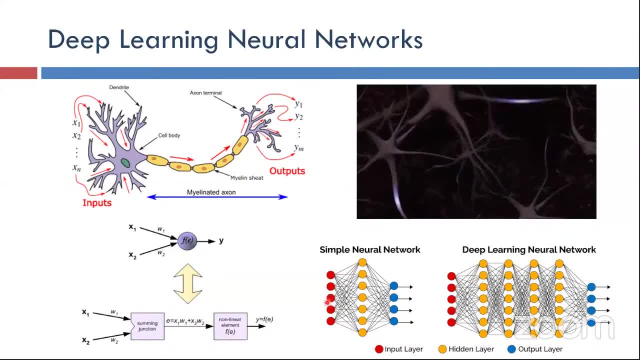 Basically, you will see: the output that came out of here enters here and enters with it from here and from here and from here, and so on. each one of these receives inputs. from all the inputs that are present, This shape is called. 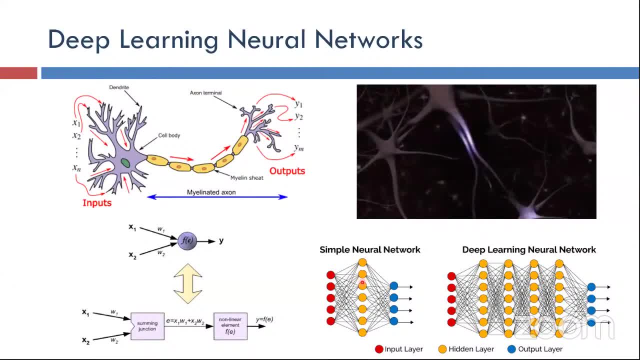 Fully Connected Layer. Fully Connected Layer means that any one of the neurons present here in this layer is connected to all the neurons present in the previous layer. This is what people did in the 90s, and saturation occurred at the end of the 90s. 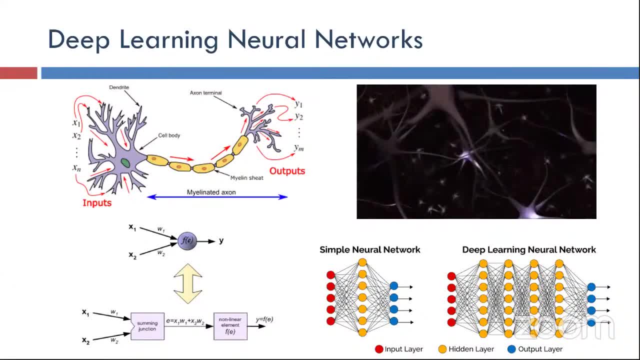 In the early 90s, the Neural Network was the hot topic that people were talking about. People thought that the Neural Network uses everything. Why in this way? Because it is something that looks like this in the simple form, And it was discovered that 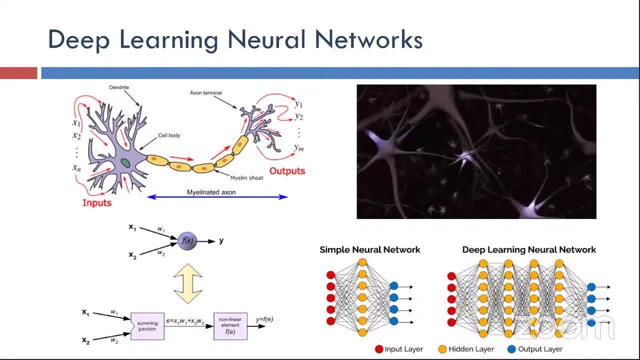 there are a lot of problems in this approach and there are problems that you don't know how to solve. So in the late 90s, a new technology started to appear that they said that the simplification of the human brain. 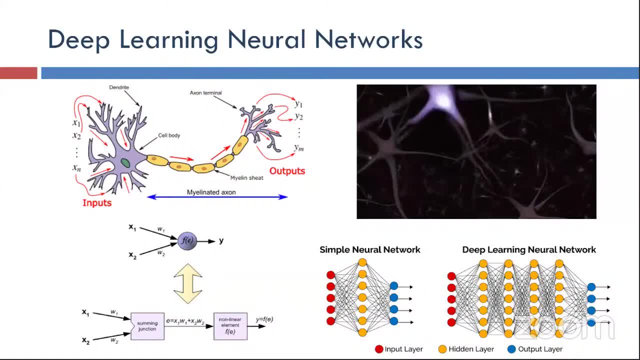 that it is about input and output layers, and one hidden layer or two hidden layers is not enough. Let's put, for example, 50 hidden layers. Okay, So we started to have a movement from the simple Neural Network, we started to have something called 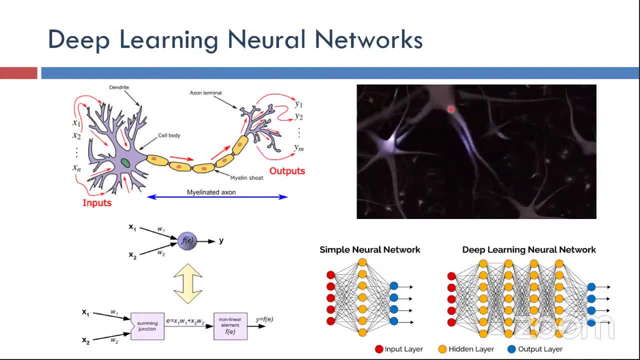 the Deep Learning Neural Network. The goal is to do something like this. We have a very complex network of connections that connects between the input and the output. When you do this, your ability to achieve any function you want or to do anything you want. 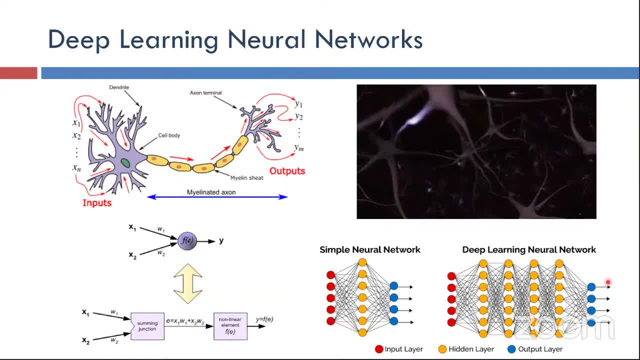 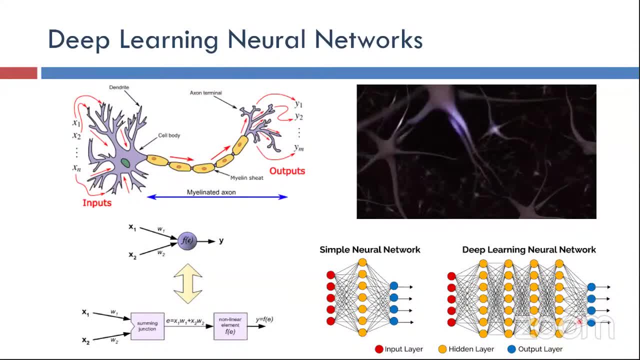 of the Hidden Layers. I can actually do this. For this reason, theories started working. we call this The Universal Approximation Theory by Neural Network. Basically, it uses a shell in this form, in a condition that, as we talked before, 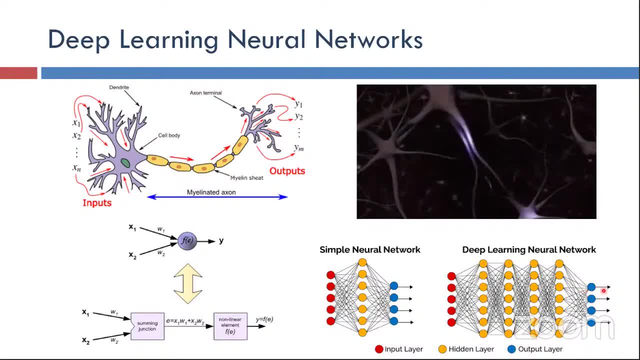 you needed to have nonlinearity. Using a shell like this, you can do any function from here in any way that you want. If you bring me any function in the world, I can make it available to you. that is, I can make it an approximation here. 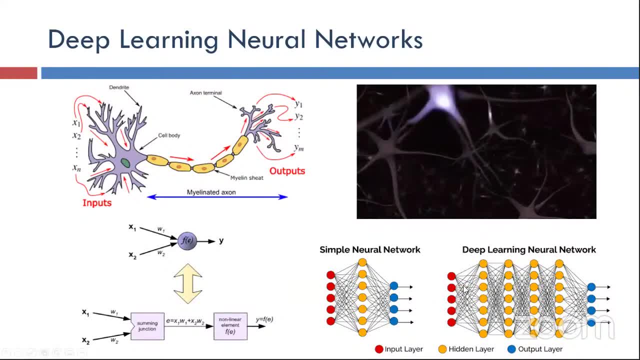 by just using Neural Network, this exactly. So therefore, there was an interest in deep neural networks and there was a boom in hardware and computers that allowed the processing of those who needed it to be able to build this network, and therefore applications began to appear and deep learning neural networks began to be very impressive. 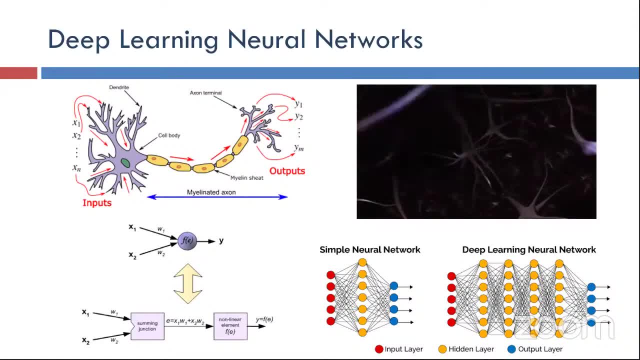 I mean before that, because people would imagine that you could do processing of images using a neural network. there were problems in the 90s that you could do something like that. When we talk about that, we arrived at the end of the 2000s, for example, and the beginning of the 2010s. we began to see that there was hardware and there were GPUs and there were things that really allowed processing to be much stronger and there began to be applications for deep learning neural networks. that became extremely impressive. 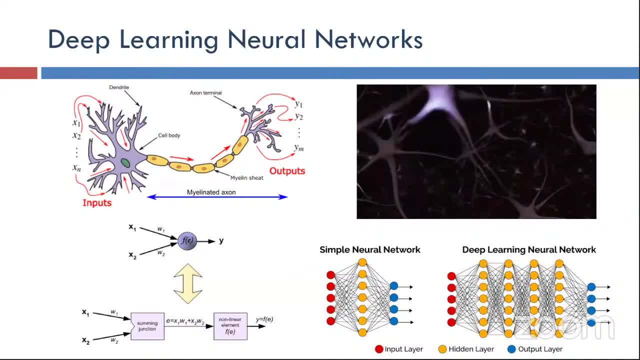 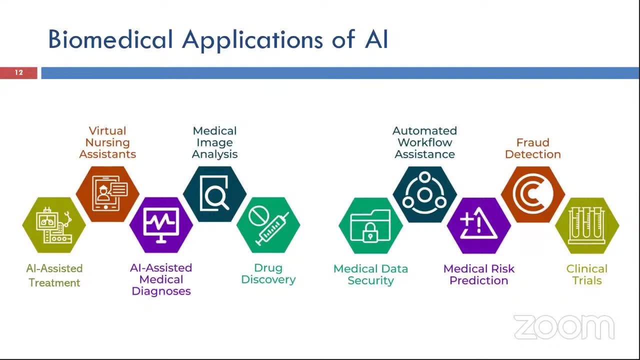 Okay, So we are talking about deep learning, neural networks. Okay, That is the core or the main technology that artificial intelligence relies on. What applications did artificial intelligence use? It has many applications. We can start at the beginning, on the left side here. 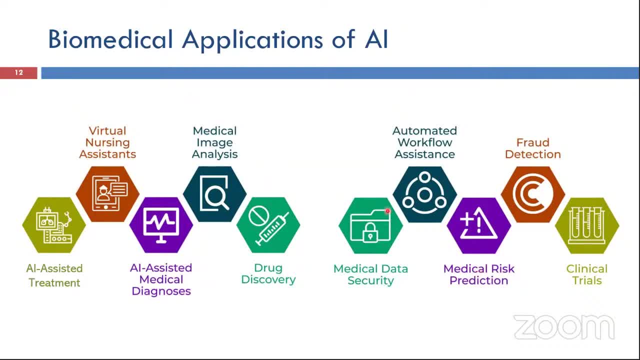 We talk about things that are not related to clinical practice. Here we talk about things that are not related to the administrative aspects of healthcare. For example, we talk about AI-assisted treatment. You can take the experience, the experience gained from the treatment of a person for 30 years. 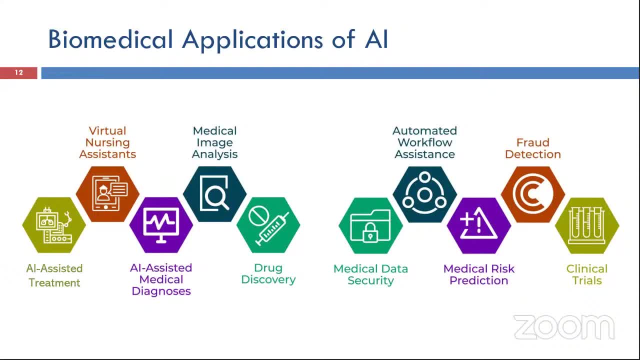 for example, and learn from it, the artificial intelligence system, and then he can make direct recommendations if the treatment is suitable for a specific case or if parameters are interfered with, for example, the analysis of image photos and so on, and then take suggested treatment. 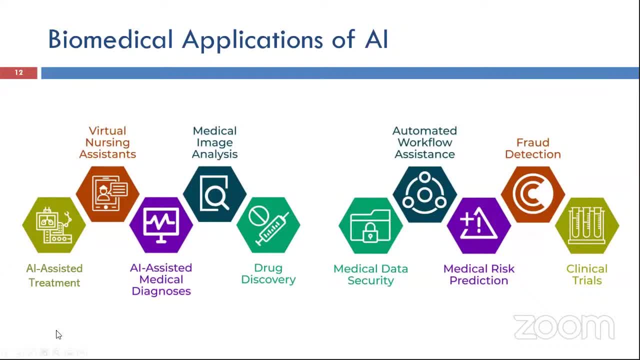 based on this AI system. We are talking about AI-assisted medical diagnosis. this is the example we will take, for example, the computer-aided diagnosis, whether it is from medical image photos from, for example, ECG, EEG. 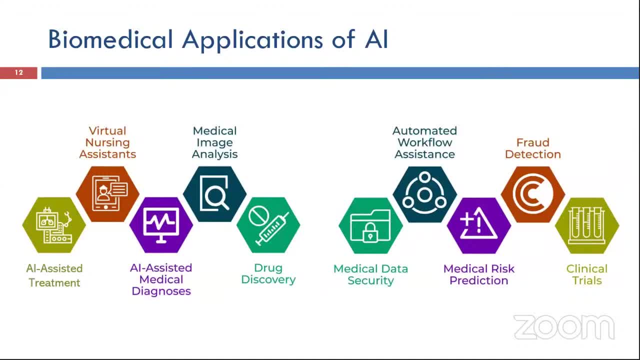 and all these things, we can really build a smart system that can help us use it in patients. Let me tell you something very important. there is the word assisted here, not AI-based, but AI-assisted. We will see later in the part related to the legal issues related to AI. 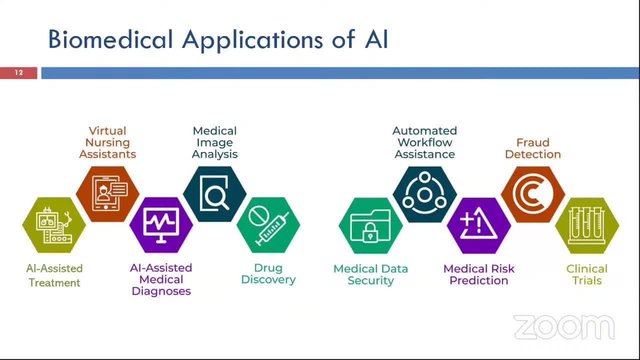 that you don't have to make a computer or smart system work on its own without accountability, because, in the end, as long as there is no problem, someone has to be accountable, and the only person who can be accountable is not the programmer who made the AI system. 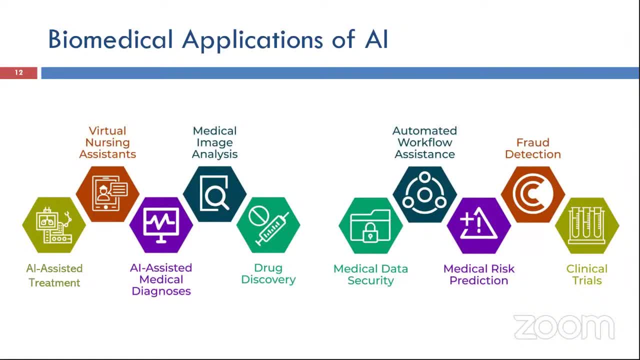 but the doctor. The doctor takes the output from the AI system, thinks about it and then decides the decision he sees for the benefit of the patient. All the technologies you find in the AI system you will find in the parts related to diagnosis and treatment, in particular. 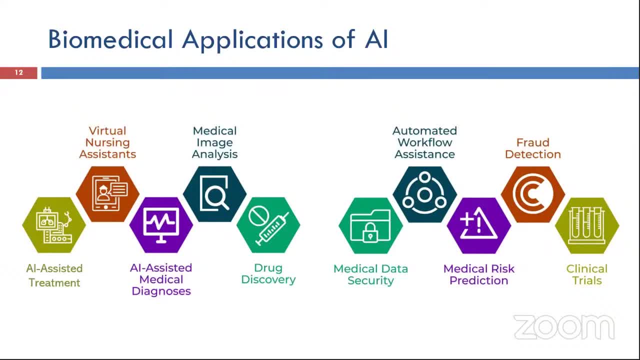 you will find that it is an assistance for the doctor, not a replacement for the doctor. We will talk about the medical image analysis, of course, one of the important applications. We will also talk about the virtual nursing assistance. we can talk about the patient staying at home. 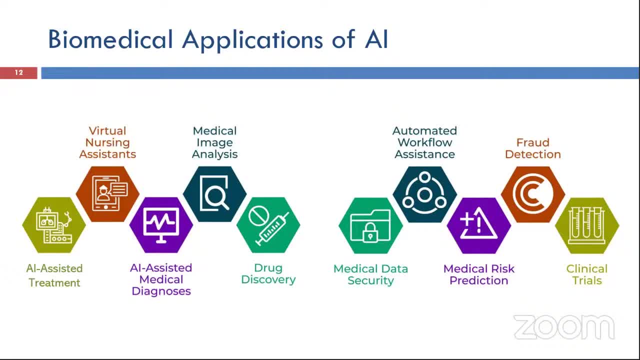 and he can communicate with the chatbots. we will talk about some smart systems that can communicate, that is, send the problem and he sends you the solution. that is, you can communicate with the actual nurse, but the actual nurse is the AI. 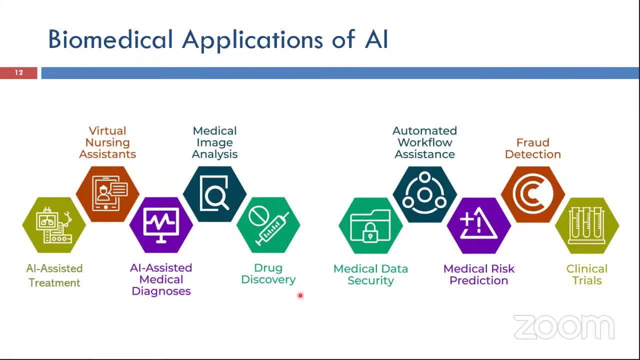 The part of drug discovery. I will explain it later because it is very important in the current circumstances, because we understand how we can do drug discovery using AI. Of course, the parts here we talk about things that we do not see. we do not see in the healthcare system. 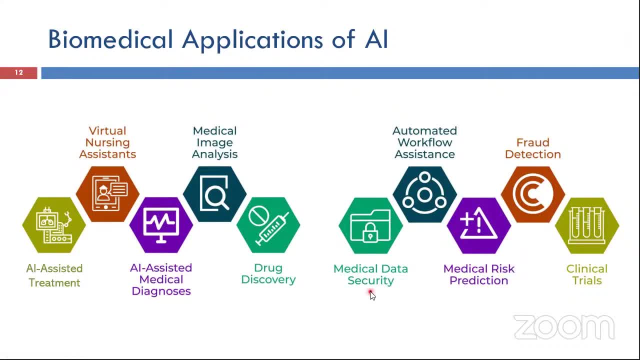 but there are very important ones, For example, medical data security. Now many hospitals are exposed to the virus, ransomware attacks or cyber attacks in general. now it is possible to stop some hospitals and there are actually incidents that happened that stopped some hospitals because there were cyber security breaches. 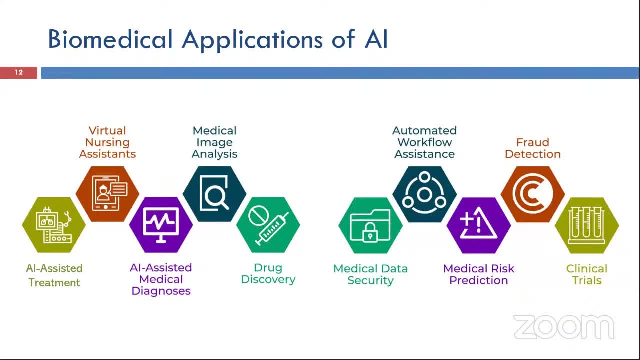 Now we have AI. that has a great role in being present in the firewalls, in the security appliances that it uses to prevent cyber attacks. It has a great role, especially in the medical field, in terms of importance and privacy. I really do not want to emphasize how important it is. 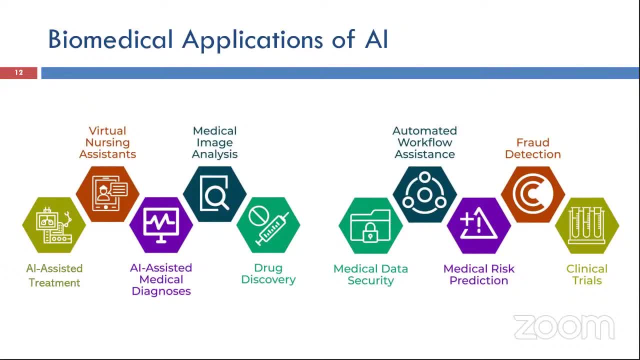 I mean the value of AI in something like this, that it follows things like this. it really has a very great potential. We are talking about automated workflow assistance, Maybe the system in the hospital. we have certain steps that we do for everything. 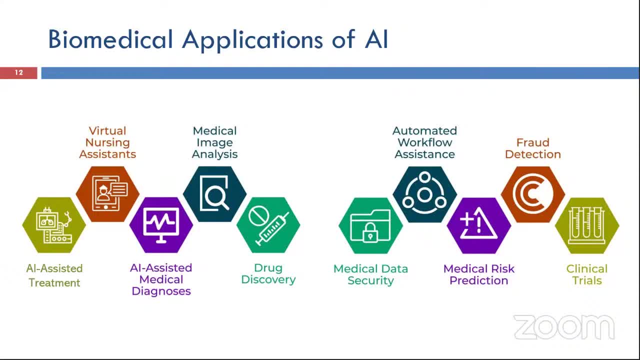 for example, the patient to enter and do certain tests. for example, there is a certain workflow. For example, at first he goes to a general doctor and then he makes a referral to the factory, he makes a referral to the doctors. 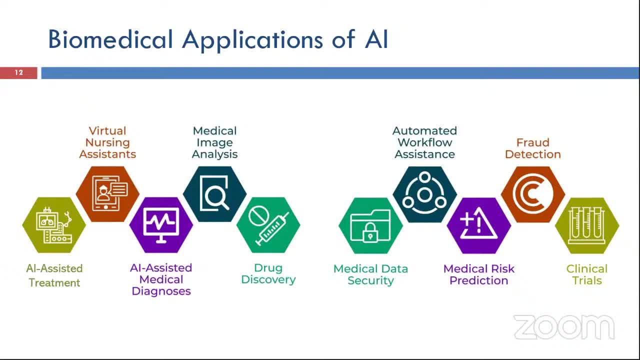 he makes a referral. according to the results, he can make him go to a surgeon or he goes, for example, according to the case. there is basically a workflow for the processes that happen in the hospital. Generally, there is a role for AI. 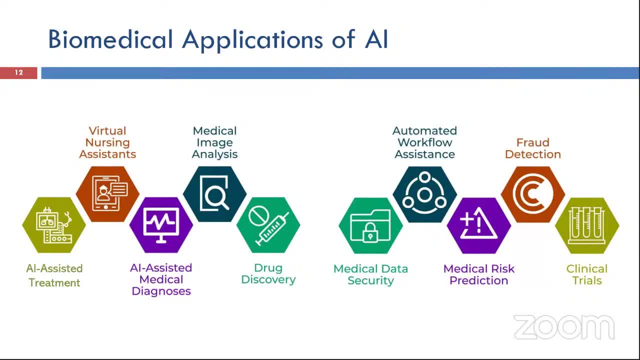 the optimization of the workflow in general in all institutions, including healthcare in all facilities. This optimizes and makes the efficiency higher in healthcare facilities. We are talking, for example, about insurance companies. we may have part of the medical risk prediction. 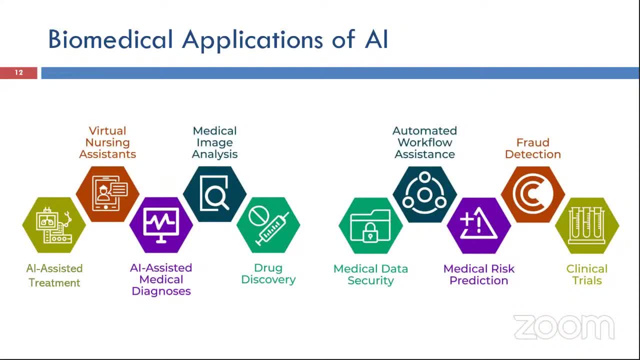 When someone applies to take insurance from a certain company, they should see their health record and, based on that, they see what their premium is and see if he is a high-risk patient and if he is a low-risk patient. How do all these things work? 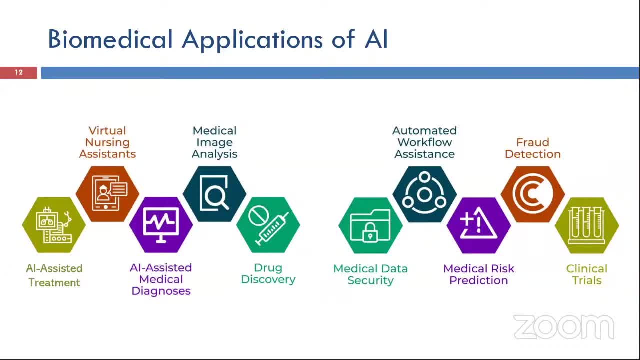 They work manually, Of course. when the data is accumulated and we have sufficient amount of data, medical risk prediction systems start to help people in insurance companies to make decisions based on much wider data, not just to examine the patient's data. They see that there are certain risk factors. 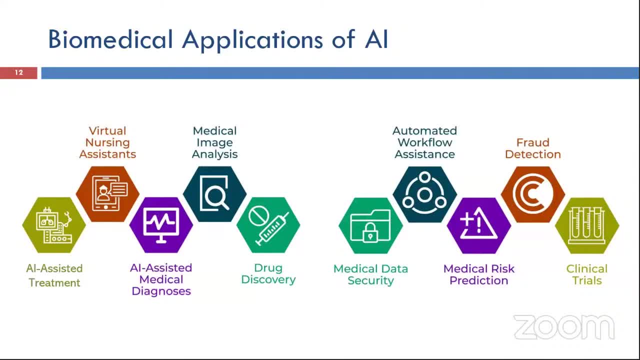 the insurance person may not be able to see them, so they can improve the operations of the patient. and the patient may not be able to see them And, of course, when it comes to health insurance, you will find that there is always fraud. 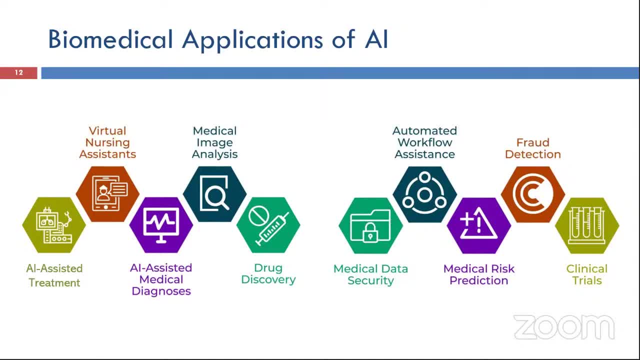 For example, a person comes to perform a personal examination of someone else, There are some things. for example, when he performs a certain examination, the system may have a part of this fraud detection based on AI and it may notice that this examination does not look like the examination that was performed before. 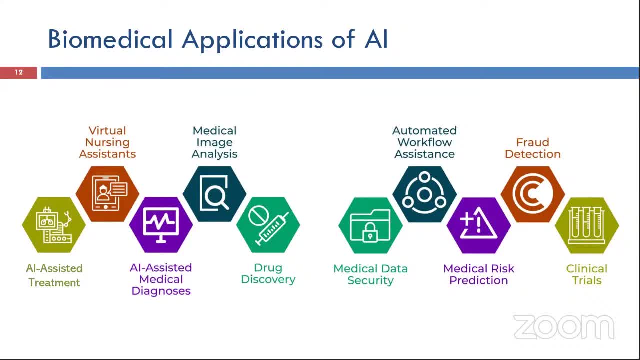 by the real person who is a personal examiner. Therefore it may detect the fraud, or if he sees that there is a different frequency for the visits of the doctor or there are medicines that are not supposed to be used in this rate, 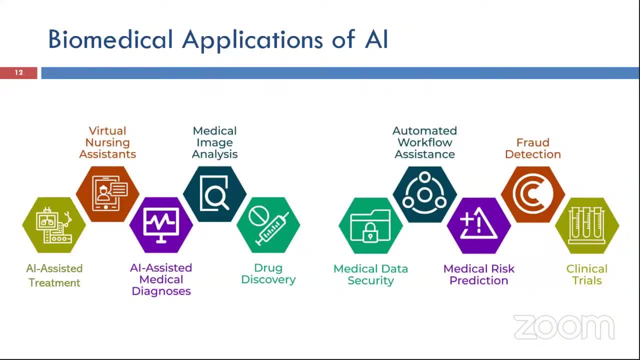 he may be able to notice all these things for all the patients in health insurance. And, of course, at the end there is the clinical trials. You can optimize the clinical trials. Maybe, instead of needing a larger number of patients, you can actually get results that prove that. for example, 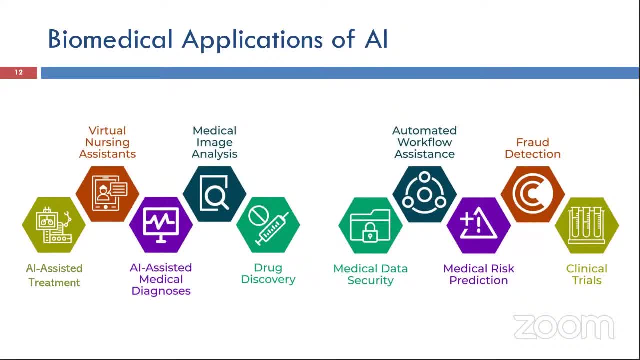 the clinical trials, by the way, are the things that are done when there is a new device, or there is a new drug, or there is a vaccine or whatever. We want to prove that it is really effective. So now, instead of relying on some of the things that are not effective, 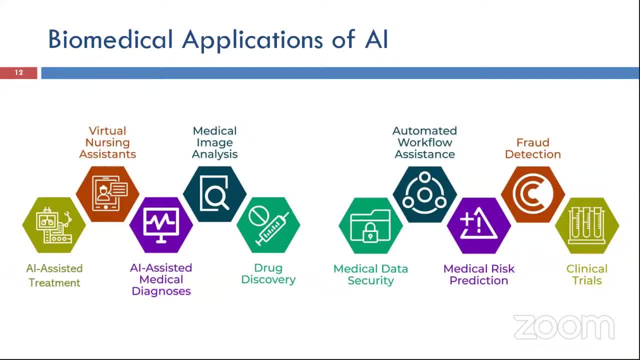 now we take into account the previous clinical trials and we may get from the AI system a confirmation with a lower number of patients. Let's talk now about the clinical trials. Let's talk now about the clinical trials. Let's talk now about the clinical trials. 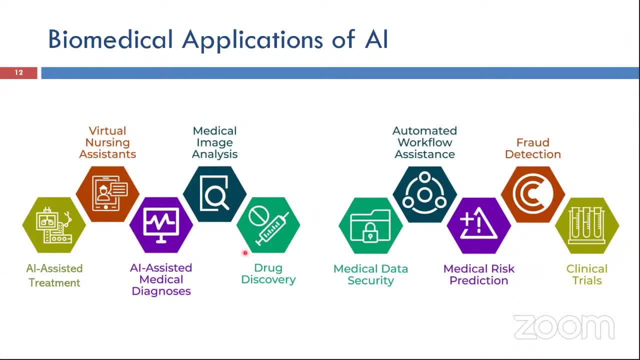 Thanks to the two applications. one is related to drug discovery, because you are actually one of the things that is considered modern, and we will talk later about the one. that is not related to medical diagnoses, because that is better understood: The idea of the medicine design. 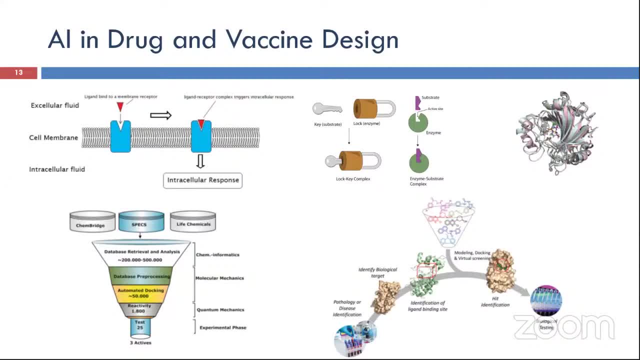 or the idea of the design of the vaccine is that, basically, you want this drug to get into a certain cell, The cells that you want this medicine or vaccine to get into, or you want to trigger a reaction in a certain way. Basically, you have to talk to the proteins in the cell membrane. 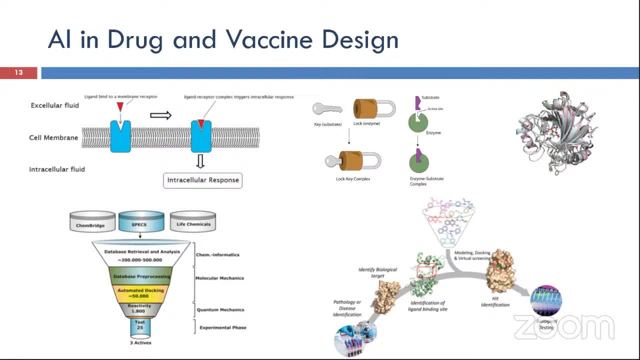 You can't enter the cell without going through the cell membrane, So the cell membrane is designed in a way that you can't enter any substance. You have to have a set of proteins like this And this set of proteins. you have to basically design something. 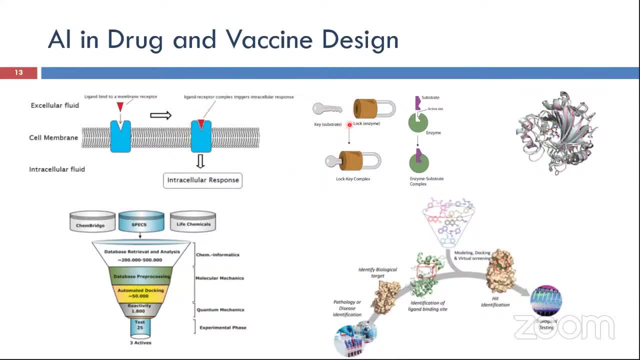 Basically it's like a lock and key. Basically, the thing in the cell membrane, the protein in the cell membrane, is like a lock. You want to use a key to open the lock which allows you to enter the cell to make an intracellular response. 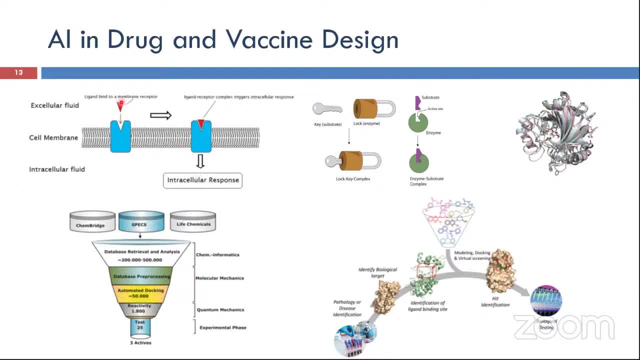 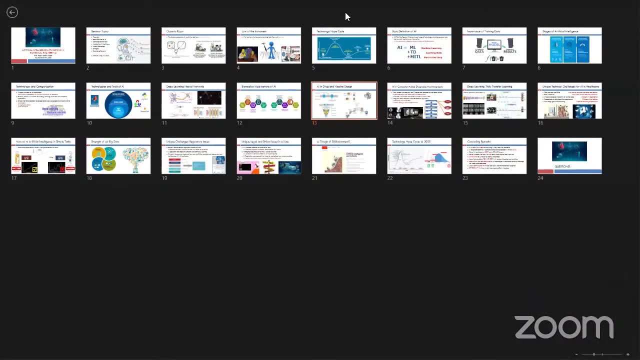 The problem with this is that if we imagine it like this, we can make all our drugs look like a triangle and that's it. No, it doesn't look like that. The protein looks like this. It looks complicated, Sorry, Okay. 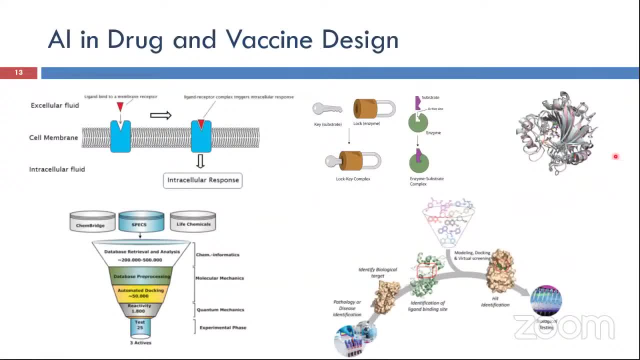 Okay, The protein looks very complicated. It has something called tertiary. What does tertiary structure mean? Tertiary structure means that it's three-dimensional, not two-dimensional, So it's basically to reach the place where you can put the key. it can be something internal. 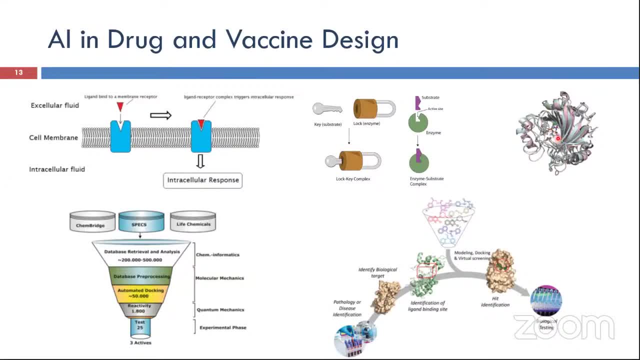 It's very, very complicated to design the substrate, or design the material, or design the vaccine which is at the end, to be able to plug in the keyhole in the cell membrane so that it can enter and make. We're going to talk about the design issue of the vaccine. 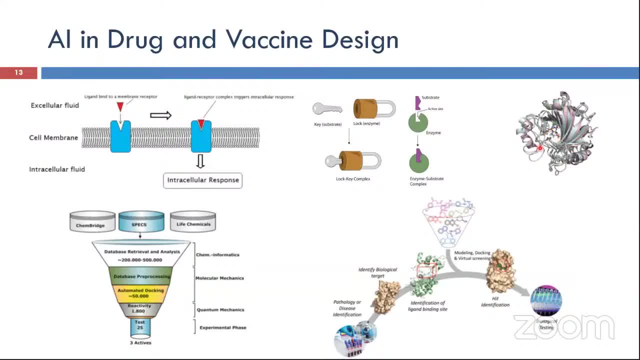 or the design issue of anything in drugs in general. We're talking about you usually starting from a database that has, for example, almost half a million compounds- if you can imagine half a million. You then start pre-processing it, you start filtering it. 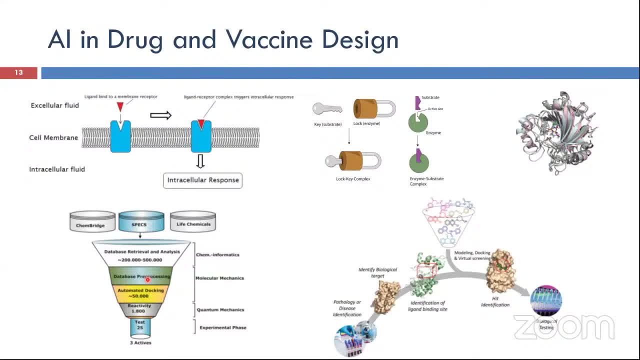 many steps and these steps are done in the first place in a practical way. Okay, People now start to interfere with the AI part and the AI part, and the AI part, it depends on something called chemoinformatics, something called molecular mechanics. 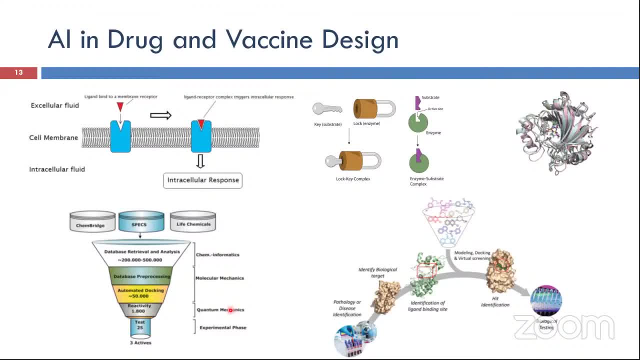 quantum mechanics and in the end, after it does all these things, it basically builds a system. It gives the part that makes the identification to take the things which are in this database and then start to test all these things. on the actual structure issue, 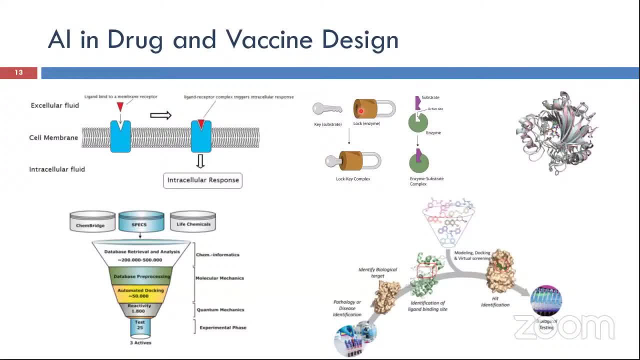 If it's a docking. maybe Docking is the question of long-term, that I put the key in the lock. Okay, Basically, in the end he does all of this in silico. In silico means you will see this expression a lot in real life. 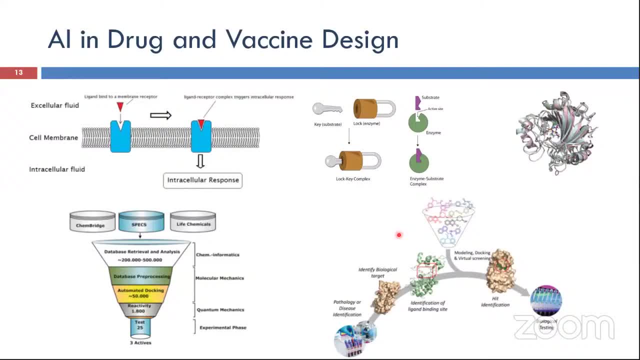 in silico means you talk about something. you talk about the drug itself. you do the practical experiments in the first computer before you go to the clinical trials on a patient. You talk about all of these stages in silico design and then you reach a small number. 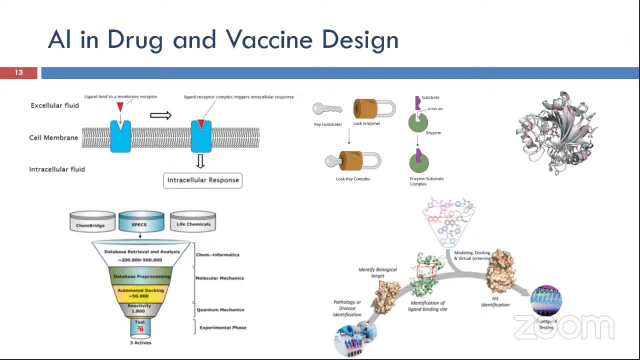 like 25 out of half a million. then you do the experimental phase on animals and then you take advantage of these three and then you go to the human clinical trials. We are talking about the drug design part, and the AI has applications to the full extent. 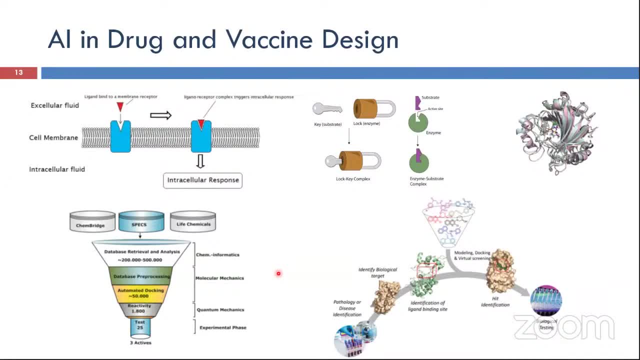 And of course we have seen usually when we talk about any drug in the world, if you look at the history of drugs in medical history, you will find that the average of the vaccine development or drug development takes about 10 years. 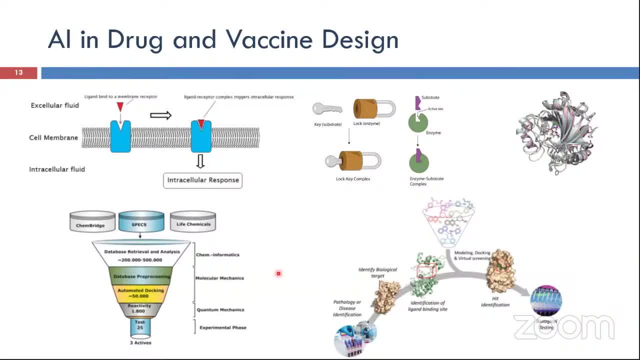 and it consumes on average about 3 billion dollars. So we are talking about what happened with COVID-19,. in less than a year, we started to have vaccines and there was production for it and, of course, after the clinical trials and all of this. 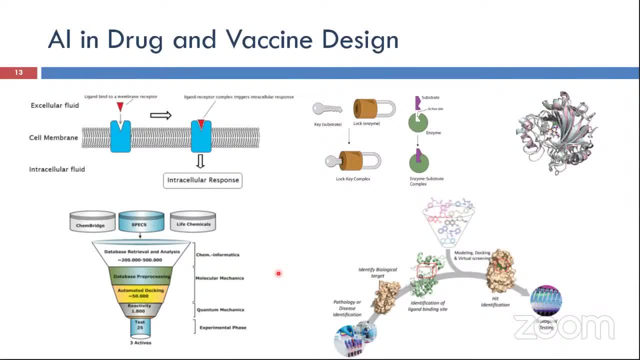 it was a miracle And, you see, in fact, a big part of it was for the intervention or the use of the enzymes which have the AI to help us track the candidates that we are going to test later on, Because if we test the candidates in a practical way in the first place, 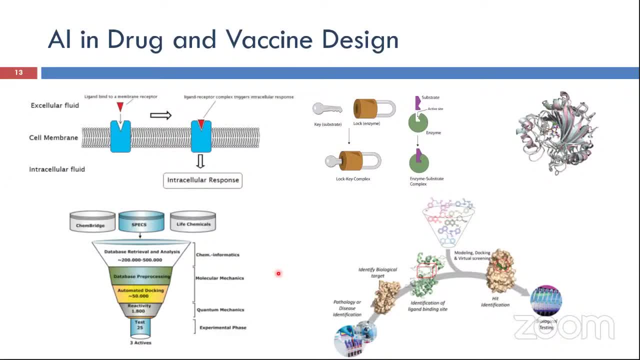 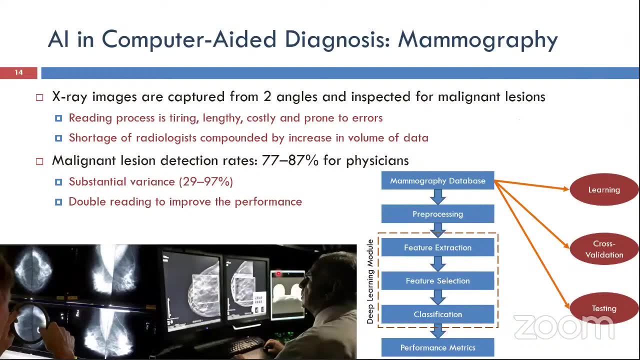 it will take a very, very long time to be able to make the vaccine at the right time. This is a very important life experiment. The second experiment that I am hoping to show you how this work is done is using the AI in computer-aided diagnosis. 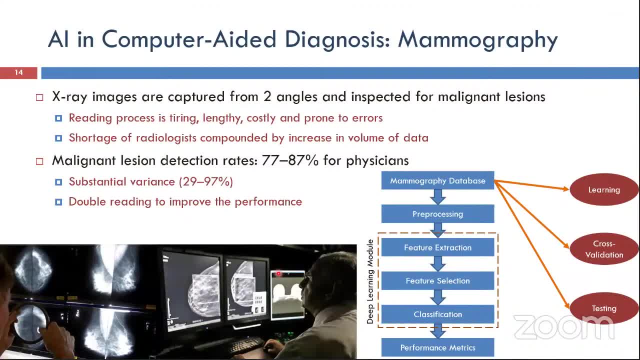 So we are talking about the problem in mammography, for example, in particular that it starts to be in in the skin, in the screening programs. It starts not only with the ladies who have a problem. they are the only ones who go to the doctor. 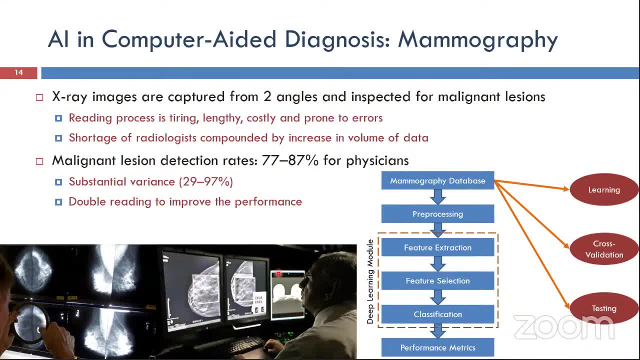 No, it starts now with the ladies who are above a certain age. It is advised that they go every year- or every two years according to the family history- to do mammography. So the mammography is made up of two pictures. one is a medullatory oblique. 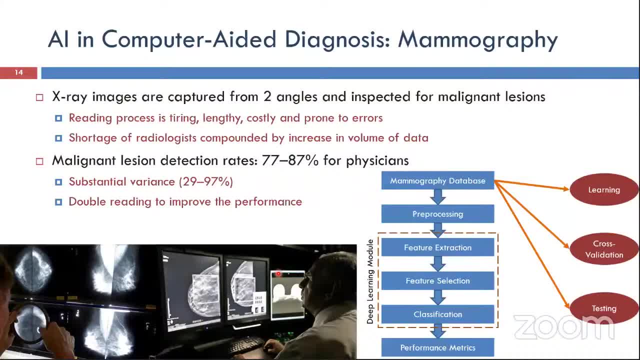 and the other is a cranial caudal. So two pictures from two different angles And in the end we take these two pictures, the doctor looks at them and sees if there was, if there is any beginning of cancer. we call them micro-classifications. 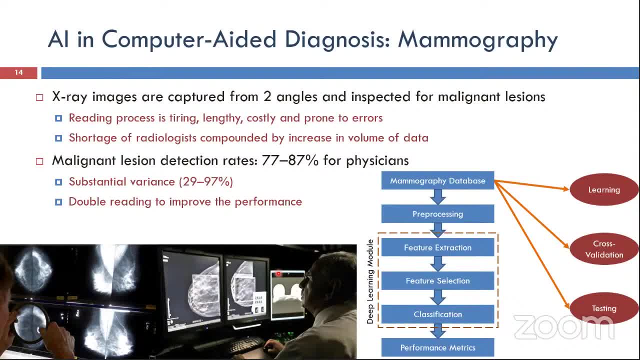 And micro-classifications are very small, like salt particles on the picture, And we talk about the picture of the mammography. we talk about the resolution of 5000 by 5000. So we imagine the doctor. what was he doing in the past? 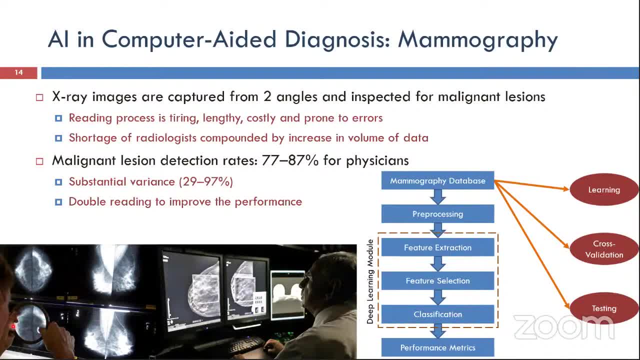 In the days of the film he was holding a magnified lens and he was walking on the picture point by point, because if it happened that he had, he had a place where there were micro-classifications and he didn't take care of it. 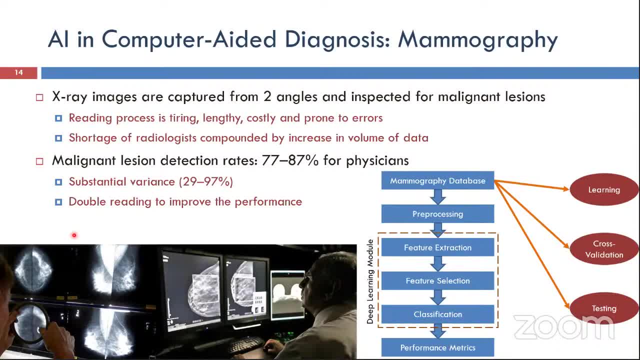 it became a big problem. The lady would go home, she would go back to her home and stay there and she would have micro-classifications and the micro-classifications would continue to grow. and so when she goes after that, for example for the screening test again, 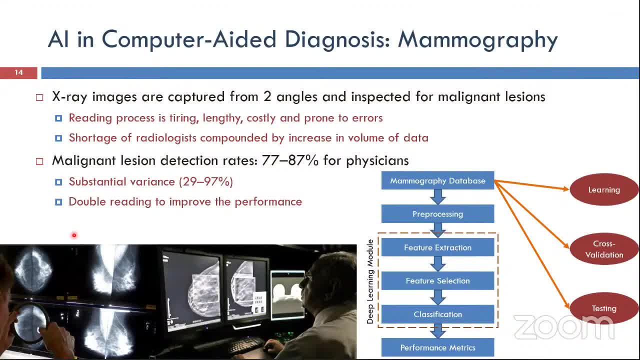 when she comes to do a mammography again after two years. her time would be in mass, So it's a problem now. Of course, when you know these things early, you know them early, so there is a great importance for detection of any problem. 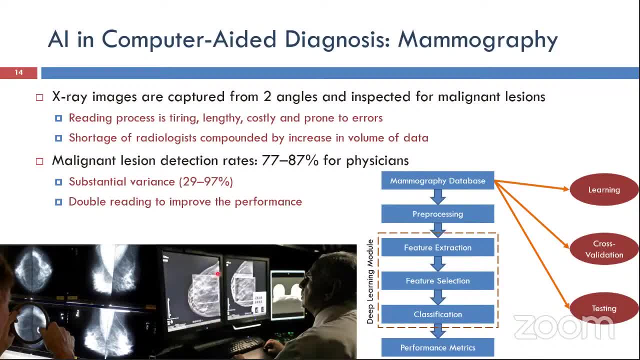 even if it's the first one. The person who is now all the mammography is now digital, so now he has a very, very high resolution screen. he can't see from this normal picture, he can't see from it, he can't make a diagnosis from it. 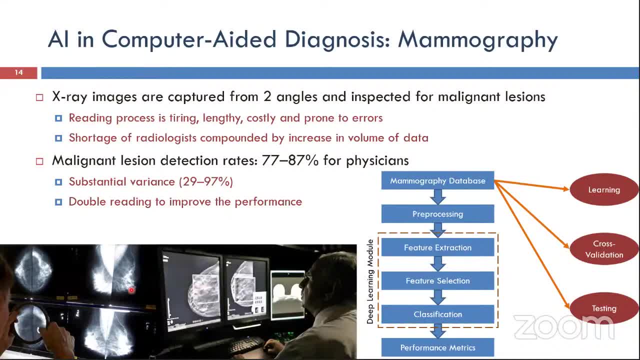 so he has to enlarge a part of the picture and he starts looking at it as if he's walking with a magnified lens, only on the computer. We're talking about the fact that the operation is very tiring, very lengthy, very costly. 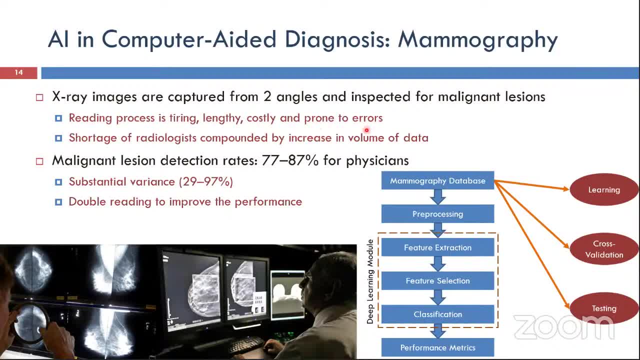 and of course there is a person who does it. there is a person who makes a diagnosis. he can work 10 hours a day. Of course his accuracy in the morning is different than at night, after he has worked 10 hours. 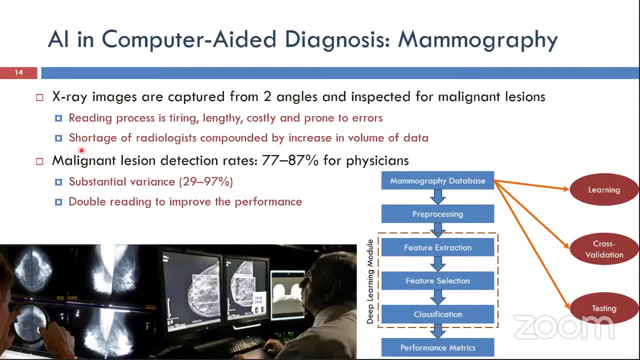 So of course there is a problem. The bigger problem is that we have a shortage of radiologists. We don't have many doctors. When we talk about screening programs, we talk about increasing volumes. The more people have awareness, the more people go for screening. 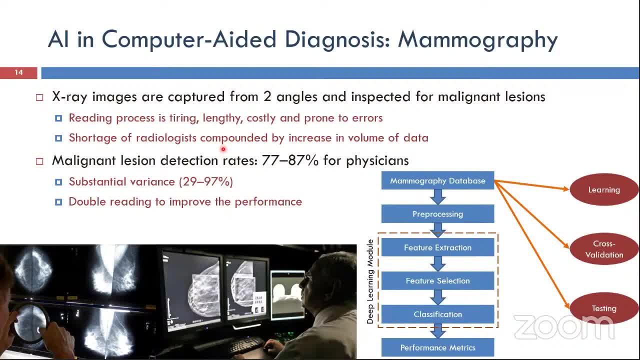 so the volume increases. So we have a problem. In order to ensure that the screening is done properly, it is better to have two doctors looking at the picture, not just one doctor. So there is a real problem for this area. This is a motivation that makes people think about. 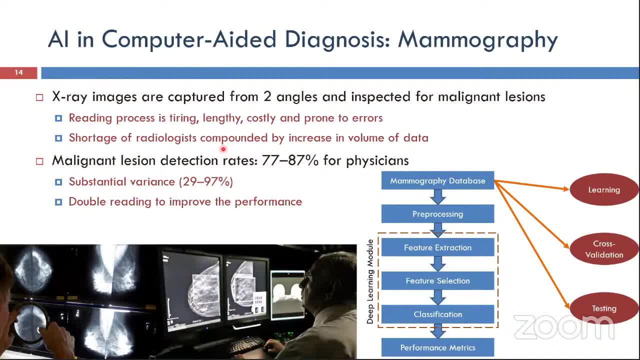 the computer-aided diagnosis in order to use the screening. We're talking about the average rate for physicians from 77% to 87%, but there will be a wide variability: We're talking about from 29% to 97%. 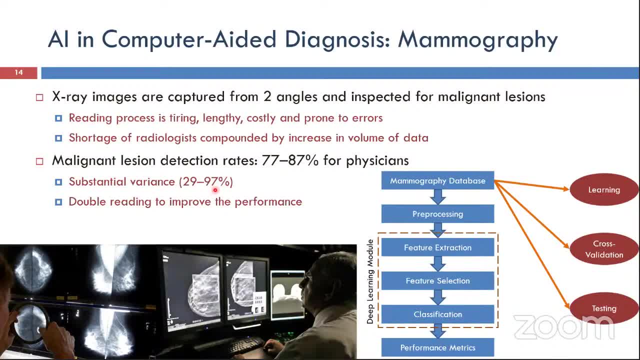 but there will be a wide variability. The range is very wide, So from a new list of doctors who don't have experience to a trained doctor who looks at the picture and always knows the problem without anyone else seeing it. So of course we're talking about a very important double reading. 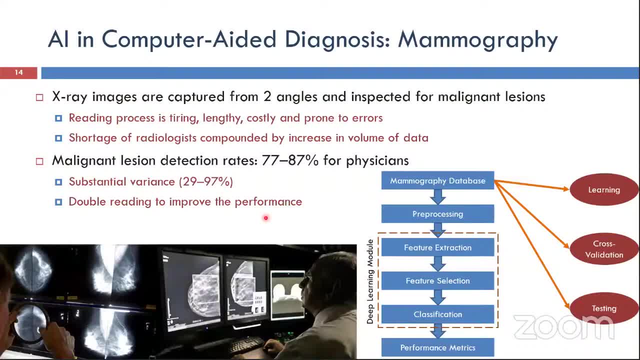 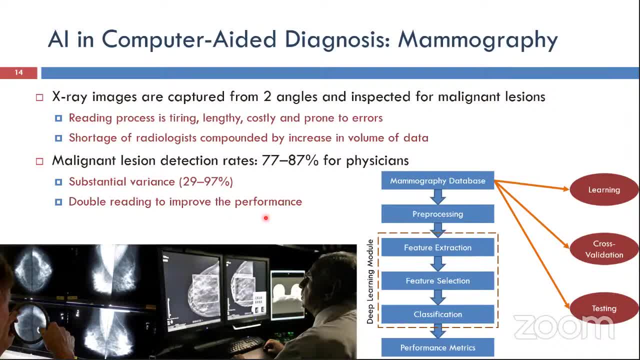 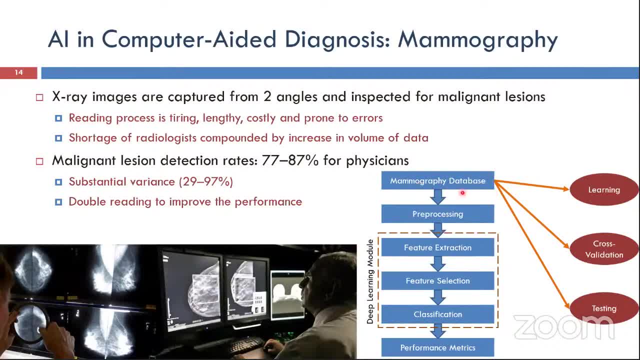 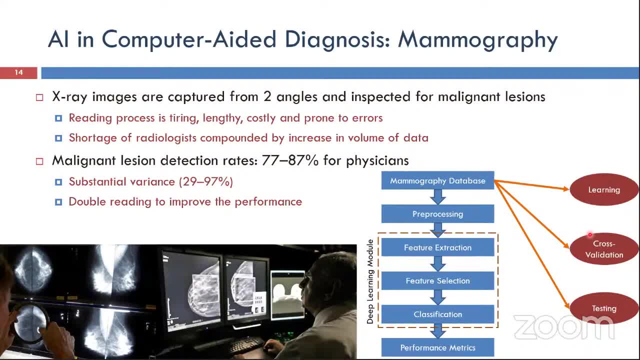 you solve it, but you don't know many degrees. But in the end, if you don't know how to solve it, you ask the doctor to understand it. In the end, the final exam is the testing data. This is what tells you. 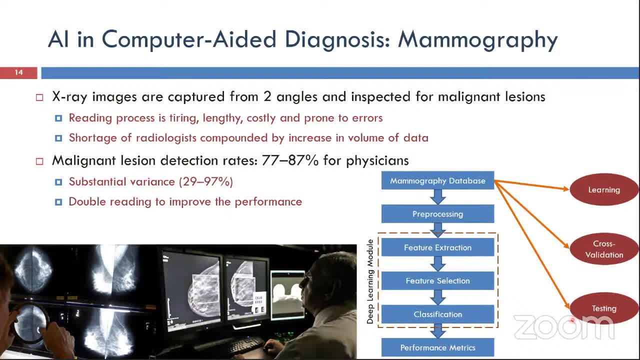 if you really learned this thing or not. Okay, So of course there are many stages, In fact, for machine learning. there is something called feature extraction, something called feature selection, something called classification, Now in the deep learning module, 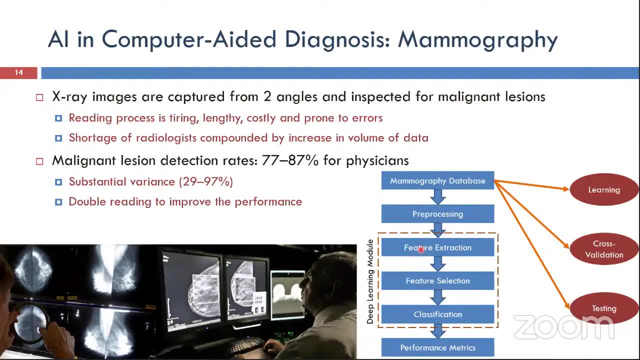 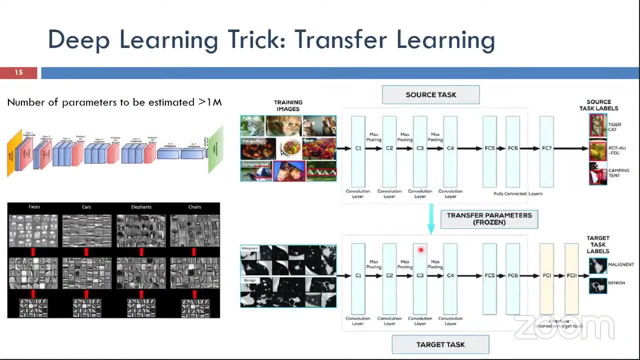 there are three things. You don't need to separate the three things. You take the pictures immediately, you get a diagnosis immediately. you learn the system from the pictures directly. In fact, deep learning is one of the things that really has potential. 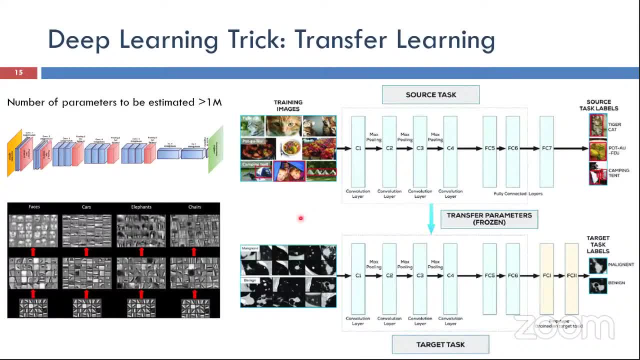 but the problem is, when we see the number of parameters that you have to make an estimation, you get more than a million And maybe actually some types of deep learning are technology. We're talking about 50 million parameters. 50 million parameters. imagine you have 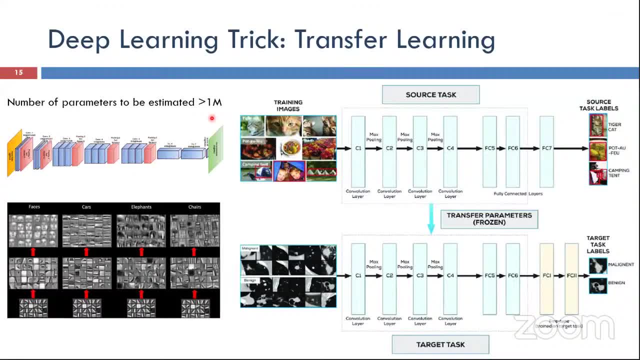 a polynomial, for example. second order: There's x squared x plus one, for example. Each one of them has a1 or a1, x squared plus a2, x plus a3 or a2, a3.. These are three parameters. 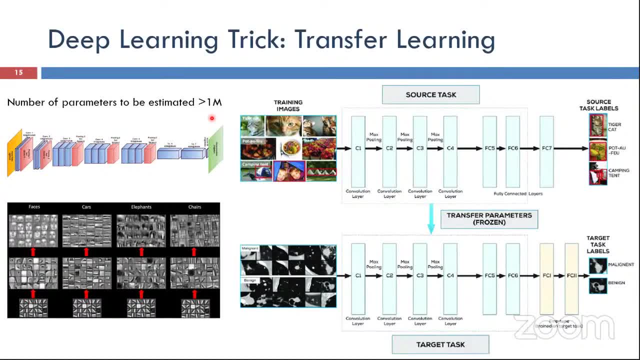 for a simple thing, I think. So, in order to make this polynomial have a certain behavior, you have to learn a1 and a2.. The same thing for the neural network. Your problem with the neural network in the medical instruments is that you don't have a million cases. 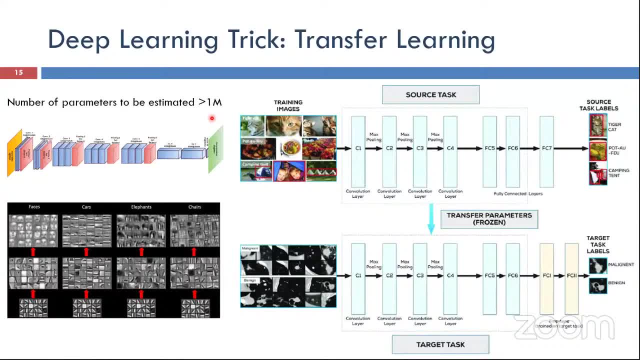 When you collect 100 cases, you've done an achievement, So you don't have all this data. There's one very nice trick in the deep learning called transfer learning. People noticed something very nice about deep learning. This all looks like neural networks. 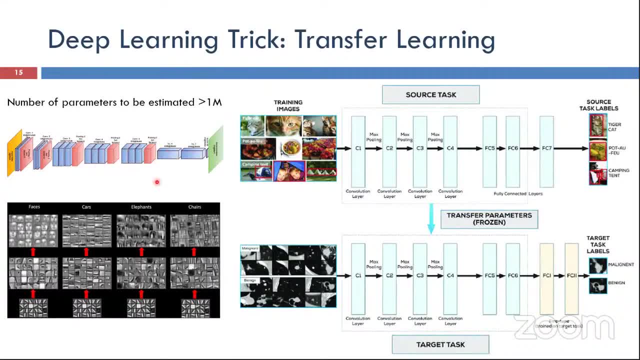 but I put it like this because it's just a display for you. This one is called this and this one is called that. Notice something very nice When they teach neural networks with faces, or with cars, or with cars or with chairs. 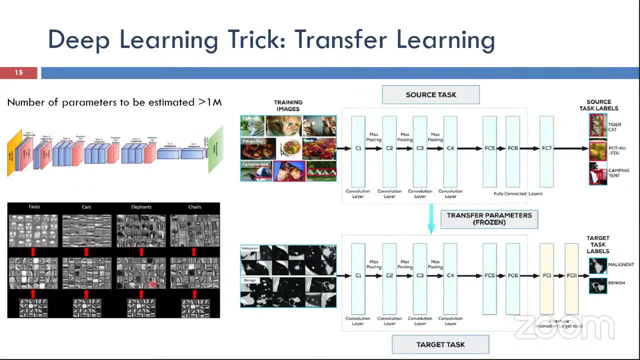 they found that in the end, the initial stages remain the same. In the end, you reach that things are similar at first. Let's do something a little better. We take a database or a network that is already taught in many pictures, If you saw, for example. 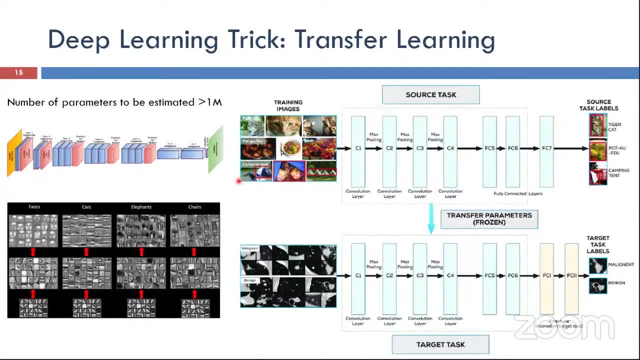 we have a database called ImageNet. It has a thousand types of pictures And we can talk about more than a million pictures. Basically it has pictures of dogs. pictures of dogs, pictures of children, pictures of cars, pictures of traffic signs. 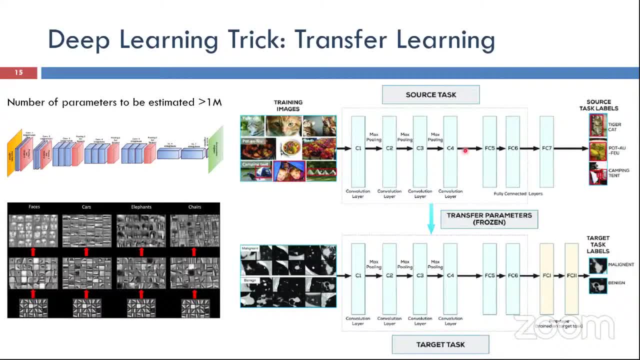 and many other things. We can take a network trained to teach these things and we take only the part at first. the part that I'm telling you is similar here. we take it as it is and we learn the last part to fine-tune it to the malignant and benign. 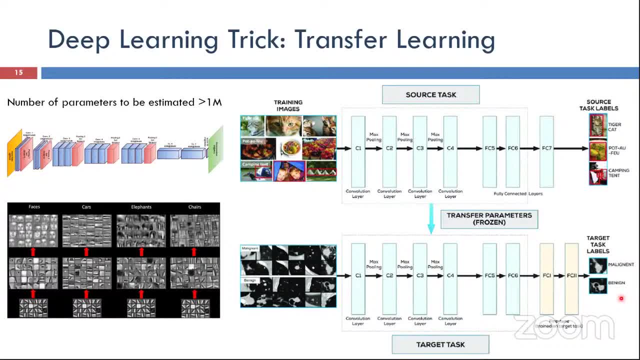 that we were talking about. These are the medical things that we want to distinguish. This method is very different because it really made the reliability of the techniques higher. the speed of training is much better and therefore you now have a chance to get reliable results. 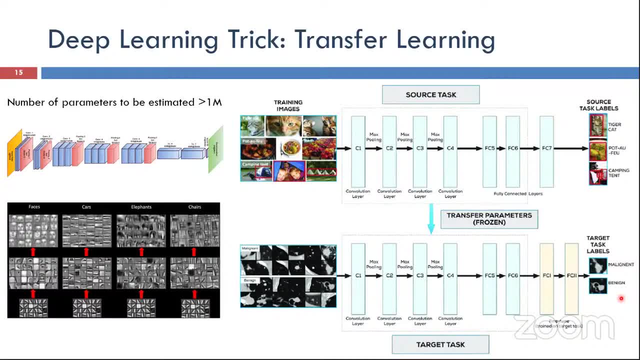 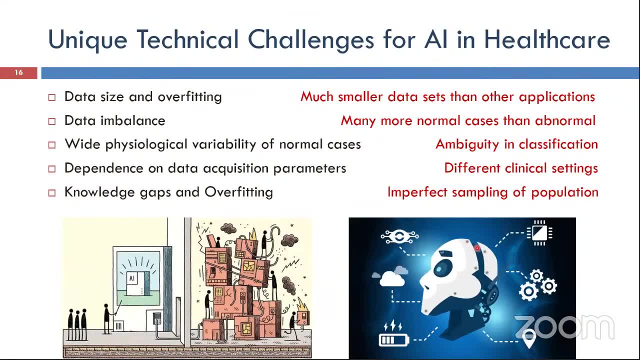 from very small datasets in medical imaging. If we talk about the unique challenges, the most important part of them is the data size, because this is really what we have a problem with: much smaller data set than other applications When we talk about self-driving vehicles. 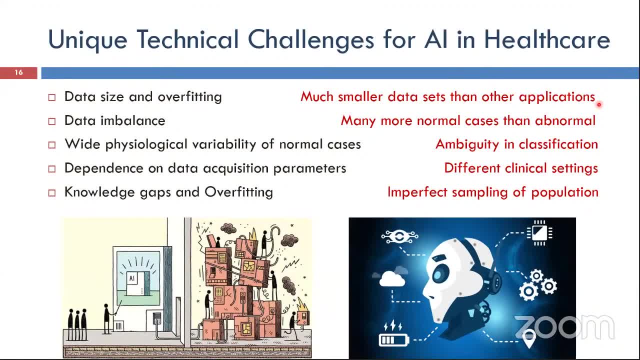 for example, cars that drive by a driver. he can walk all day to collect pictures. for a year. He can take millions of pictures. The things, for example face recognition technologies. people are afraid that governments will take them. they will use them. 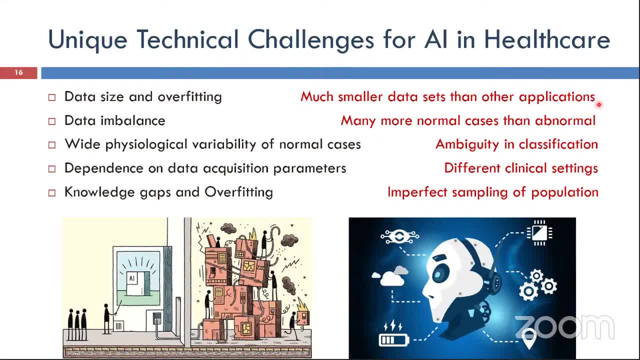 they will use them for bad things. Google had a system, Microsoft had a different system. We already have systems like this, of course, in China. in real life. We talk about billions of pictures in other applications In medical engineering. you will find that when you talk about collecting data from a patient, 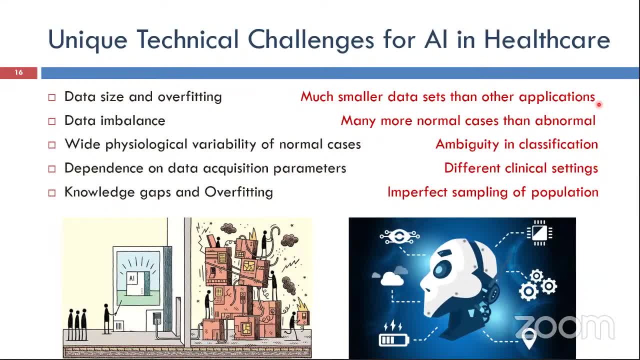 you talk about datasets. when you talk about having 200 or 300 cases, you have done an engagement. If you get a thousand cases, you are unique. you are not like the rest of the world. This is a big problem. The data size and the overfitting are linked together. 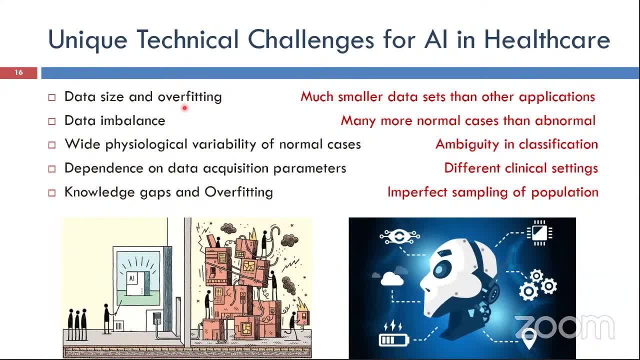 When you talk about overfitting, it means that you want to use a fitting for a polynomial First order with a polynomial, for example, 10th order. We will see this in the next slide. I will explain the overfitting problem. 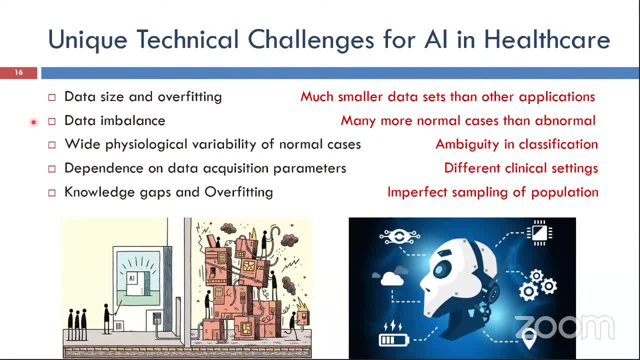 These two are working together. The other thing is that you have data imbalance. You want to learn the system, the malignant and the benign. To learn it correctly, you have to give it a number of examples of the malignant and the benign. 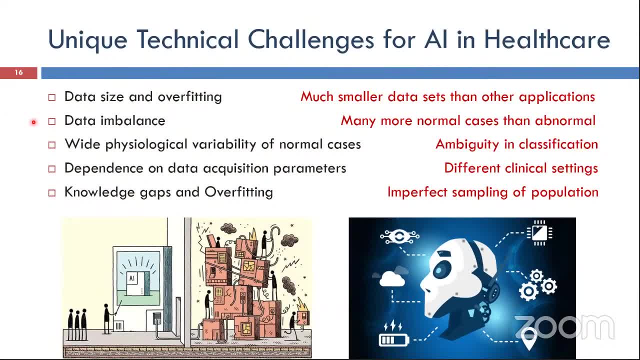 If you don't do this, what will happen? There will be bias. Bias means that the outcome of your system will be biased towards the thing that had more data, because it sees that it is most likely that these things will come out. This means that let me go towards the thing that has more data. 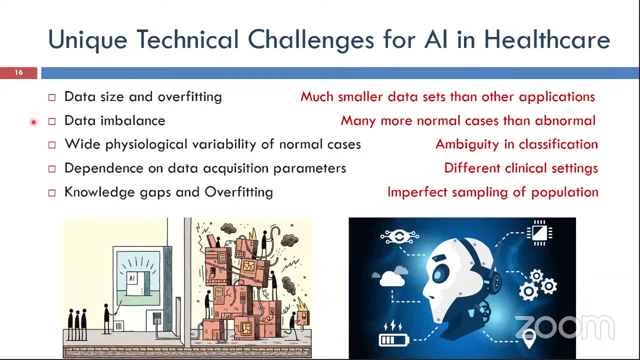 because it sees that it has more cases. Of course, in the case of disease databases, you will always find that the number of cases of diseases is less than the number of normal cases. When we talk about screening in mammography in particular, we are talking about the number of cases that have malignancy. 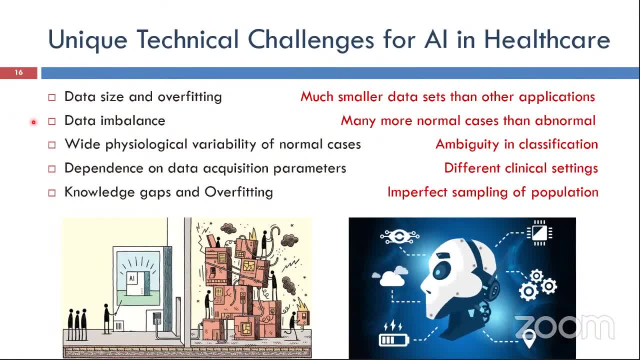 In the case of the total, we are talking about 1%. It may also be less according to the community. We are talking about a much lower number of abnormal cases. Therefore, we are talking about a much lower number of abnormal cases. 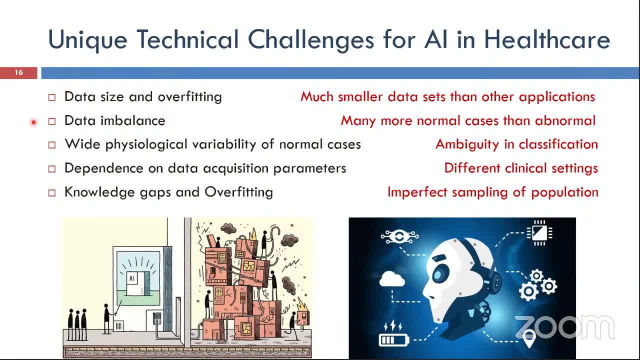 We are talking about a much lower number of abnormal cases. Therefore, we are talking about a much lower number of abnormal cases. Therefore, we are talking about a much lower number of abnormal cases. We have a wide physiological variability. You are talking about that. the same people who are normal. 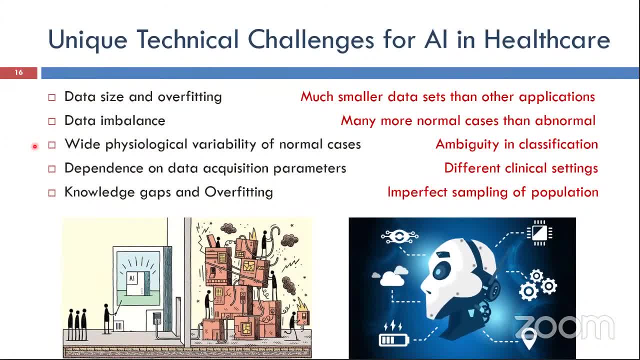 who do not have diseases. if you took their medical photos, you will find that there are very large differences in the normal. Therefore, you will find that you have ambiguity in classification as a result of the wide distribution in the normal. Therefore, when there is abnormality, 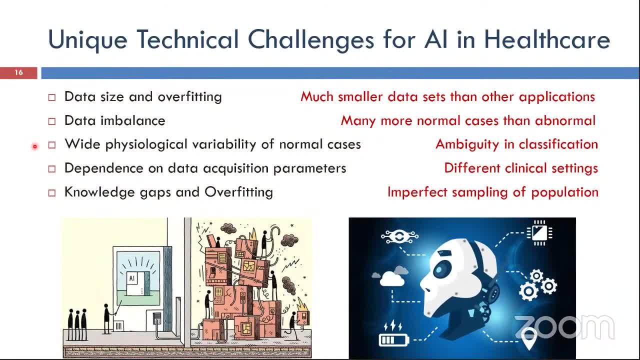 abnormality may really be abnormality, But it is actually something very similar to the normal for other people. Therefore, you have a problem in this matter. These problems are really unique to biomedical engineering. We are also talking about dependence on data acquisition parameters. 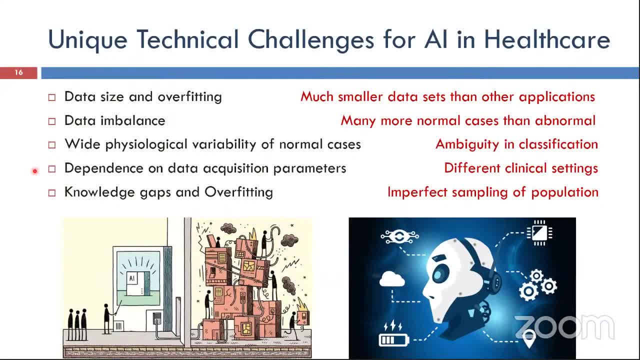 If I now took mammography photos taken in different ways, in different angles, I entered the same system that I was telling you about a while ago, or rather, instead of taking from two angles, I took something different In a different way. 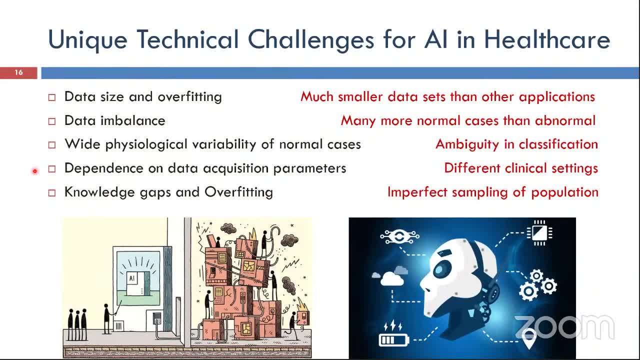 I changed the way I took the photos. Once you have changed the way, it means that you have to learn your system in a different way. Therefore, if you have learned your system in certain settings, you have to keep the same settings for all cases. 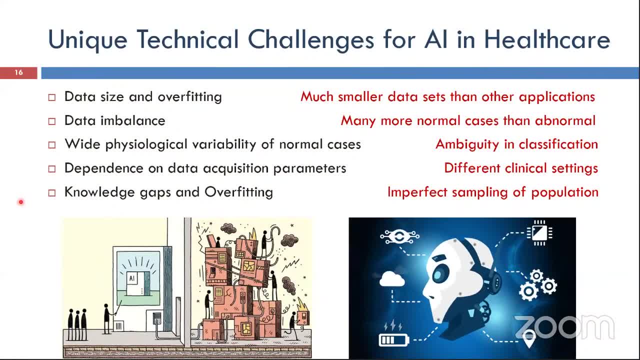 so that you can use it in a simple way. And, of course, in the end you are learning something like a monster. You are learning something very big with a million parameters. A million parameters. You entered some of the cases and it turned out that they were identified correctly. 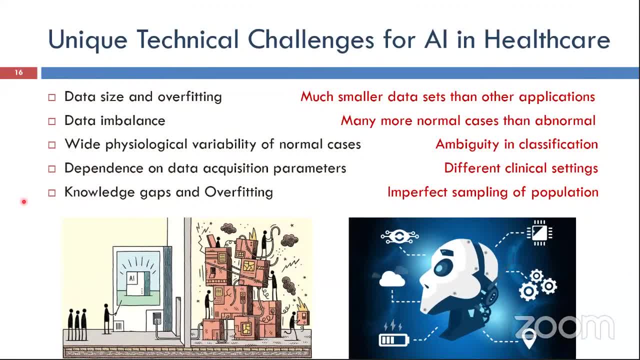 Do you know what is inside? Do you know that it is actually identified or made a complete system so that if you bring it new cases that you have not seen before, it will be able to act in them correctly? We have a big problem called knowledge gaps. 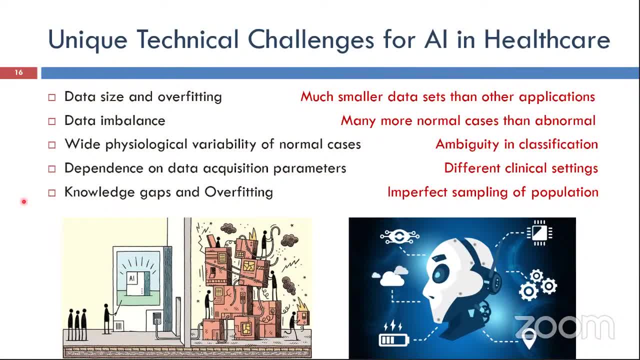 in neural networks in general. People talk about it for 90 years. This is also not related to overfitting or other things, but it is really not related to imperfect sampling or population and it is also not related to a small data size. 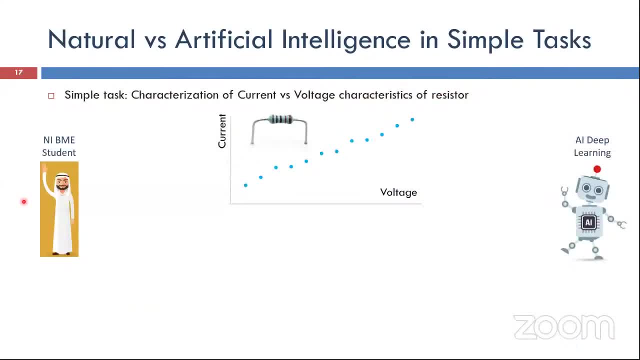 Let us take an example like this, A very nice example We all took in the circuits: how to calculate the resistance of current and voltage measurements. We will now make a challenge between the natural intelligence of a biomedical student and artificial intelligence as represented by deep learning. 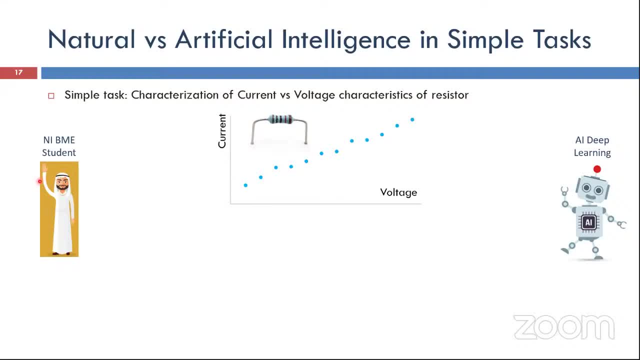 The big game. So, basically, a very simple task. We have data. We want to see how this data is represented. How do we make a model of this data using a smart person, a smart human and artificial intelligence? So what is the result? 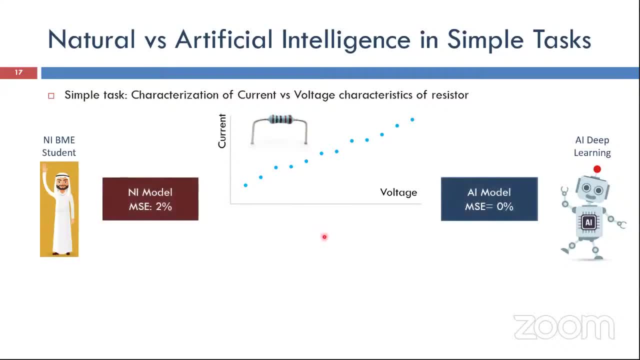 We will find what happened Basically for the natural intelligence model. the mean square error of the model was 2%. For the AI model, the mean square error was 0%. Any few are better If we want to look at the numbers. 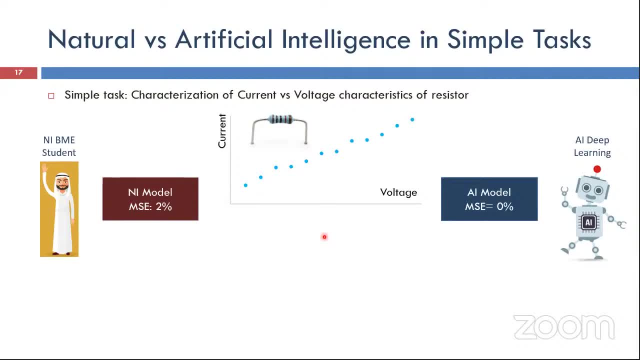 the AI model will look like this. There is nothing better than this. It is a zero percent error. In other words, it is a perfect model for this data. Let us look at it a little more. Let us look at how the model looks like. 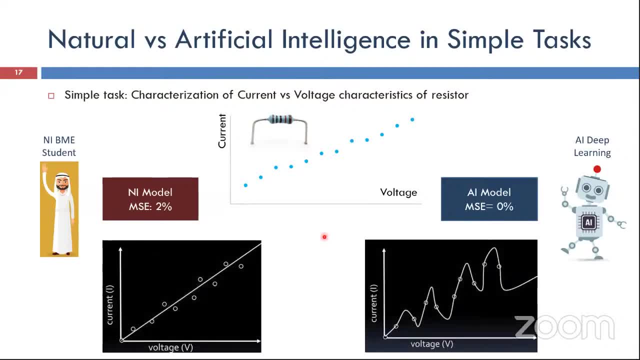 The model that the biomedical student came up with is a straight line that runs in the middle of the points that he has calculated. Basically, this is the model that he came up with. He thought that with his intelligence he saw that there is something called Ohm's law. 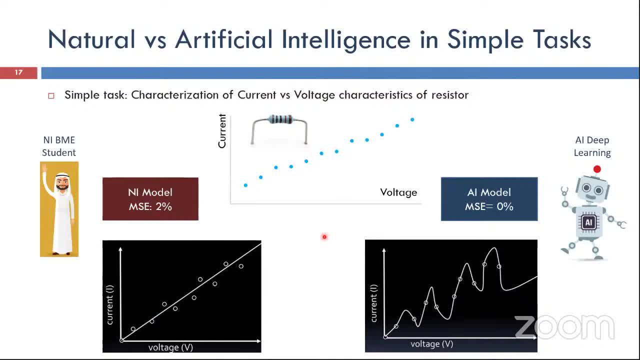 It is supposed to connect the current and the voltage that pass through the resistance. Therefore, he made a fitting with the correct model, which is considered a linear model. What happened to the AI model? The AI model does not accept that, you say. 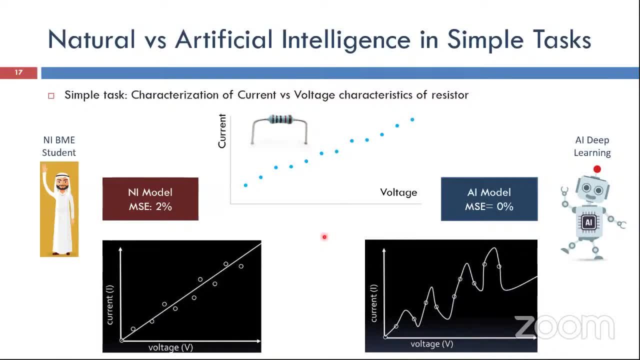 I swear this is Ohm and so on. It does not answer Ohm. It is better than Ohm. Basically, it takes the data and interacts according to the data and learns from the data. The point is that, unfortunately, in the AI 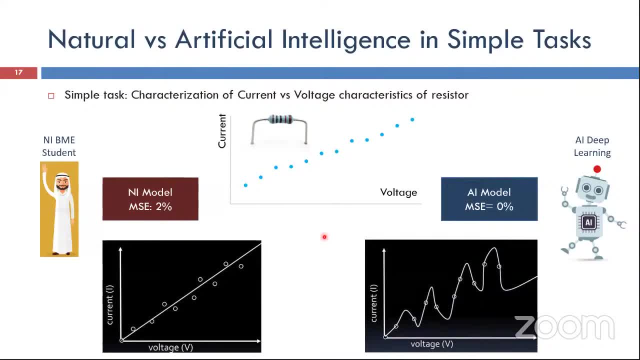 you will find that you have the main goal in the deep learning algorithms: that you fit the data. If you do not understand this data, what will you get at the end? You do not have a model at the beginning. You have a concept that the model is supposed to be like this: 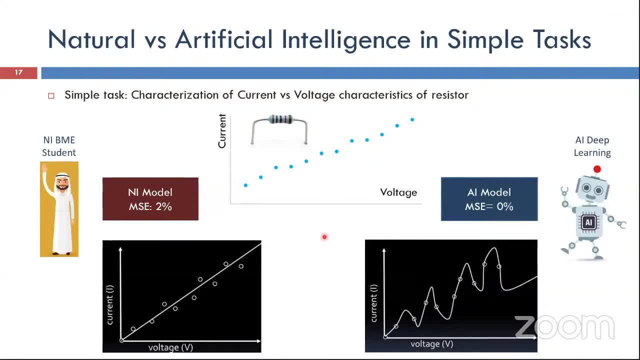 in order to be built on the basis of the model Or in order to fit on the basis of the model. Therefore, you get something that does not make any sense. in this way, The error is zero. It creates a curve and passes through all the points. 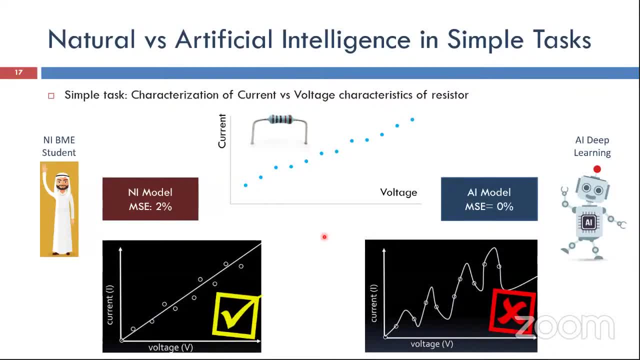 But is this curve correct? No, it is not correct. Basically, we are talking about that in this case, the solution created by the natural intelligent student can be better than the solution created by the artificial intelligent deep learning system- The situation we are talking about here. 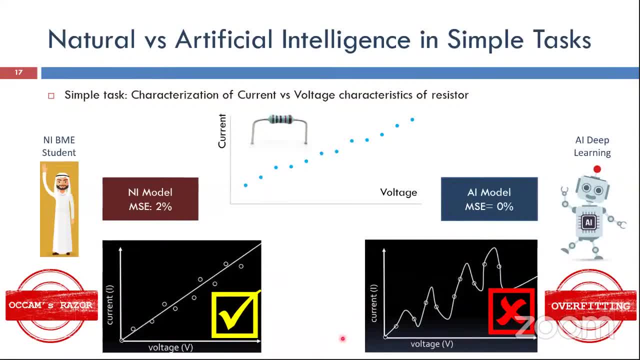 is something called overfitting. Now we have data that is supposed to be linear. The idea model is linear. It was created in a much higher order, So basically it looks something like this: The things that are supposed to be logical. 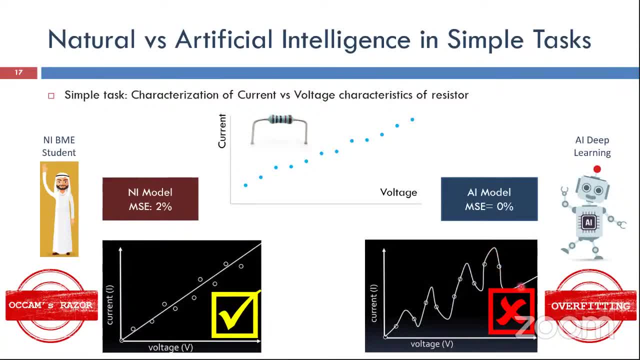 are done in a non-logical way. Therefore, this is rejected and this is accepted, And this is what we are talking about. that it is a very clear application of the Occam's Razor, If I told you, without telling you, where these results come from, 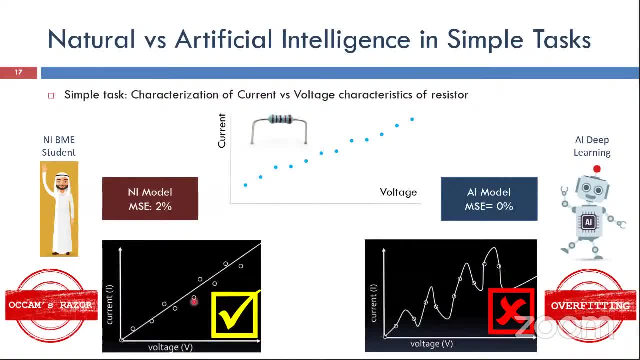 If I told you that I have a model that looks like this and there is a model that I have that looks like this, You have to accept this model with the Occam's Razor, Because this is the simplest explanation and it really looks logical. 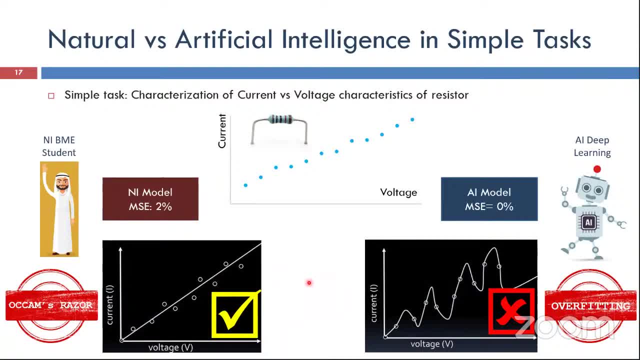 So a very important advice: Artificial intelligence is not for all problems. Artificial intelligence is made for problems that deserve to be put in the resources of artificial intelligence. Artificial intelligence is made for problems that deserve to be put in the resources of artificial intelligence. 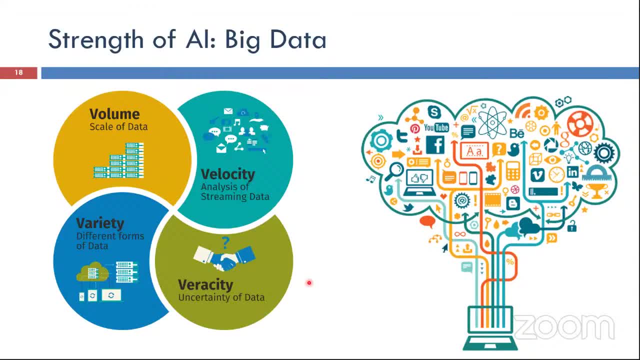 The strength of AI comes from big data, The thing that I can't handle. Natural intelligence can't surround it Like big data. Why do we talk about the scale of data? The volume is huge. I can't look at it. We talk about the treatment of the patient. 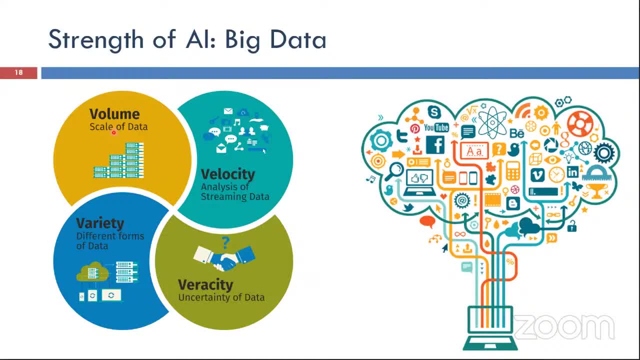 in Saudi Arabia in the last 50 years. Very nice, If you have this data, you can go through it, You can get information from it. Big data means that you have velocity. Big data means that you have velocity. It means that the data 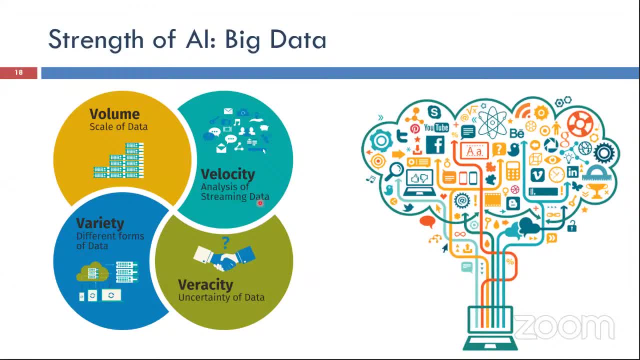 has a very high rate, For example, the data of COVID-19.. You want to know the cases in the whole world, For example, WHO wants to follow the spread of the virus. It means that you have data from all over the world at the same time. 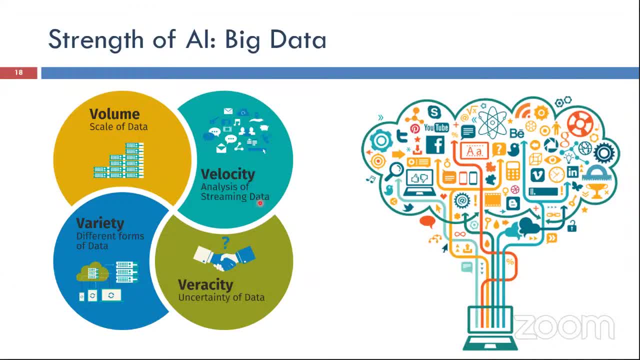 You have to think about it all. You have to see this data. It gives you an indication of what will happen. We talk about the uncertainty of data- Some data, Not some data. You have to know that all the data you take has errors. 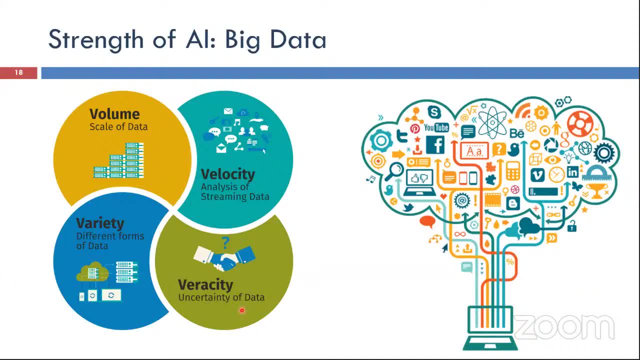 It has noise. basically, There is no data that is completely clean In big data. how do you have the problem that you have to check the data and use something that has a meaning and throw it away? Variety means that, for example, for the patient, 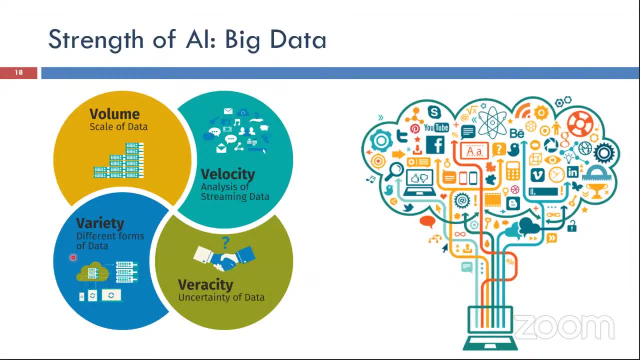 you have pictures, you have analysis, you have medical specifications, you have a medical record, Data with different shapes. It is supposed that all this data, if you have an artificial intelligence system, you take it and put it on the computer. At that time you can put algorithms. 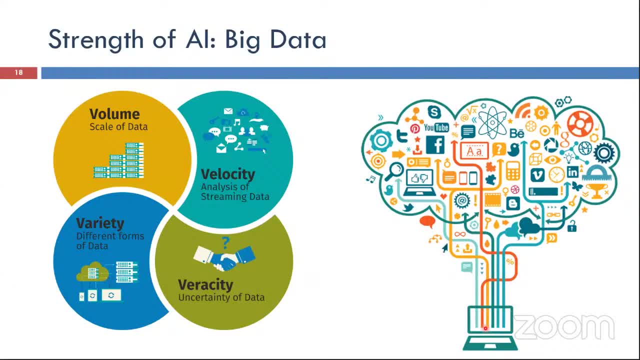 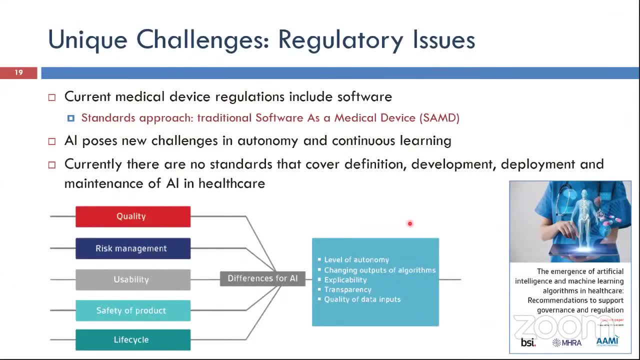 to help you, and artificial intelligence to give you results that you can't get from humans. Regarding regulatory issues, there are a lot of problems. The platform, in short, because of the time and because I wanted to show you what I was telling you earlier. 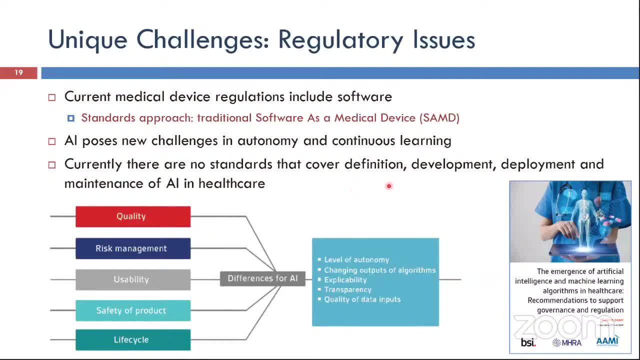 we don't have standards at the moment that govern AI. You have a big problem If you want to use a product that works in a hospital and has AI. you have a problem that you don't have a framework that you can use and people can accept. 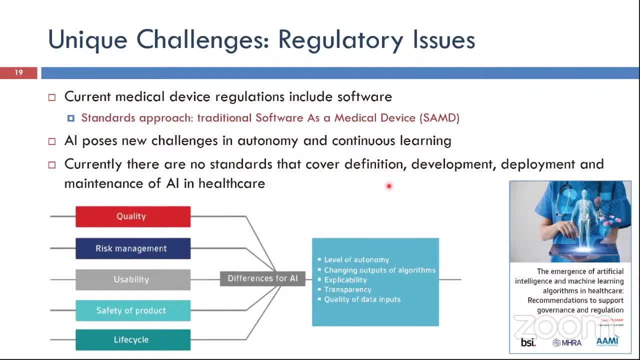 that, once you have achieved it, the product is safe. The issue is still there, People are talking about it, but there are no standards yet. Currently, the existing standard is software as a medical device. It deals with software as a medical device and puts 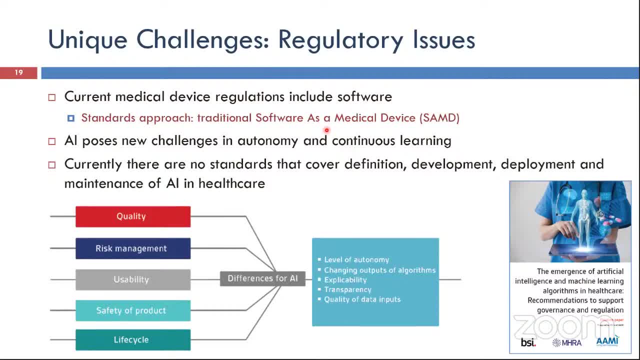 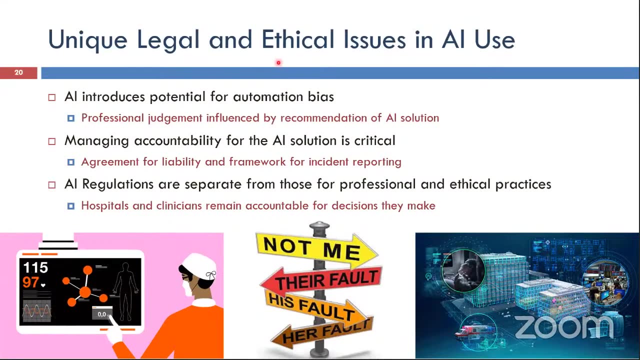 risk management. Basically, the same standard is used in regular medical devices. to make an application on the software, We still have time and a lot of work in the part that is related to regulatory issues. Regarding the part that is related to statistical issues, 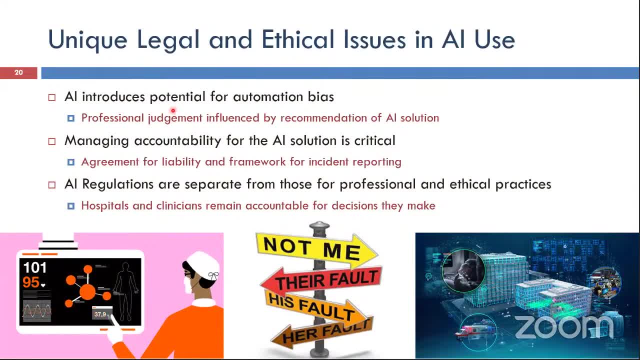 this is important. First of all, AI introduces potential for automation bias. What does this mean? This means that the professional judgment of the doctor can change or can be affected by the recommendation of AI. For example, we talked about the CAD system for mammography. 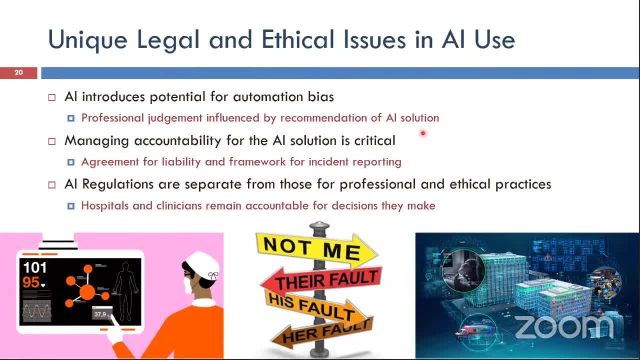 We talked about the possibility that the doctor can have an opinion and the doctor can confirm his opinion from AI. Now the doctor can see the output of the AI and immediately be biased by it and say that there is a problem. This is a problem. 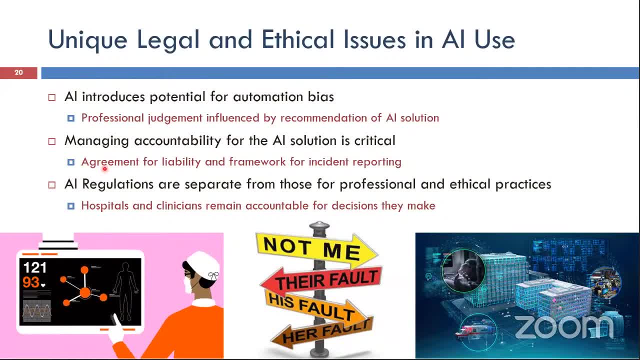 The second thing is the liability. on whom Does it depend? on the people who made the AI solution or on the doctors? We have to make sure that the liability is always on the doctor. Their choice of AI and their use of the AI system falls under my responsibility. 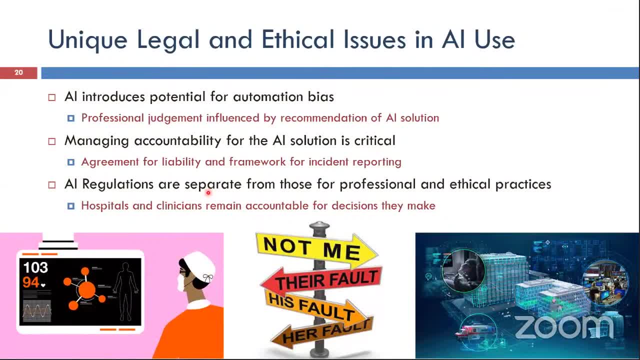 I cannot say that the responsibility of the AI is on the AI. This is a very important thing to consider. AI is considered an assisting tool. Basically, we can say that it is like taking a prescription from a doctor and making sure that it is okay. 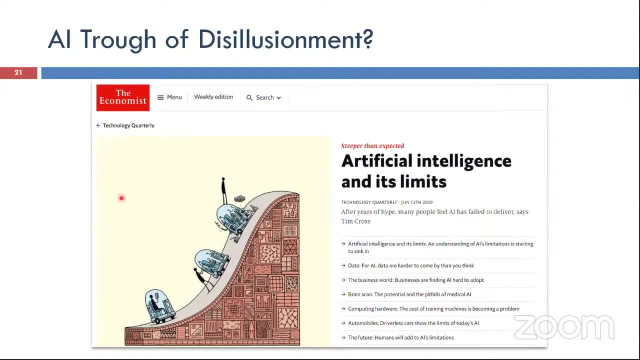 There is a very nice technique by The Economist, one of the well-known journals. He says that, after years of hype, many people feel that AI has failed to deliver. He says that, after years of hype, many people feel that they have entered the trough. 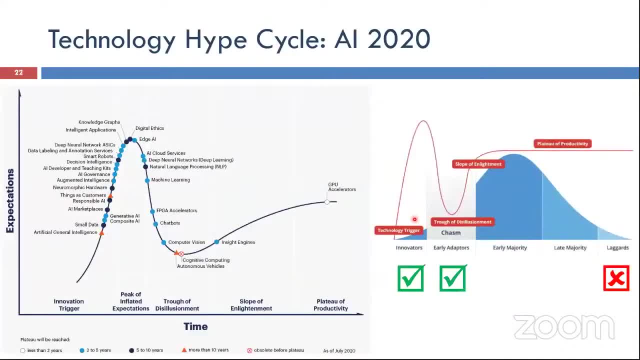 of disillusionment, The trough that we have here. Actually, if we look at the technical report of AI in the world in 2020, we will find that artificial general intelligence is still here. We will find that deep learning is still in hype. 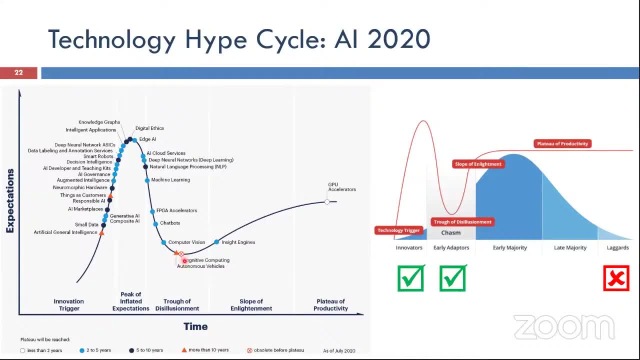 Machine learning is still the same. We have some technologies in computer vision that have reached the trough of disillusionment and stopped here. After that, no one is pursuing anything else. People have been working on AI for more than 10 years. People have been working on it for 10 years. 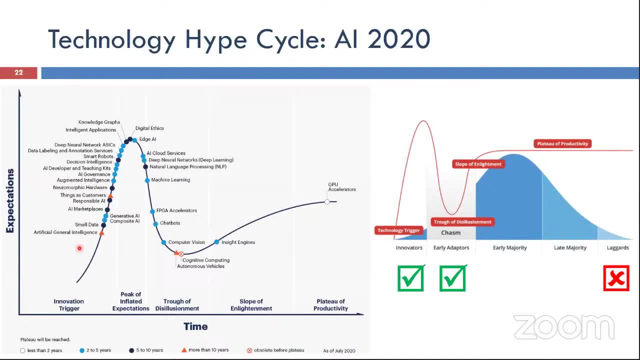 and they have not found anything that is really reliable. We are talking about something that in AI, there is still a lot of work to be done. We have an opportunity to talk about this spectrum. Usually, we start with the innovators in the first part. 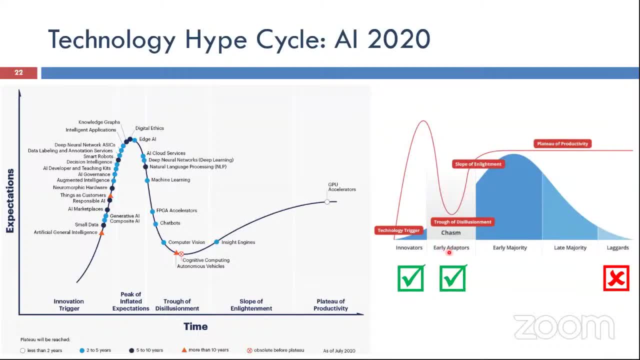 in the technology trigger In this part. if you started with the technology, you will be in the early adopters. After that you will be enlightened a little bit. You will have applications as products. You will be in the early majority. 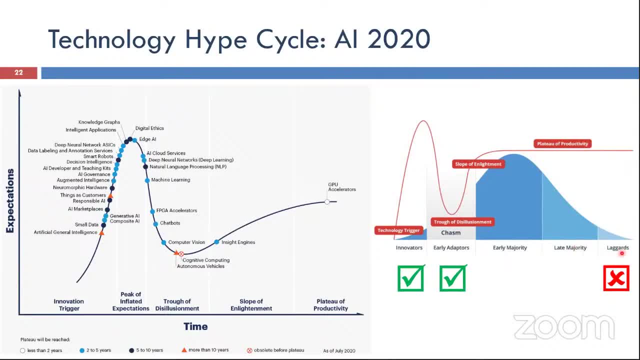 Then the late majority, Then the laggers, the late adopters. You have to always try to be in these. Either you are an innovator or an early adopter. This is an opportunity for us to talk about the laggers. 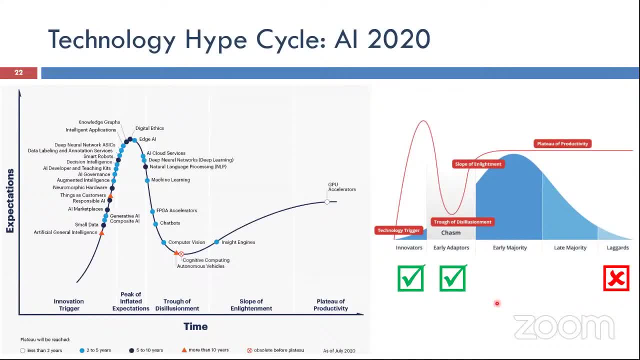 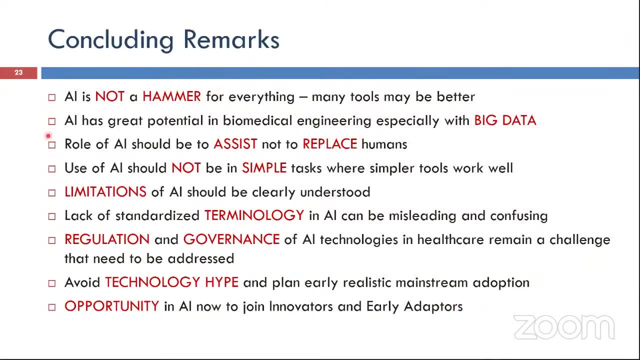 After that, people have done everything and you are ready to buy it. You have the strength to be in the technology. Concluding remarks: AI is not a hammer for everything. Basically the only tool you have. You have many more tools that may be better. 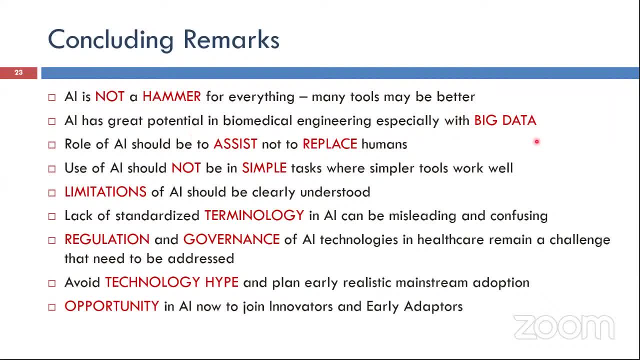 for the particular problem you have. AI definitely has great potential. by American engineering We are talking about. the role of AI should be to assist, not to replace humans. Use of AI should not be in simple tasks, as we have seen If you tried to make it. 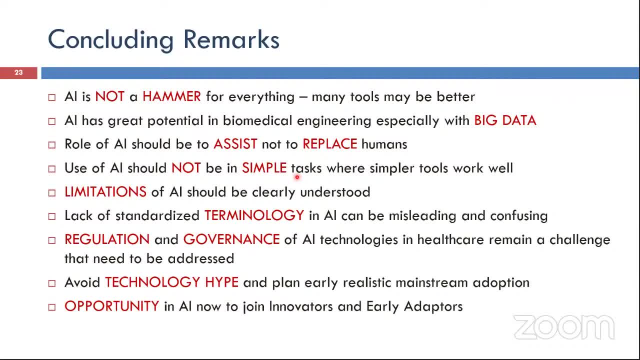 do something simple. There are many people who want to put AI in everything. For example, there is no artificial intelligence to turn on the elevator. Why? There are many other things. We have to understand the limitations of AI, especially in our field. 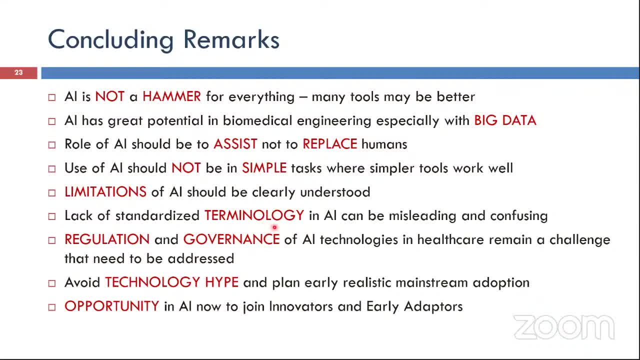 The lack of standardized technology is a problem. Try to understand AI through the three items we talked about so that you can compare different technologies. Regulation and governance are very late. We will see what they will reach in the end. It is very important to plan early, realistic. 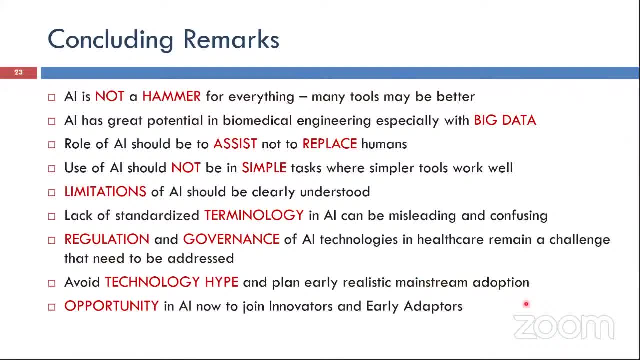 mainstream adoption. Think about applications that are reasonable. AI will not enter the hospital and do everything. There will be no people in the hospital. The hospital is all about AI. Think about logical applications and employ AI in something that is powerful and used in mainstream products. 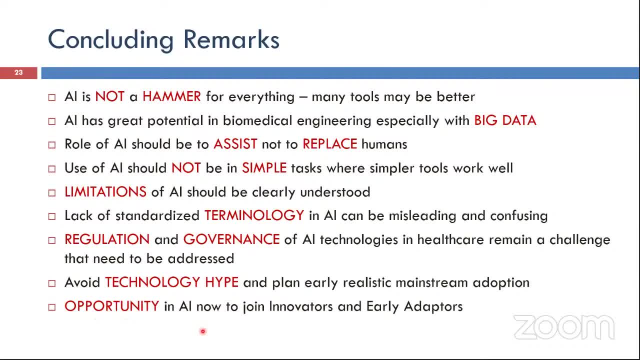 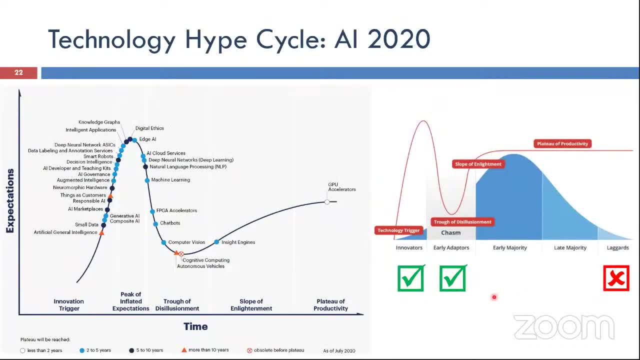 As I told you, opportunities in AI are now to join innovators and early adopters. We are still in the beginning, As you can see. we are still in this area. We still have a chance if we do not do new techniques. 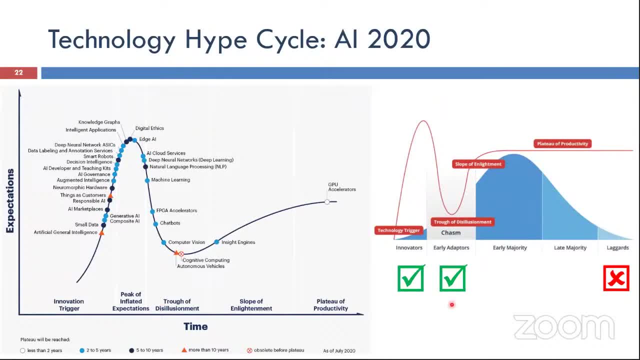 We are still in the area where we talk about early adopters. We can start doing products and go beyond the stage of trough, of disillusionment to understand the limitations and go beyond this stage. You can reach the stage where you understand technology better and, at the end, 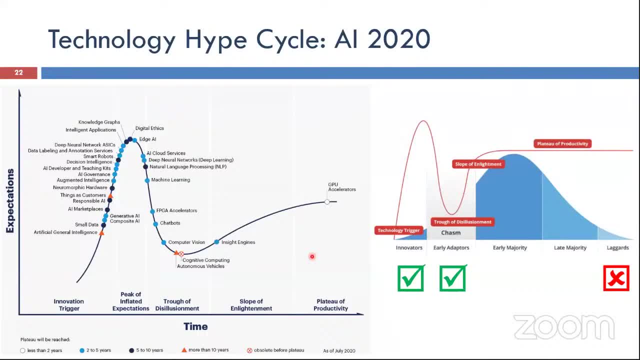 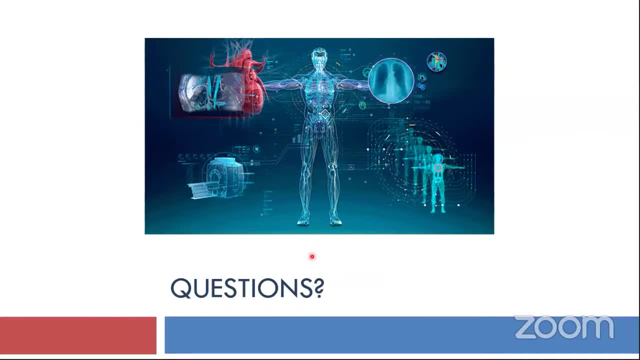 you can make a product that is valuable. We have finished the lecture. I do not know if there was time, but I would like to do a demonstration on how to make a complete AI diagnostic system using MATLAB. Do the organizers have to tell us if there was time or not? 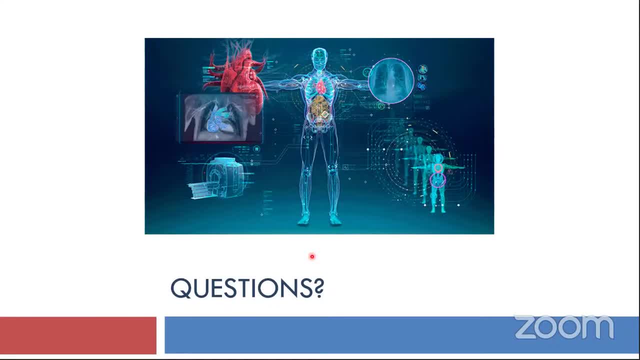 Yes, Doctor, We can do it, But there are still a few questions. I do not know if you would like to answer them or not. No, there is no problem. I do not have a specific problem, But I would like to show you. 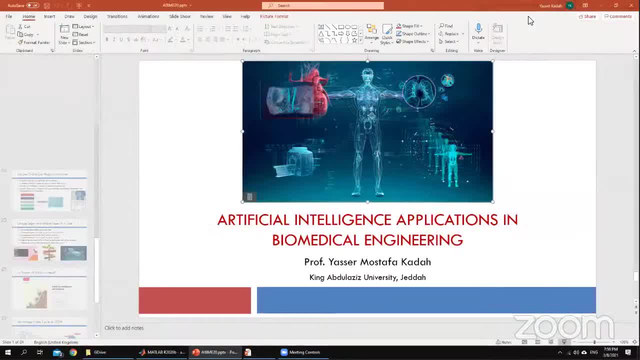 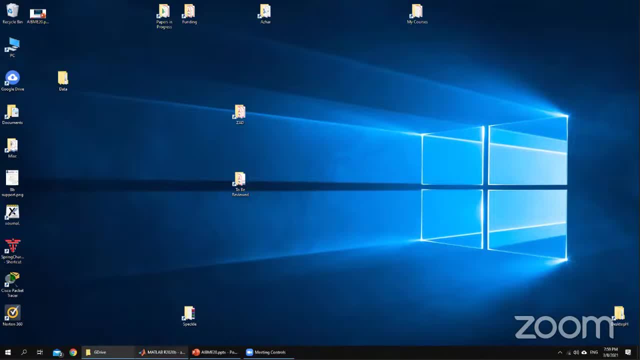 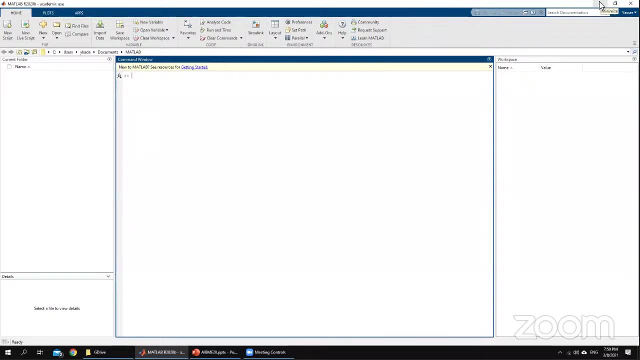 how easy it is. Let me show you how it is. Now I want to do a computer-aided diagnosis for mammography. I have a mammogram for each patient. Can you see the screen? Is there any problem? Sorry, there is no problem. 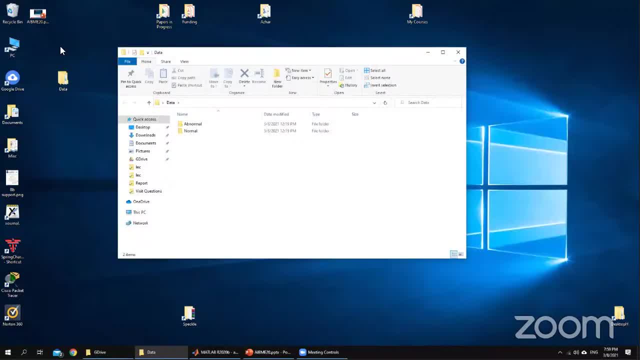 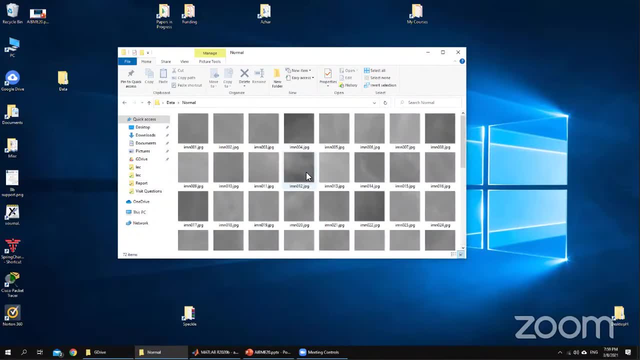 No problem, I have put the data on the desktop. These are normal regions. These are parts of a mammogram. This part is considered normal. I have also put abnormal pictures in another folder. This is from a database which contains the abnormalities, so that I can select. 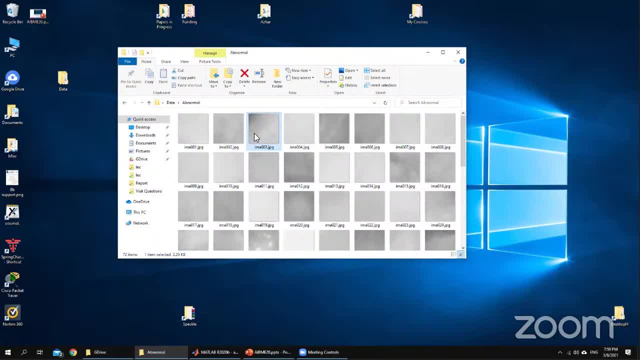 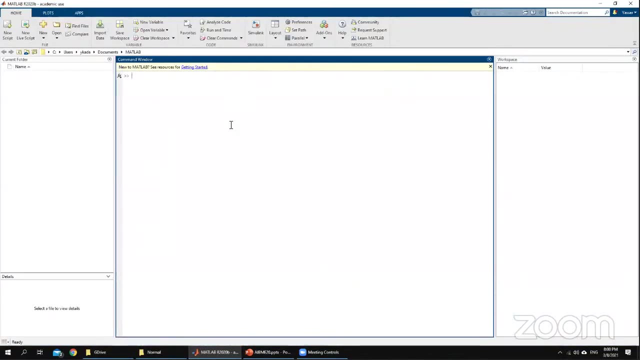 these parts and put them in a database. Here I have 72 pictures of the abnormality. As you can see, I have 72 pictures and the same number of abnormalities. Now I want to go to MATLAB and build a system to do a computer-aided diagnosis. 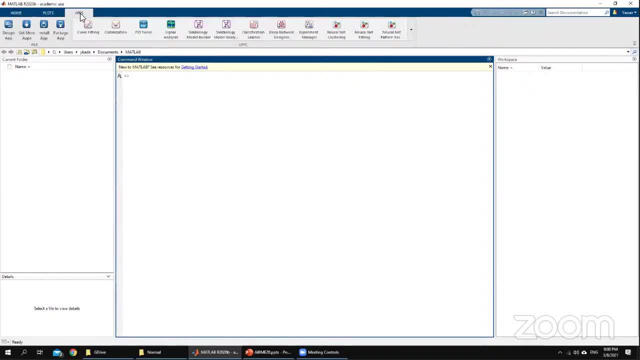 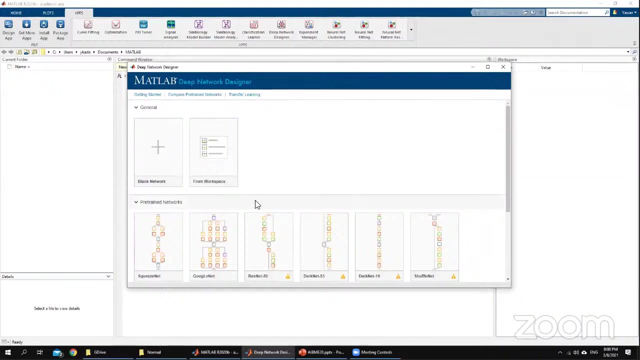 In MATLAB we have apps. If you go to Deep Network Designer, it will open the interface. You will see the networks which are already pre-trained. As we said, we will use pre-training or transfer learning. As you can see, there are pre-trained networks. 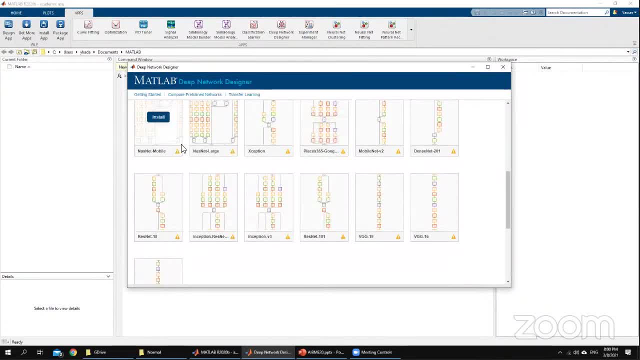 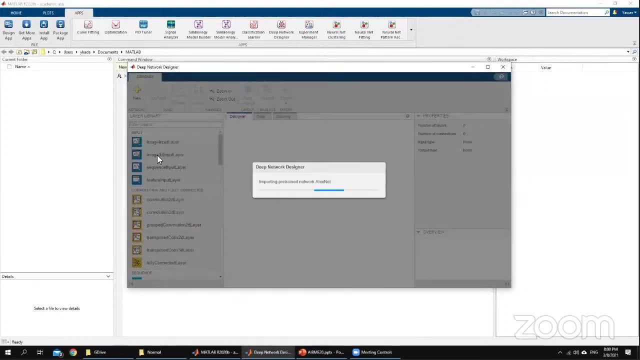 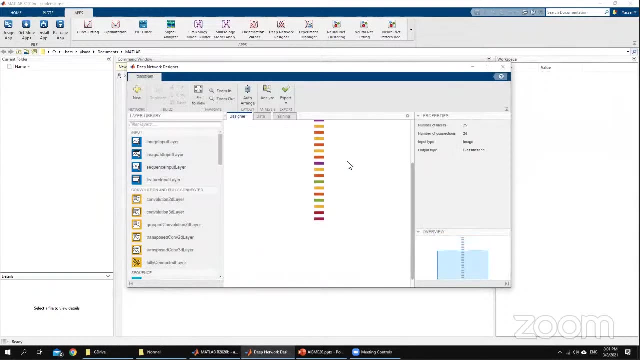 and there are squeeze networks. Let's look at them. As you can see, they are very complex. Let's go to something that looks simple. The AlexNet is one of the things I used before I will open it. This is the network. 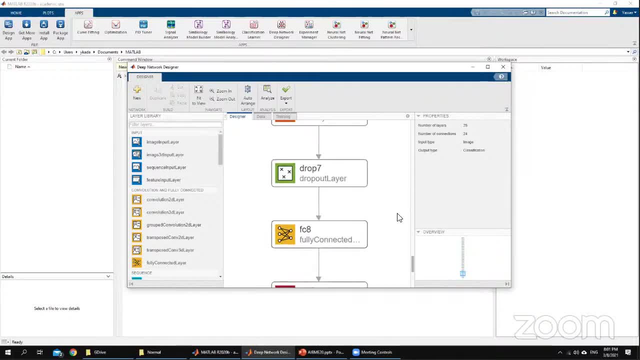 As you can see, there are many parts. It is not clear here, so I will make it bigger. Each of these is a neural network. I want to specify 1000 outputs. The output size is 1000.. Now I want to specify: 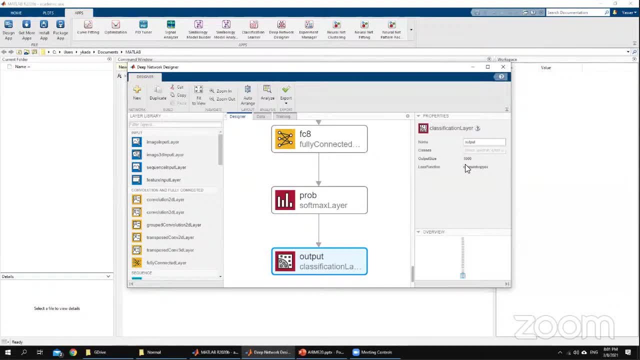 either malignant or benign. I only have 2 outputs. I want to change this. I will notice that the fully connected layer is the last stage of the network before it starts classification. These outputs have a large number. I need to change these, so I will take this block. 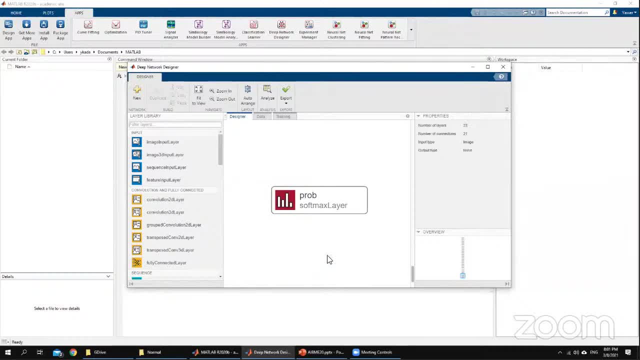 and delete it. I will take this block and delete it. Now I want to see the fully connected layer. I will drag and drop it and put it here. I will connect it to DPD. I connected it to DPD. I connected it to the first layer. 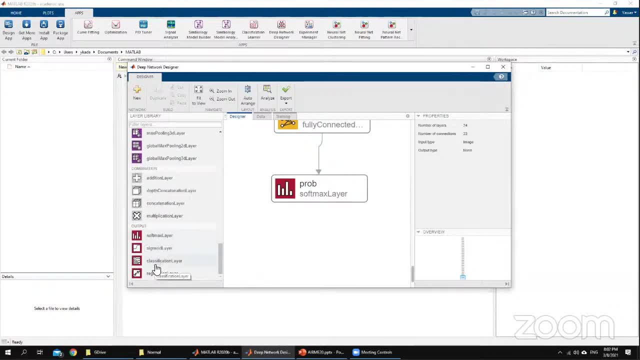 I need to put another layer to do the classification. The output layer I had, I will put it here. I will make sure to change the output size. I will make it 2.. I will make it 2.. Now it is 2.. 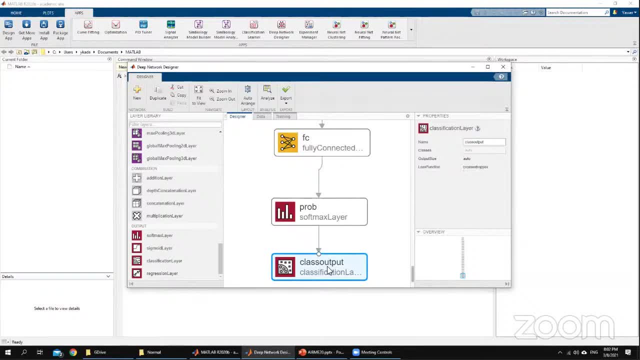 The class output is automatic. What comes out of here comes out of here. The output that comes out of here is softmax. It is like thresholding: If it is higher than one, it gives 0. The network is better for me. 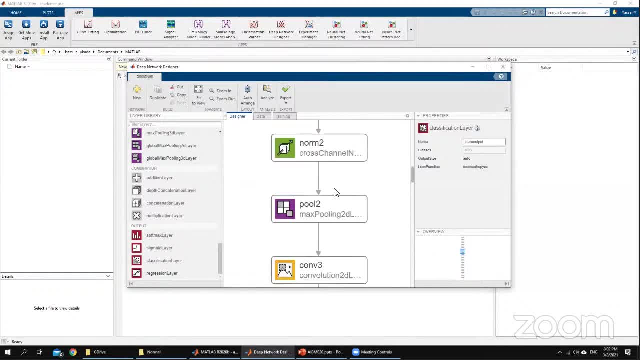 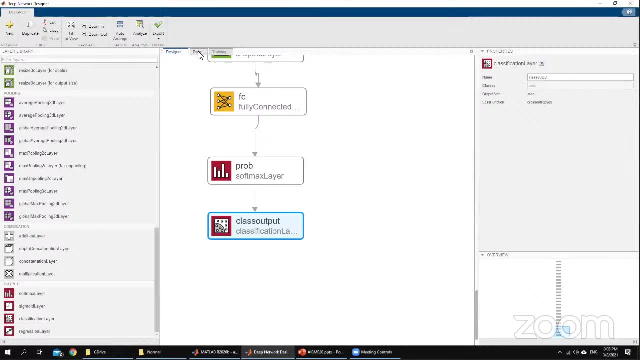 As you can see, there are many layers. There are many layers. I will make all of them the same. I will not change them. I will train the networks only. I will go here. There is a data option. There is a tab for data. 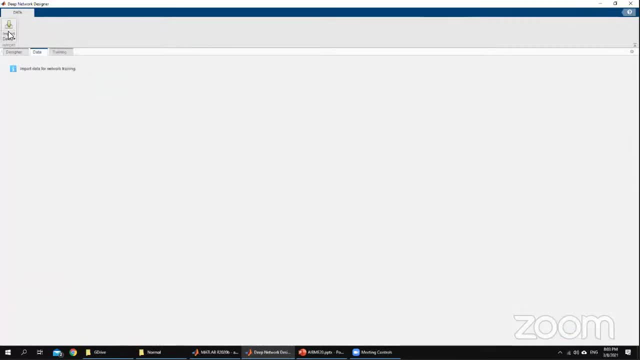 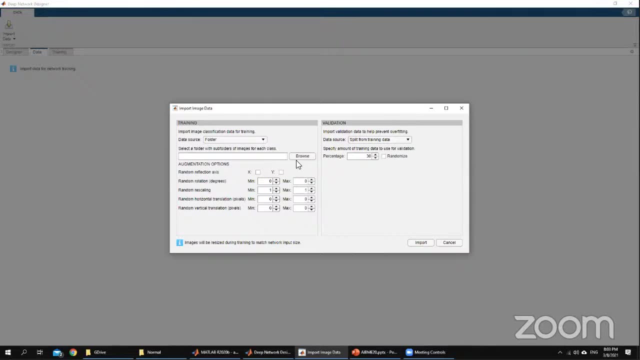 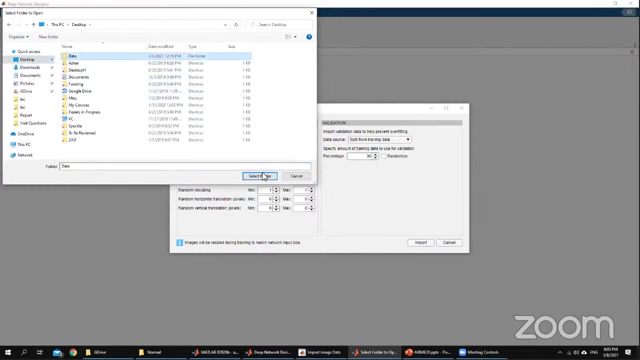 Here it says import data for network training. I will go to import Import image data. Here I chose a folder. I will do browsing. I will go to desktop Data. I will choose only the external folder. By the way, it will take this folder. 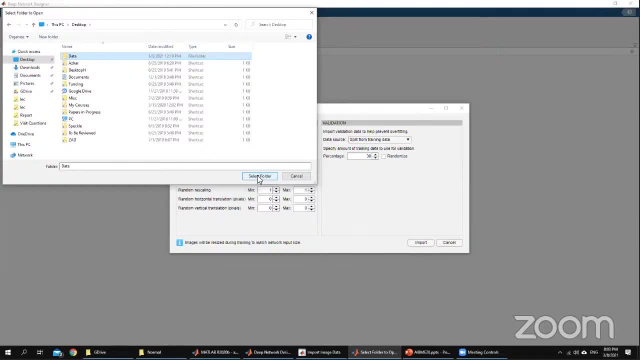 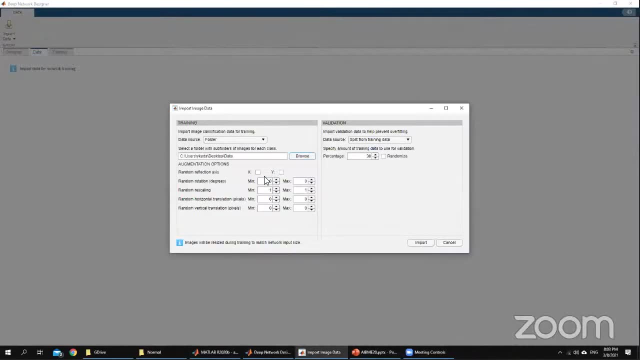 and see the subfolders. Usually subfolders create classes. As I have two, normal and abnormal, It means it will see only two classes. If I have more, it will see more. Here I need validation. Validation data is important in training. 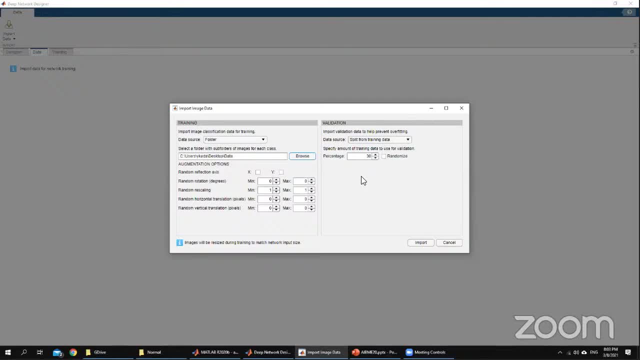 like homework for students. Basically, we train with some data and do validation to see if we have learned or not. Therefore, here my choice is to leave 70% for training and 30% for validation. I took the default and leave it as it is. 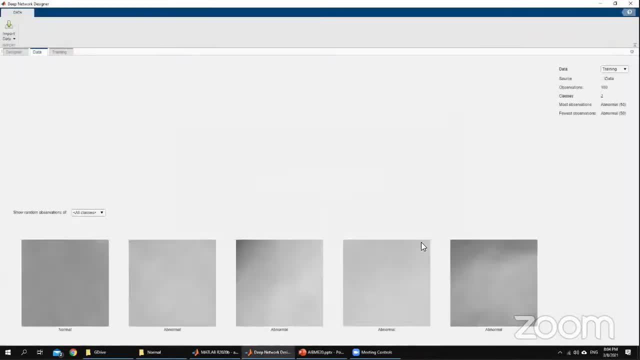 I will import. As you can see, you have 50% of your data and 50% of this data You have examples of the existing images. We want to do training. Let's go to training. Training can work as it is. 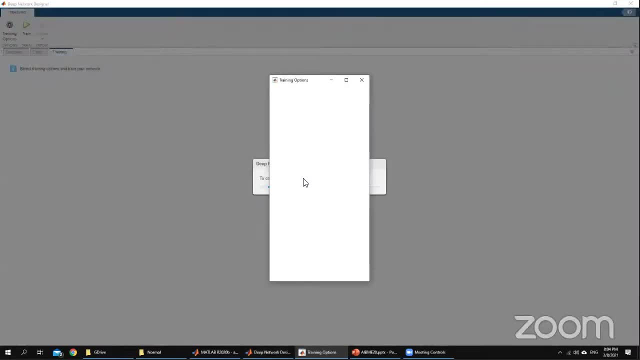 but it is better to look at training options. I always prefer training options in the initial learning rate to be a little smaller, because when it is large it will skip the correct solution. Let's make this validation frequency a little higher. Let's put some numbers. 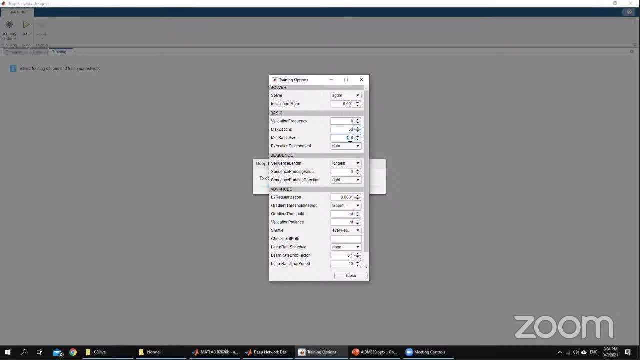 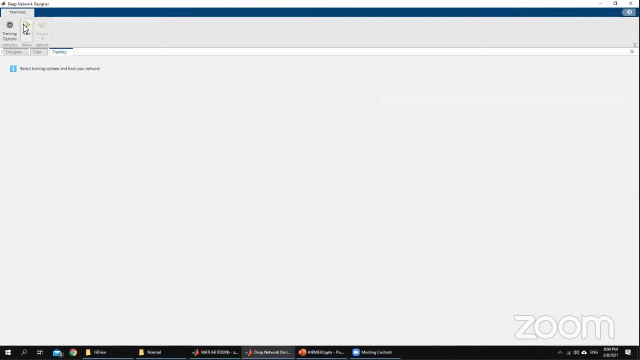 After you have some experience in training, when you have tried several parameters, if you did not find a good solution, you can repeat the experiment with another solution with a different set of parameters. I will take a set of parameters that seems to be okay. 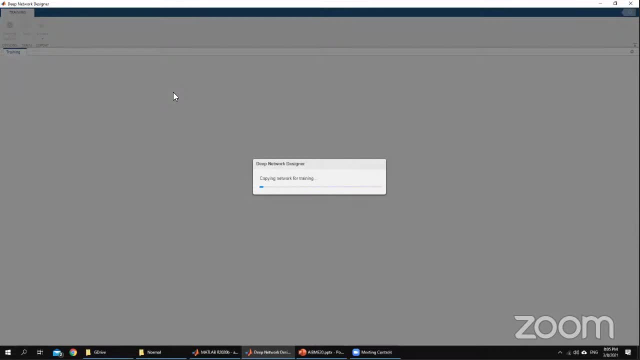 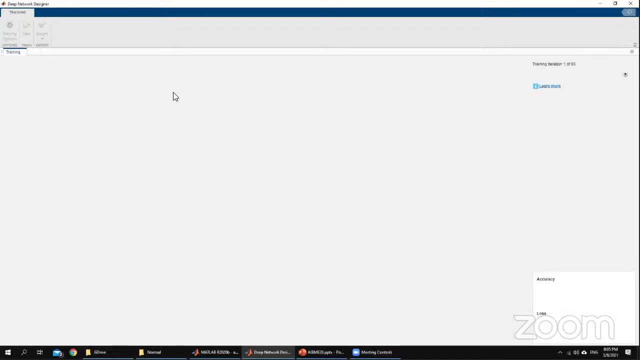 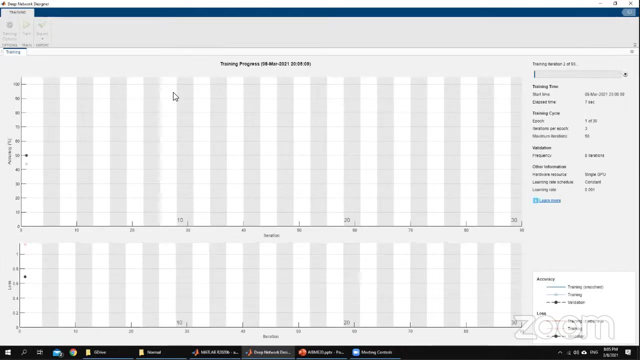 and do training. What is important now is that in validation data, it learns from training data, and when it comes to solving problems, it gives me a percentage of almost 100%. This is the goal: When you learn something, it proves that you learned it well. 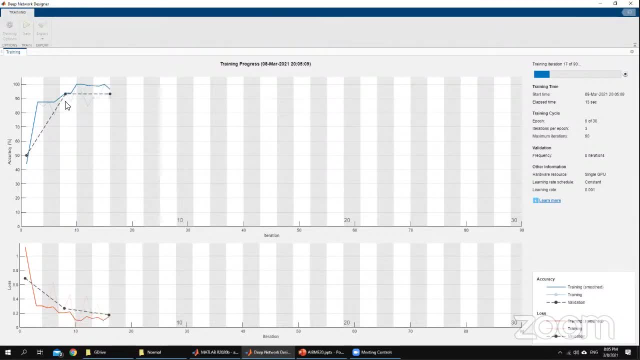 and that you got a good level in homework. The first one starts from 50% and then it goes up. The validation is the dash line and the continuous line is training. It is the progress with training. It is doing training. now I made the training. 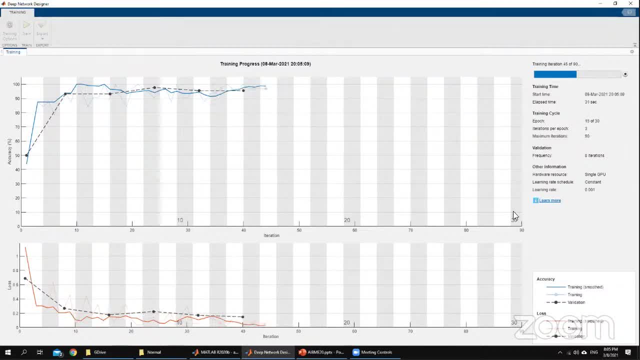 to be considered to some extent, because in the end I do not want the time to be long, But if we talk about a large dataset, this training can take a long time. I also did training on the GPU, so it takes a little less time. 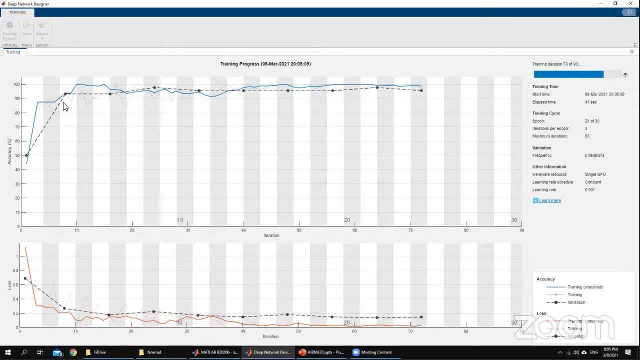 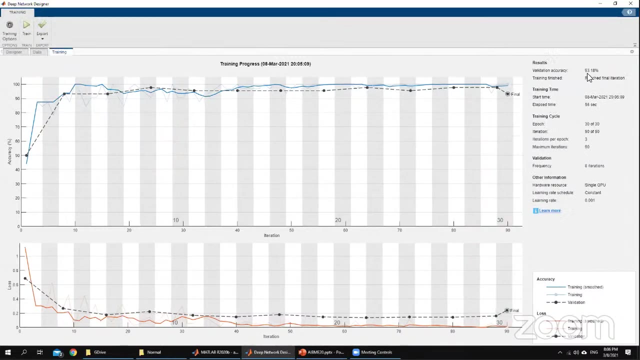 As you can see, the accuracy starts to get closer to 100% in the training and for validation it starts to be more than 90%. This is how it finishes. This is how it actually finishes. The final accuracy was 93.18%. 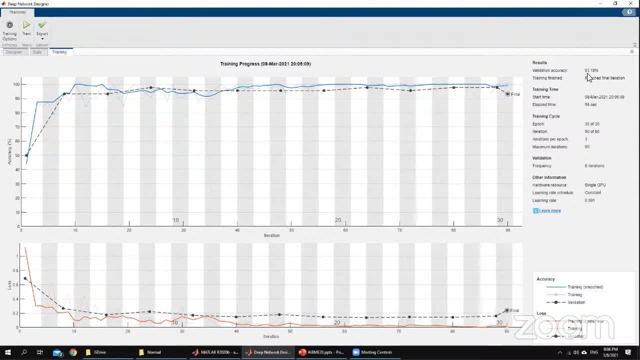 93%. Now we have built a computer-aided diagnostic system for mammography in less than 5 minutes. You can imagine the ease of the tools available for these techniques. The problem is not that you find a tool and use it. 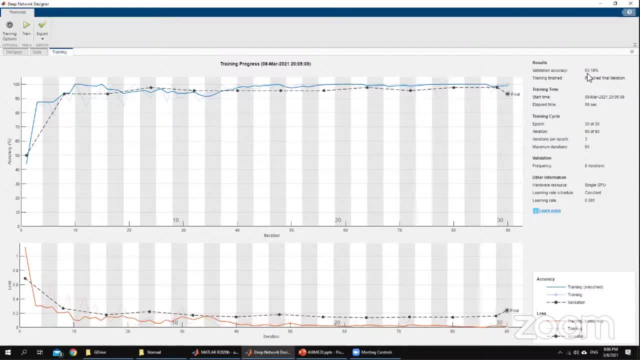 The problem is that you have to think about whether this validation is really accurate. In order to take the final exam. you have to test your system with data you have never seen before. You have to see if it really knows how to interact with it. 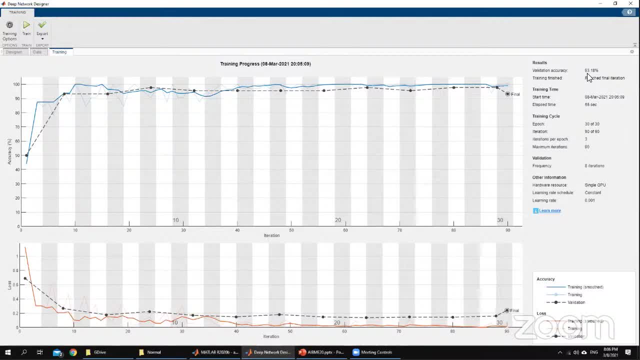 In the end, even if it did a good job in testing, you still do not know what this network contains. There may be data in the future that gives you illogical results. If you follow the topic of self-driving cars, you will find that 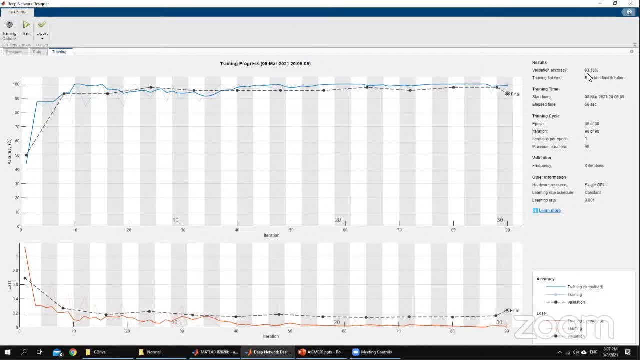 it is a freak accident. It is a very strange accident. People do not know how to drive a car. They do not know how to drive a car Despite the training and everything. there are still some places where, when the data comes in a certain way, 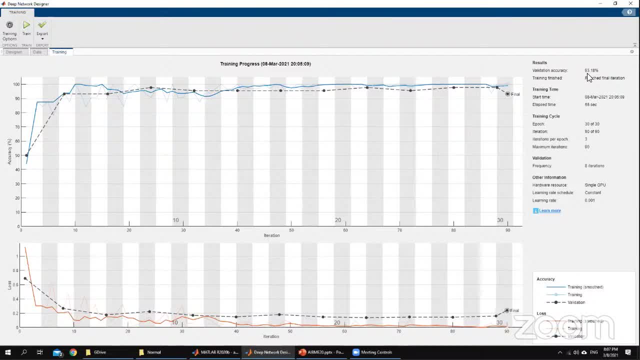 you find that the output is something you do not expect. This is just a simple thing. For those of you who want to try and need this data, please send me an email and I will send you this data to be trained with. The most important thing is to make you learn. 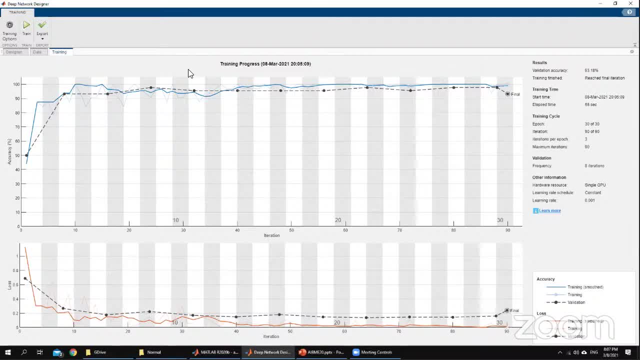 how to drive a car. It is not a matter of working with your own hands. You can listen to a theory lecture and see a few pictures that look nice. You may be happy that you got this information, but you will probably forget it tomorrow. 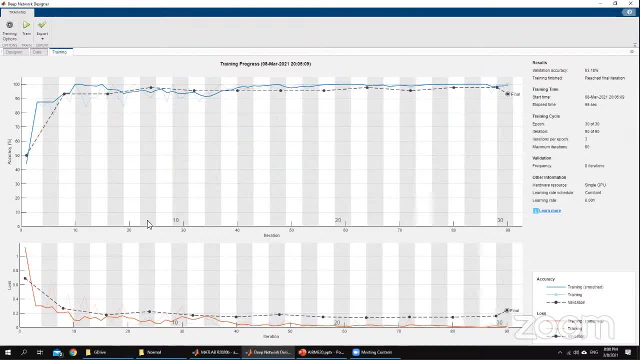 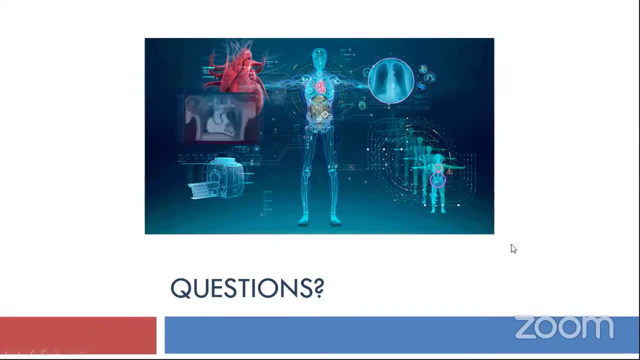 If you worked with your own hands and tried it, you will find that this information is very consistent with you. If you have any questions, you are welcome. Before we move on to questions, I would like to point out that we sent a link to the Zoom chat. 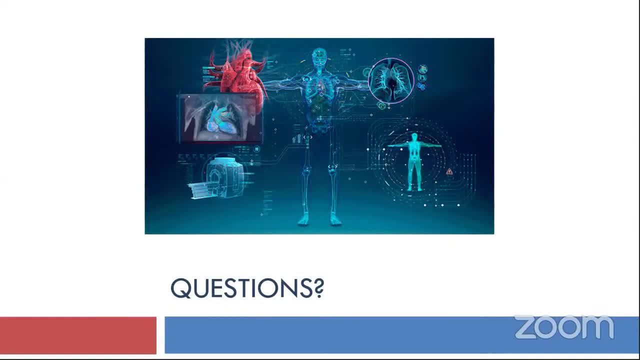 and the YouTube chat for the students who are traveling from Yemen to Mecca. We will receive the questions, whether it is on YouTube or Zoom. If you have any questions, please send your questions to the Zoom chat. We will be happy to answer them. 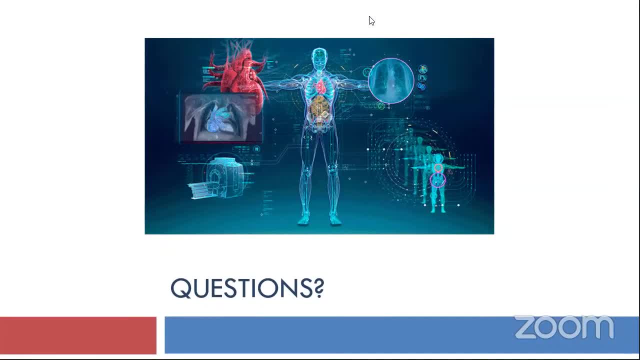 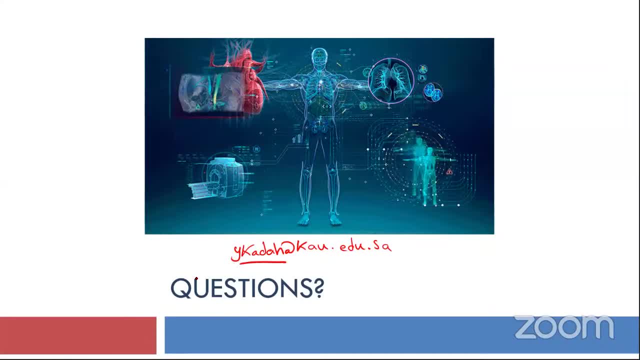 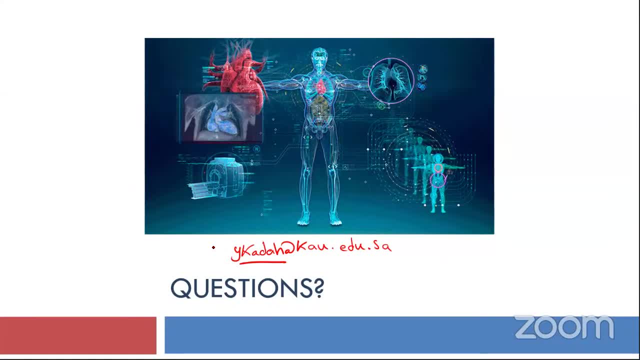 where do I start, doctor? From deep learning or do we start from AI in general? No, deep learning is: if you start from theory, it will take a very long time and you will get lost before you get there. Okay, 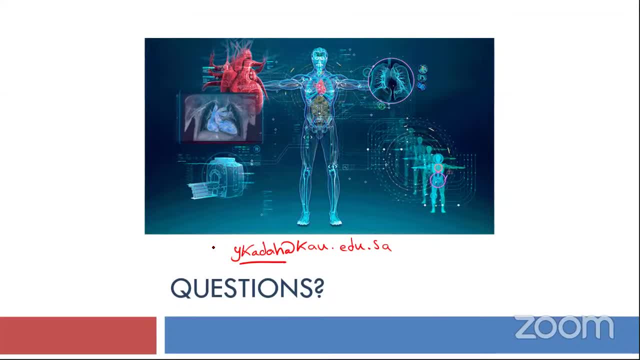 I advise you to walk in parallel. okay, Meaning try, and you will know the theory. You will realize that the two will help each other. Okay, When you try, you will have the experience of the experiments and you will know the parameters. 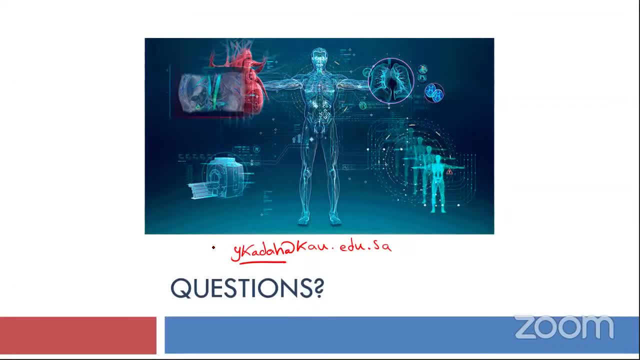 meaning, what are they, and all these things. And at the same time, when you read the theory, it will not be very abstract. as a result, you really saw in the end how the system worked. So I advise you to walk in parallel. 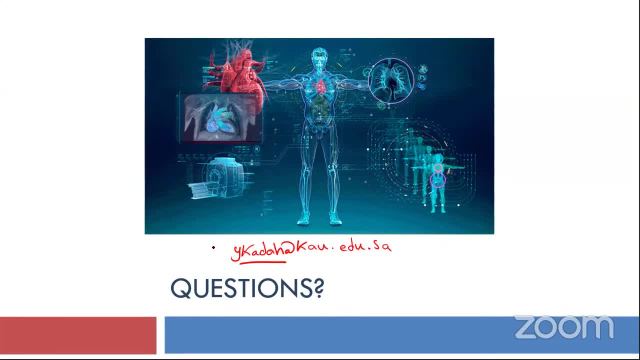 And, by the way, there are many examples, whether it was in the MATLAB itself, you will find examples on, for example, deep learning, which has to do with the image net, for example, which is, as I told you, the database. 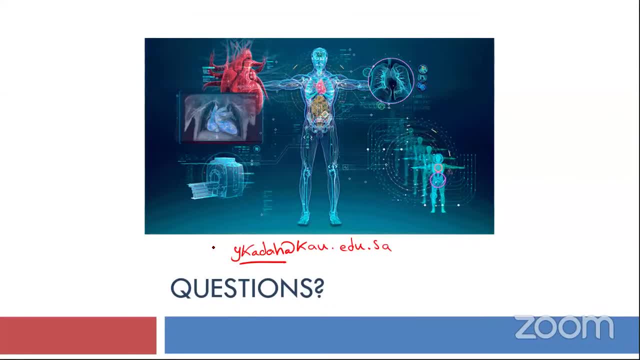 which has photos of all kinds And, as I said, if you learned on any database, you can take the information itself and you will have the deep learning and you can take this application for the biomedical application. So you don't have to work. 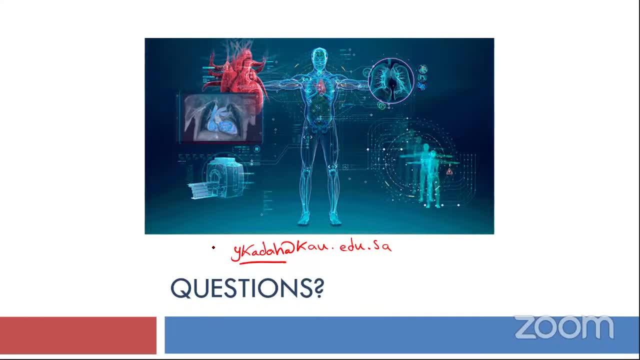 on the biomedical applications from the beginning. You can look for the data that is available and work on it, and then the experience you have taken, you can apply it to the application. Of course, guys, the slides that the professor gave me: 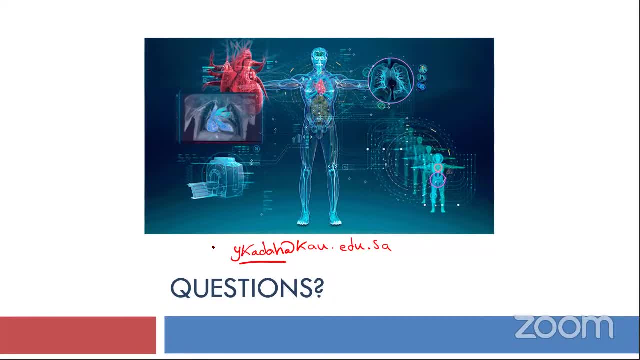 I hope we will put it in the Twitter account and the lecture will be recorded. There is also a question from Abdullah: Which is the best specialty to be closer to computer science? Which is the best specialty to be closer to AI, Computer science or computer engineering? 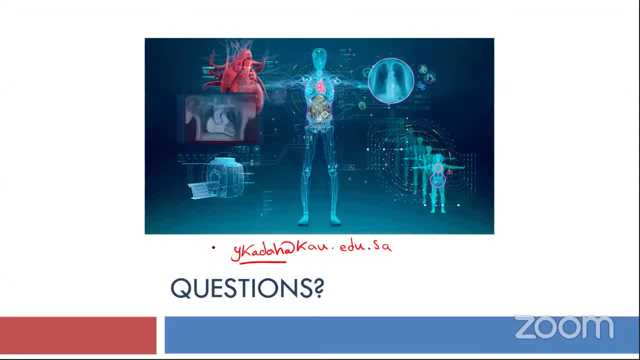 I think that's what he means, In my personal opinion, this or that. If you were imagining deep learning, in order to understand it, well, you would need an optimization theory. Okay, This optimization theory, you will find it. it can be used in communications. 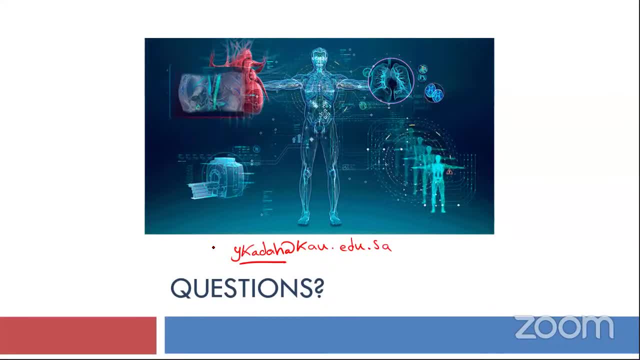 you will find it in computer science and computer engineering. They have a relationship with it and everything else. but other specialties can be used in it in a big way. There is another part, if you understand the physiology of the brain, the physiology of the neural system, 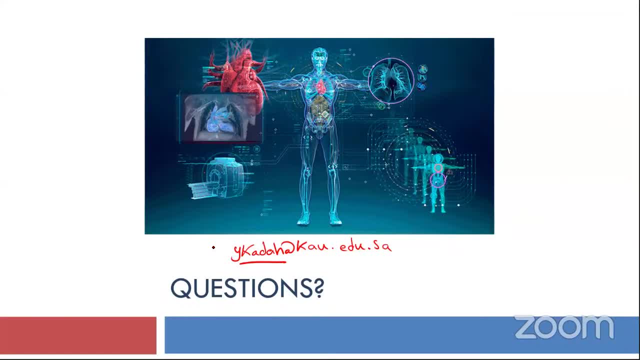 you can actually work in deep learning. if you were building new circles, you were building, you were building networks. no one had done it before and you tried it. The real advantage of deep learning and the advantage of the existing platforms. 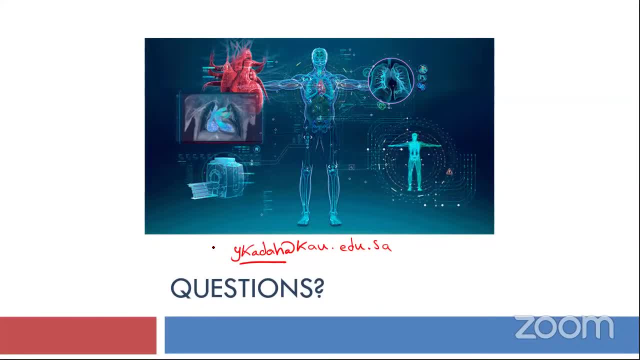 is that it allows you to enter your specialty. you can find something to do in deep learning, Okay, In other words, something that you are not very specialized in. you can take what the specialists did in this part and continue it in a part that has a relationship with your specialty. 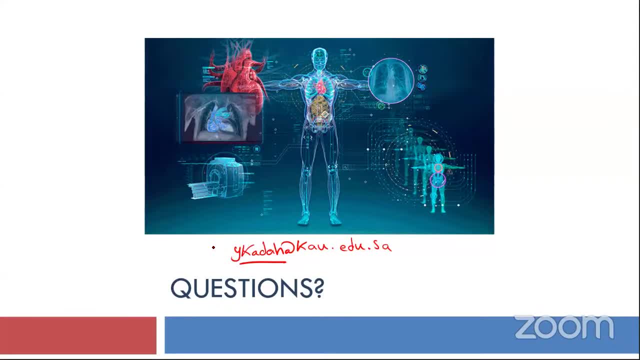 Okay, For example, if you are a biomedical engineer and you don't have anything, you don't have anything. you don't have anything special in the computer. you can work on the part of data, that you prepare the data in a way that allows learning to be done effectively. 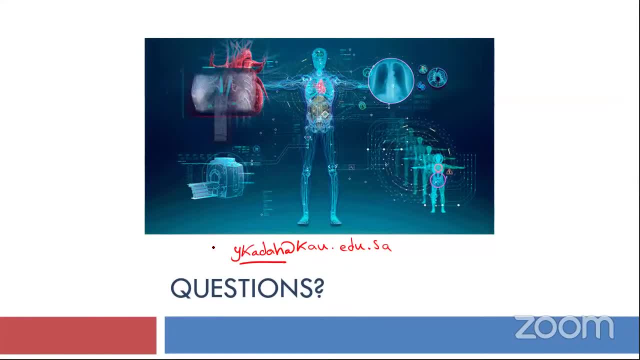 And this is actually a lot of work as a result, because there are some techniques at the moment that have nothing to do with how you do the augmentation of the data, how you increase the data set. you have a number of points or a number of limited pictures. 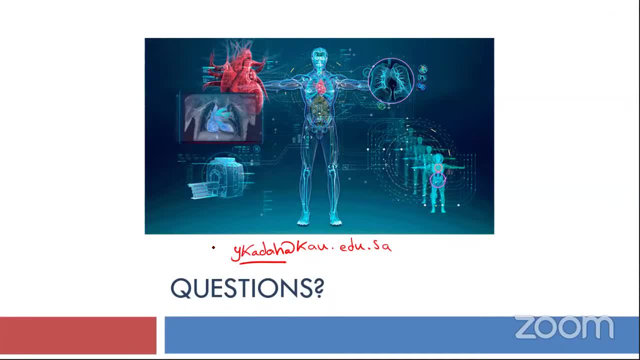 how you increase the number of that, how you do the simulation of new pictures from the existing pictures. Okay, So there are techniques that have nothing to do with us. we are the only ones. no one else can do it other than us. 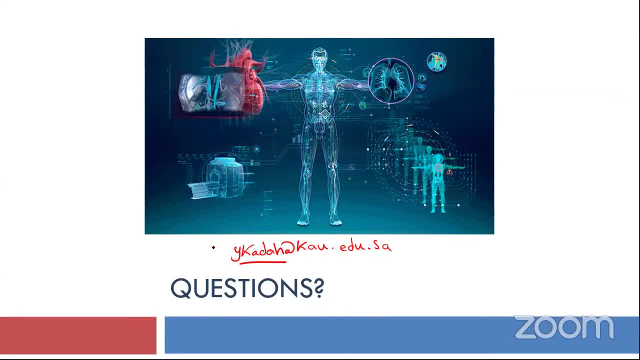 So I mean, in my opinion, you don't have to have a specific specialty. you consider deep learning as a multidisciplinary field. you can enter it, as others can enter it, and you all make a contribution in the field. Prof. there is a question from Mubarak. 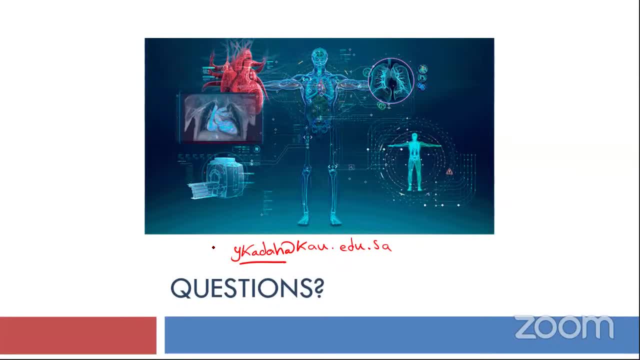 he says, in the medical field it is not possible. if there are errors, how can AI rely on the possibility that doctors can discover it? Honestly, the question is confused because there is Arabic and English. so if Mubarak can raise your hand and say the question, it will be clearer. 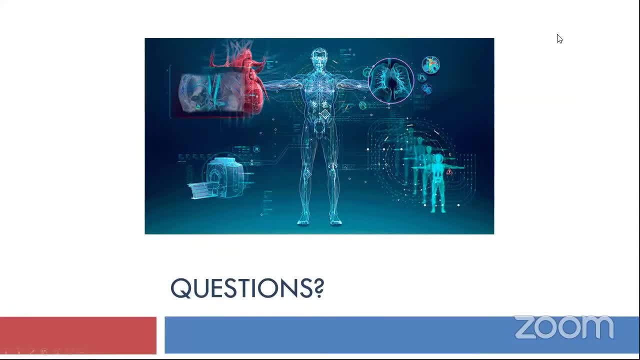 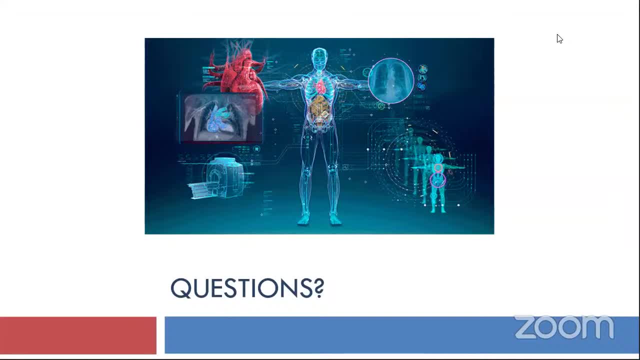 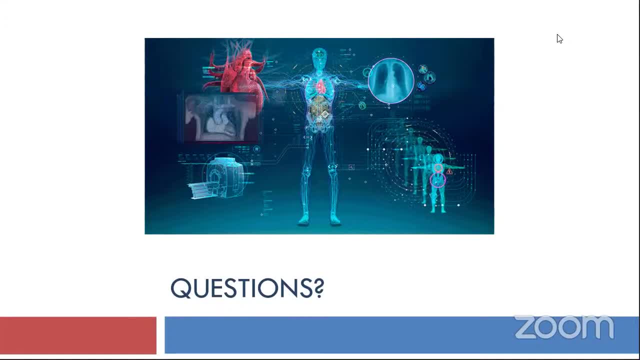 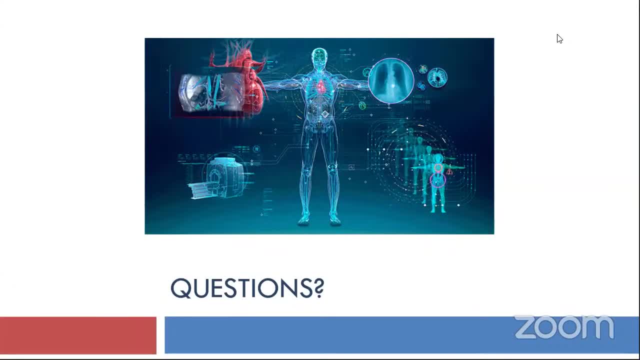 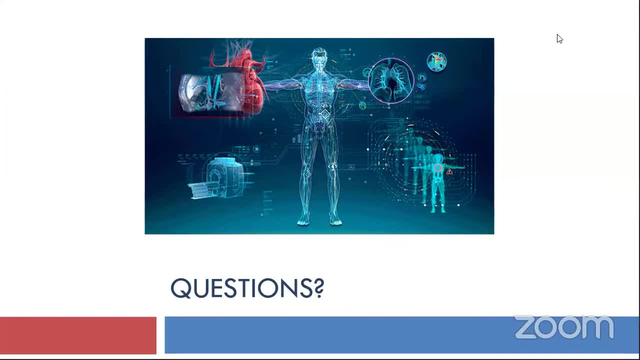 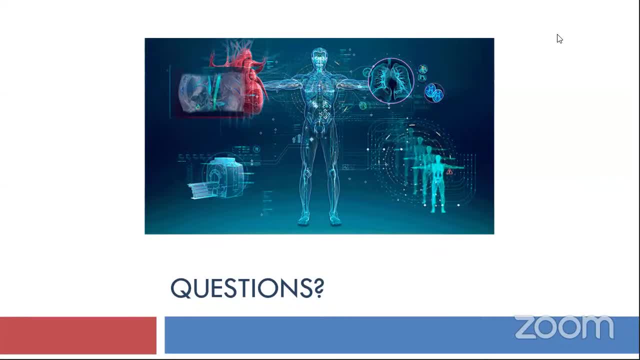 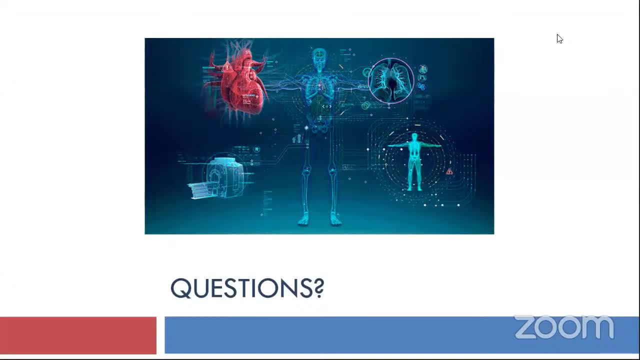 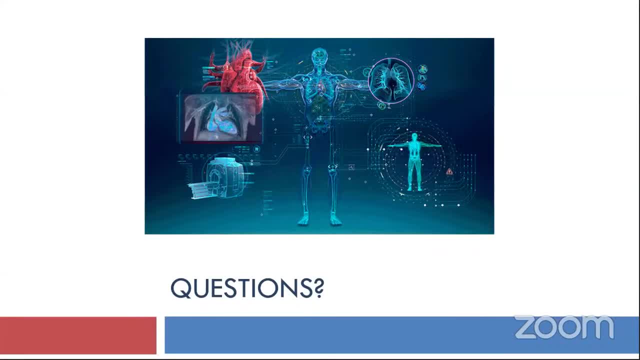 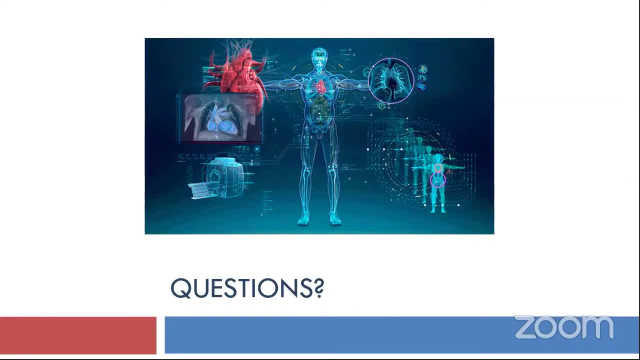 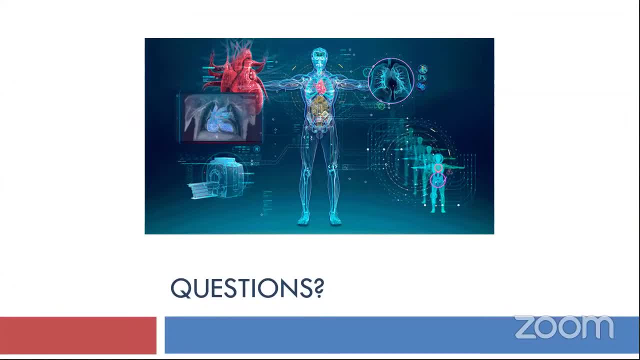 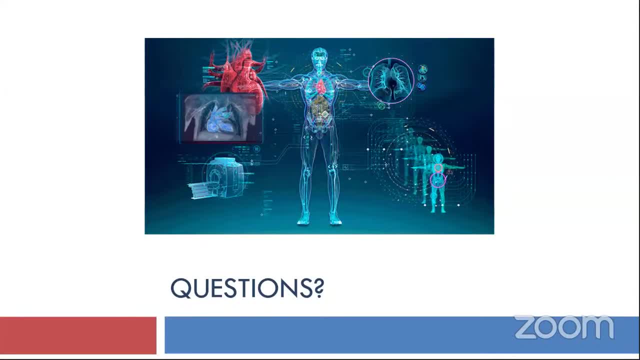 he does not know the type of features that are supposed to be created. he can use the features that he sees that may be useful or have something to do with the diagnosis that he wants to make. So there really are no features. Features are present within the network. 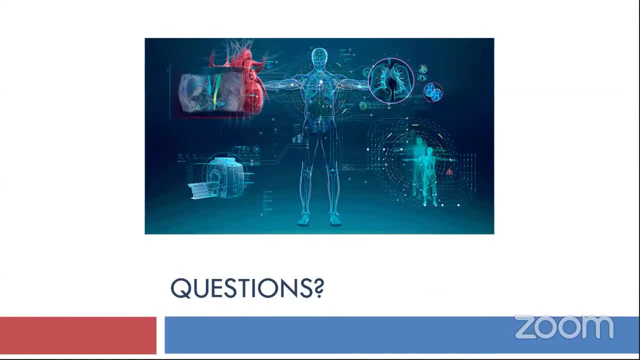 He will learn them by himself and in the end, he will use them without knowing anything. So if you tell me what features he has that depend on him to make his decision, it is basically embedded within the million parameters that you heard about. Therefore, one of the problems of neural networks is that you do not understand. 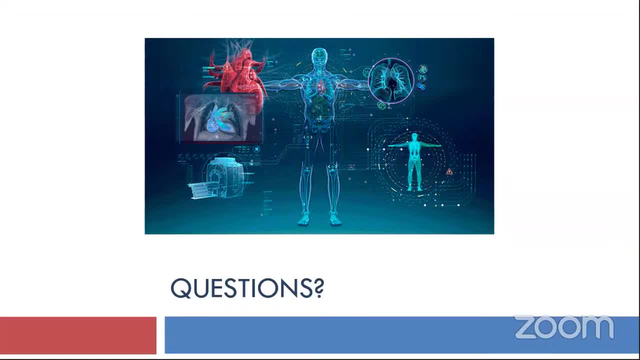 you cannot explain why the output is like this. you cannot say why it is malignant or why it is benign. This is one of the problems in the regulation of medical devices. When you say that this patient is malignant, you have to say why. 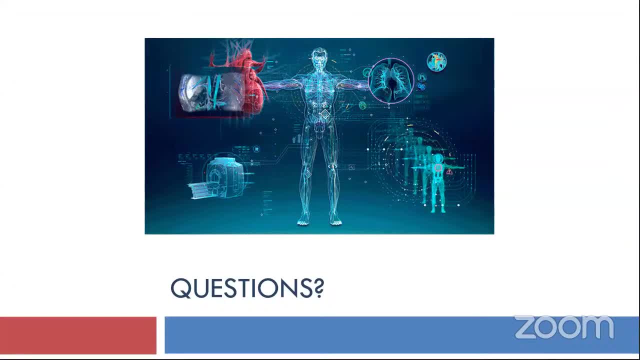 We cannot do this now, even now because of deep learning. These are some of the problems that are present as a result of us not being able to explain why the output is like this. Doctor, there are two questions here about the sources or the site that you took the data from. 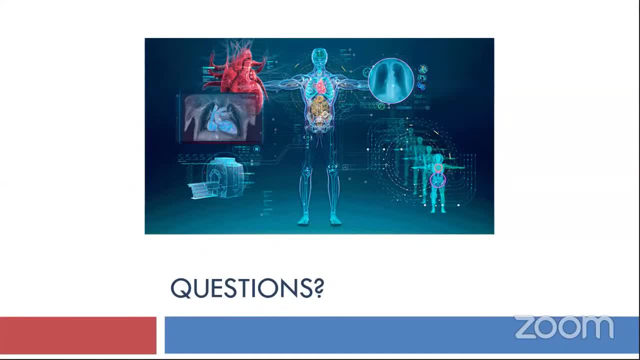 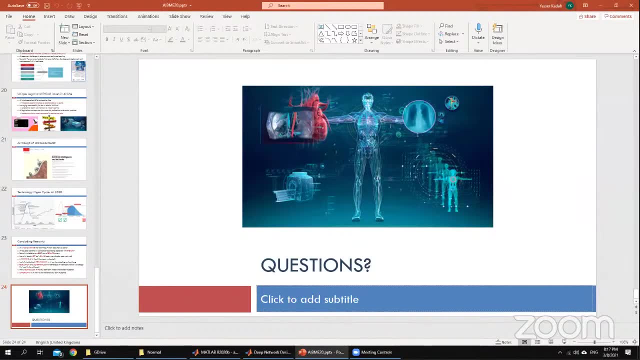 for those who want to train on it. Okay, If you looked at the data on the internet, let us look at it now. I will show it to you now, in front of you. Now I will just open it like this. I will just click on many mice. 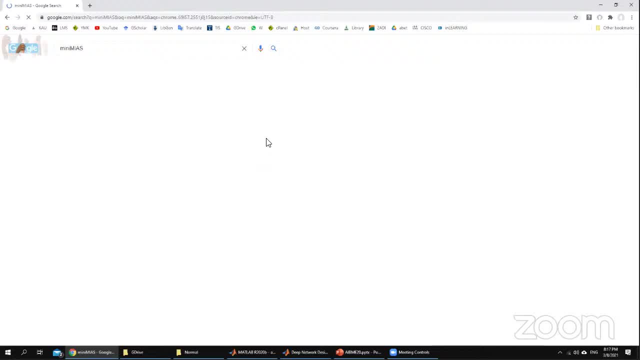 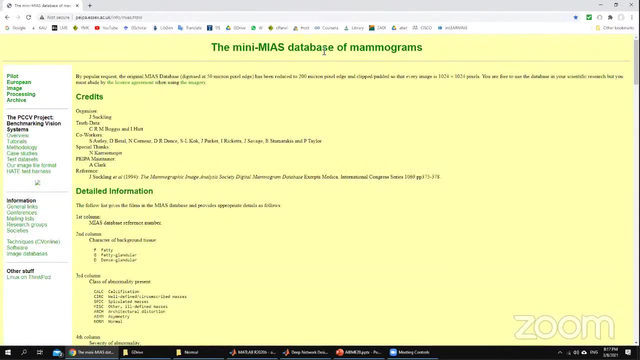 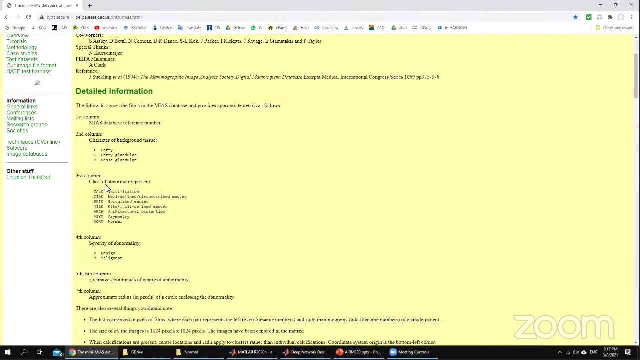 Many mice. That's it, Okay. You will find here the many mice database of mammograms. Open it, Okay. Here you will find all the information that you need Here. it tells you how the data came. it tells you the class of abnormality. 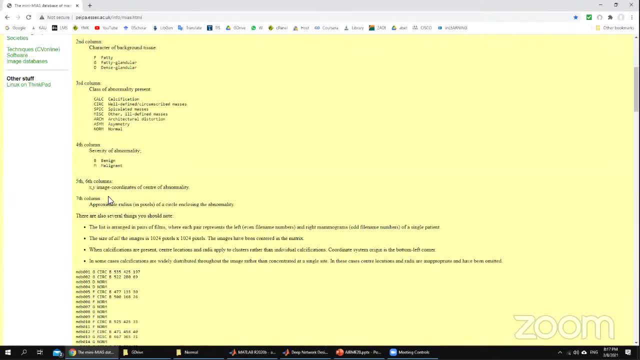 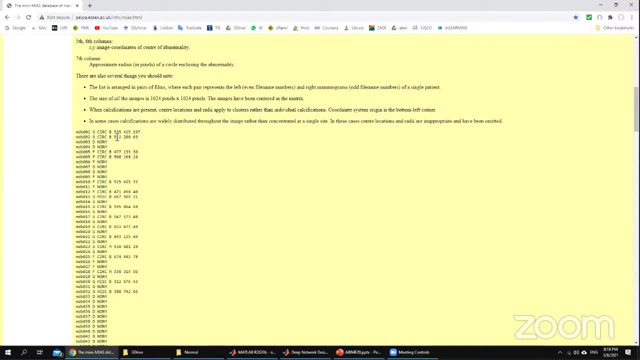 it gives you the classification of benign and malignant, and then it gives you the picture itself. each one of these is called a picture. It tells you what kind of picture this is and it tells you if it has malignancy. it tells you that the malignancy center is this and that. 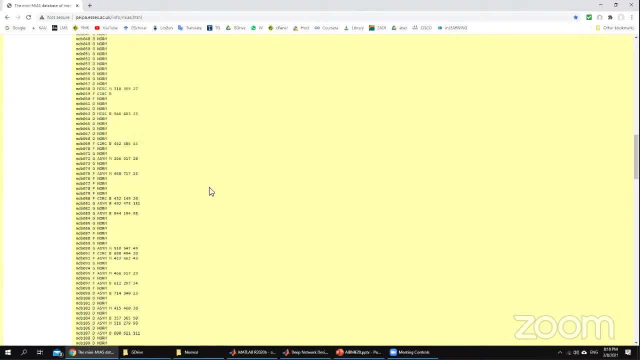 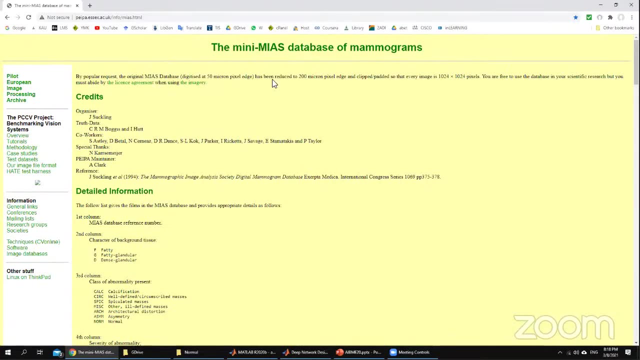 and the radius is this, So you know the circle that the disease is in, so you can take samples from it, which I have shown you now, So you can download the complete dataset from this site open. okay, one of the things that is open. 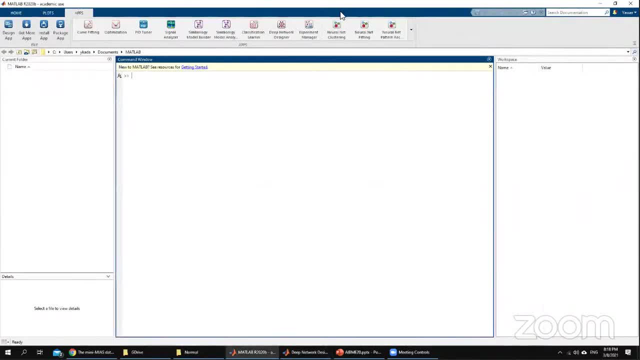 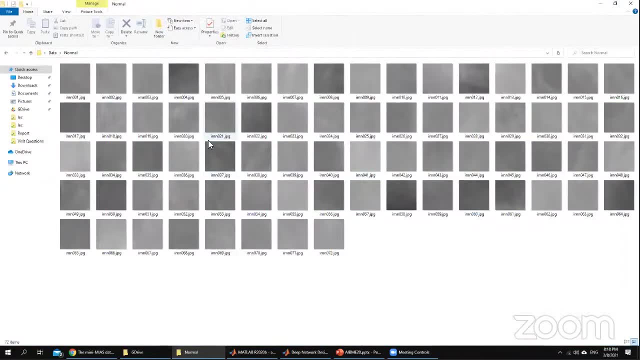 or you can ask me or send me an email. I will give you the data itself, which I have shown you now. So I took the pictures. basically, as you can see, I took the places that are in the abnormal regions. 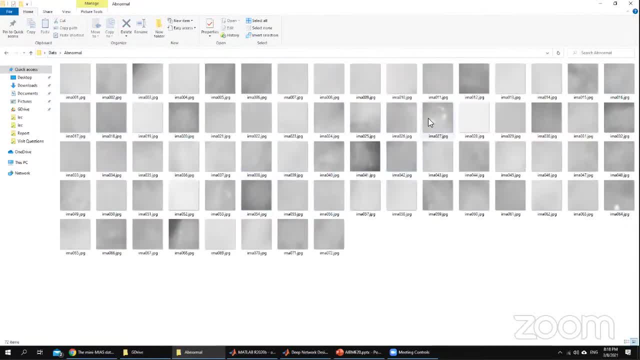 for example. let me show you the abnormal, because there are things that look like you can see. for example, there is micro-calcification. This can look like a big area, but this picture, which is 32 by 32,, 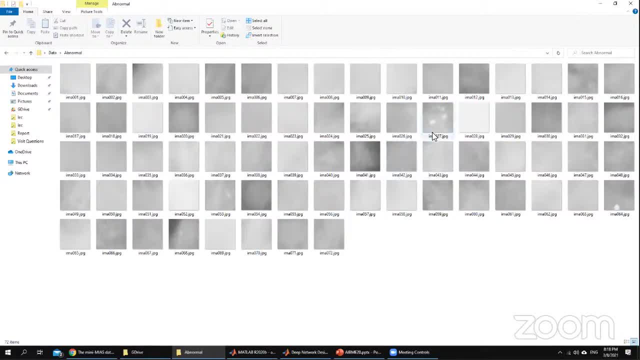 the picture is 1024 by 1024. So the picture this is a very small part of the picture, Okay, So basically we are talking about that. I just used the information that is in the site to take the regions that represent the existing abnormality. 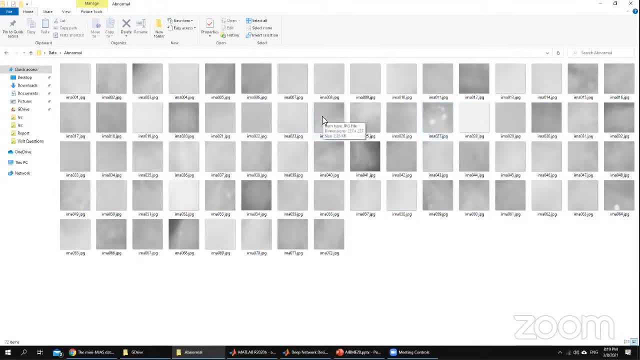 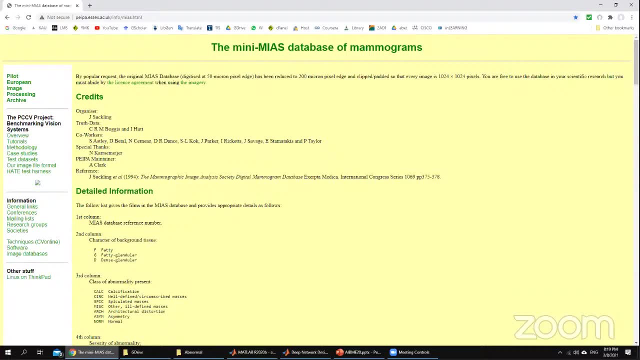 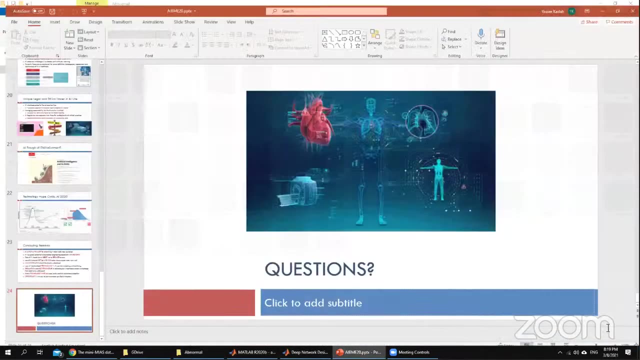 because I need to have a database of the normals and abnormals and use it in training. So it is already present in this site, so you can go back to it and you can download the complete dataset from it. There is a question here. 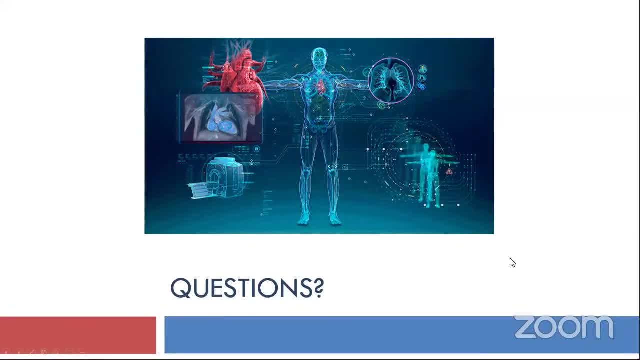 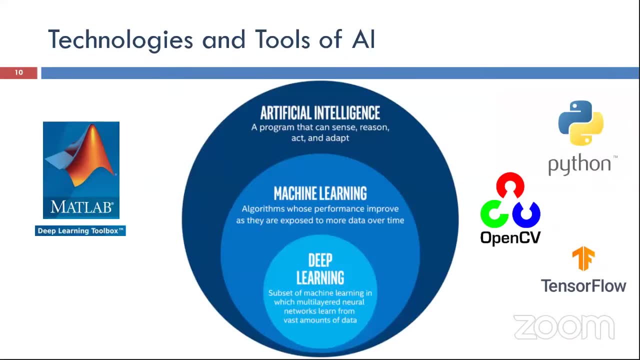 Doctor about the best software or any software. to start with the beginners, I advised you two things. I mean we have people who want to use the paid thing which is available. we have MATLAB with the deep learning toolbox If you are a little trained in software. 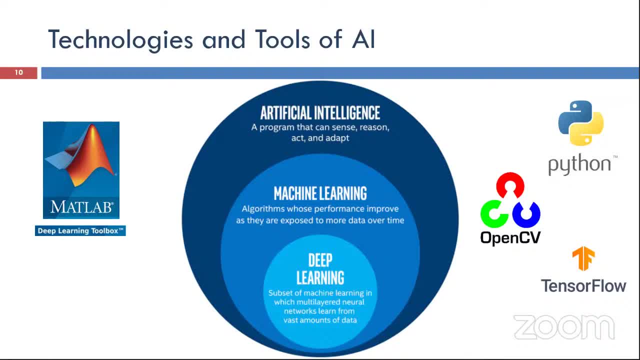 you can enter Python. you can enter things like TensorFlow. these are the things that are open source. Okay, You will always find the feature of open source that you have a slightly large community- Okay, So you will find a lot of applications. 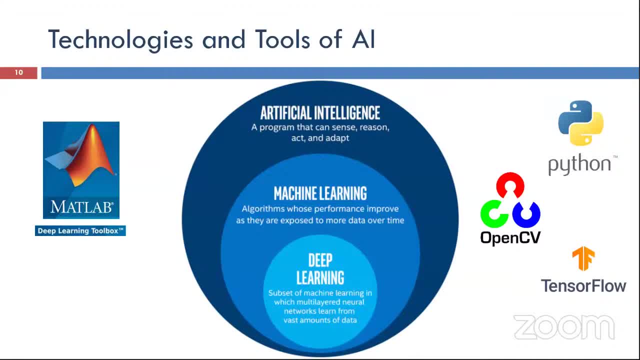 that you can use MATLAB. you only have MATLAB itself. I mean the MATLAB thing, as long as you have it. this is what is available to you If you want to start the simplest for you. as you have seen, 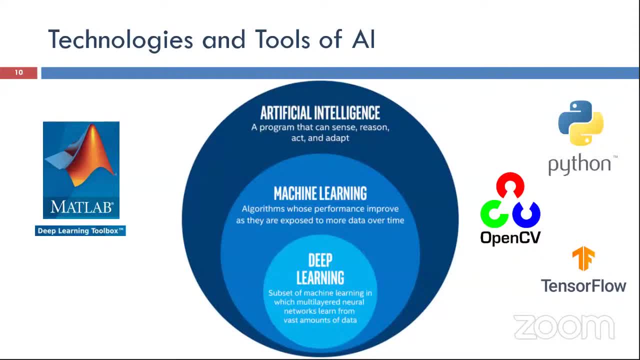 we have done it in the demo. we have done it in MATLAB. Okay, You have an app in MATLAB in a simple area. You can use it in a simple area so you can get data very quickly. Okay, But is it the method of choice? 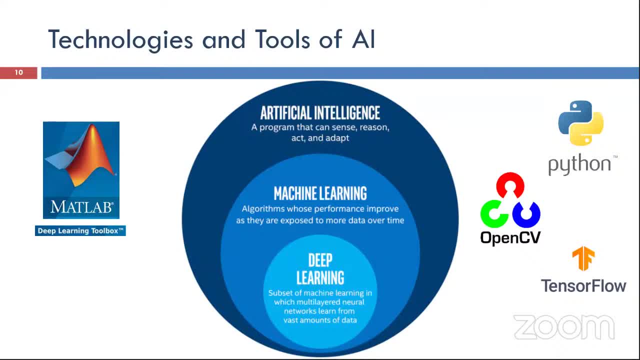 I mean depending. I mean it can have words, Okay. I mean, if you want to find something- for example there is a demo or there are examples- when you walk on it you will find that it is really excellent. 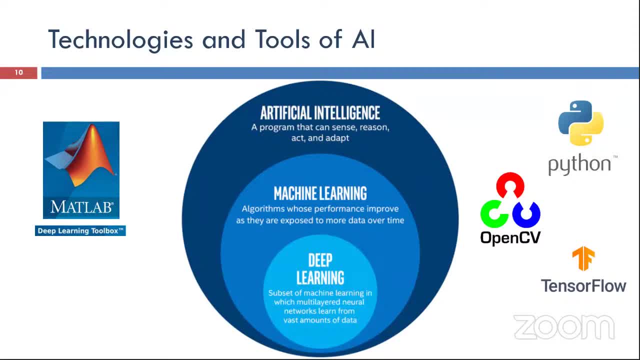 There is a question from Ahmed. he says, who specializes in medical engineering and he will continue his master's degree in AI. What do you think, as a professor, according to your academic experience? In fact, I have an opinion about AI. 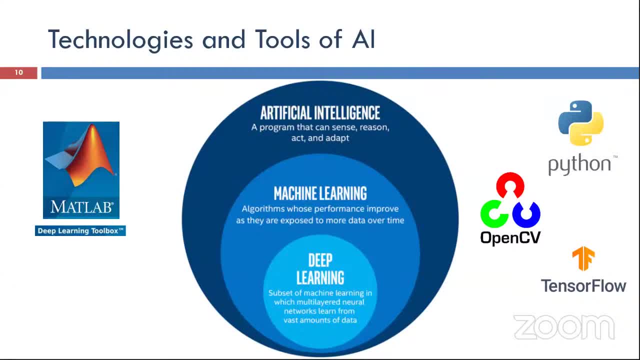 In fact, it is not possible to study AI from the beginning. I mean, there are people who talk about Baccalaureate AI. Okay, AI is a tool. It is a tool. It is a tool. Okay, After finishing biomedical engineering. 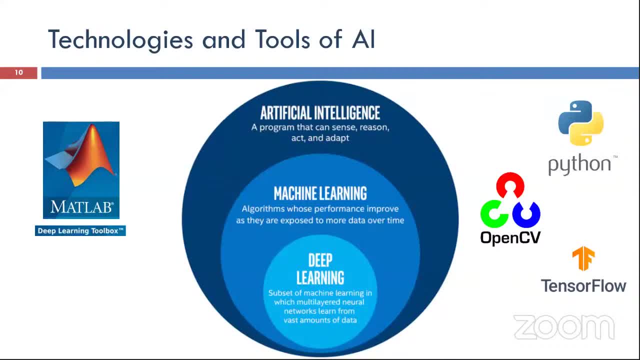 you have a background, You have problems in biomedical engineering. you look for a tool to solve them. It is very good that you go to do a master's degree in artificial intelligence, But now, if you want to do a Baccalaureate in artificial intelligence, 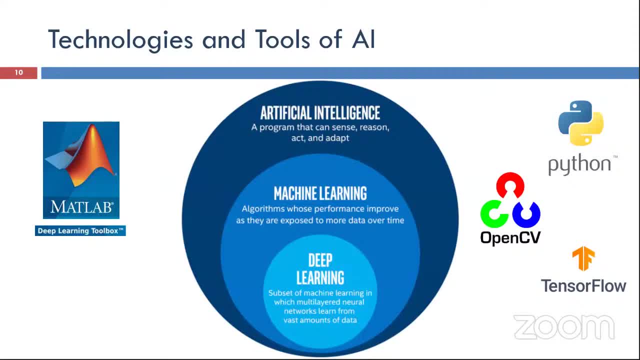 it means that now there will be, for example, a department of osteoscopic engineering, for example. I mean, I specialize in osteoscopic engineering, but I only do a Baccalaureate in artificial intelligence. So if I want to use a Baccalaureate in anything, 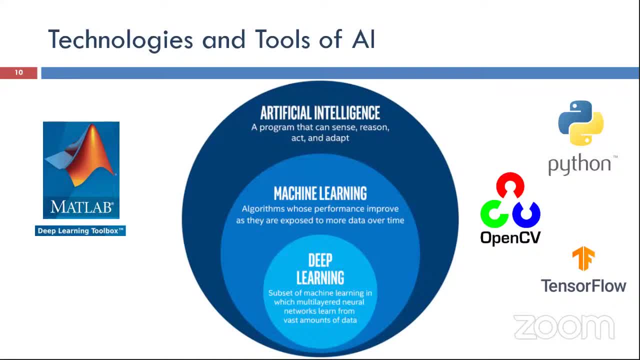 I mean, no one wants to use a Baccalaureate. I am a specialist in osteoscopic engineering. It is not possible. Electrical engineering and osteoscopic engineering for me are tools. Okay, So artificial intelligence is definitely present. 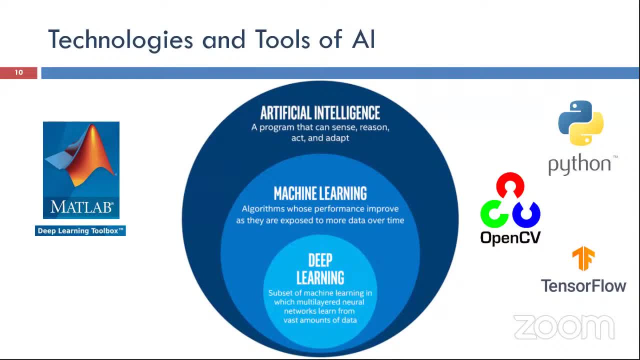 a lot now in the field of research And actually it is advised. I mean, in the field of medicine in particular, there are really good applications. So really it is a very good thing And you will find that. 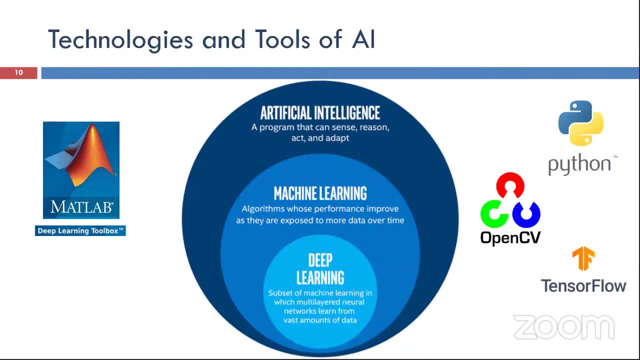 actually you will find a lot of resources that you can use. So actually the field is very open compared to the previous studies in the field of artificial intelligence. When you come from a specific background and you have your own problems, 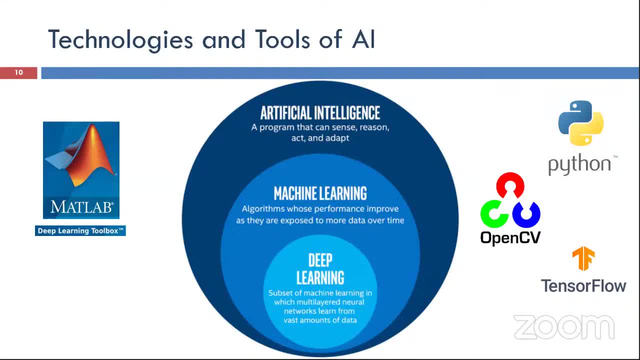 you want to solve them by using artificial intelligence Guys? regarding the preparation, the preparation link in the points, unfortunately for students in the Faculty of Engineering at the University of America in Al-Aziz, But in other universities and colleges. 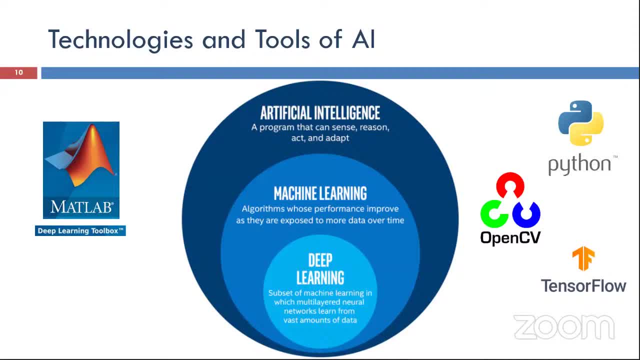 unfortunately it does not exist, Khaled, how? how did you prepare the students for the course that you can join and contact Al-Fara'a's account on Twitter? The second question is from Mubarak. He says: Dr Aqid. 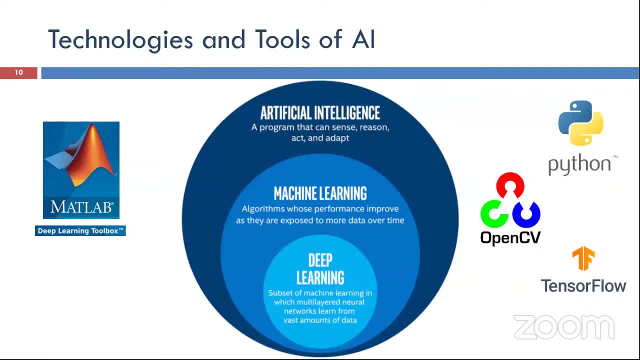 there is a lot of opposition from people about the use of artificial intelligence in medicine and their lack of trust in it. How can we convince people? First of all, you are in the stage of trough, of disillusionment. Okay, People see that people. 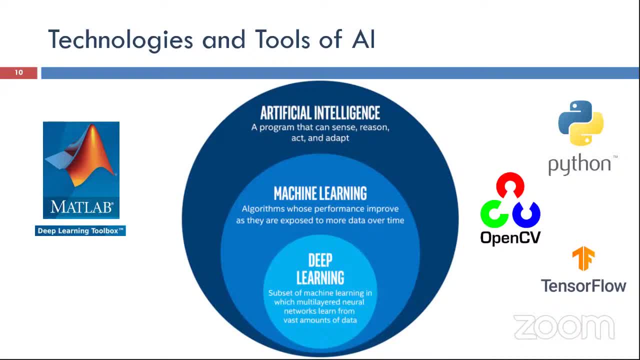 who talk a lot about artificial intelligence do not see anything. They still do not see an application. We see that artificial intelligence has really done something that nothing else has done like them. Okay, So in order to convince people, you need to have 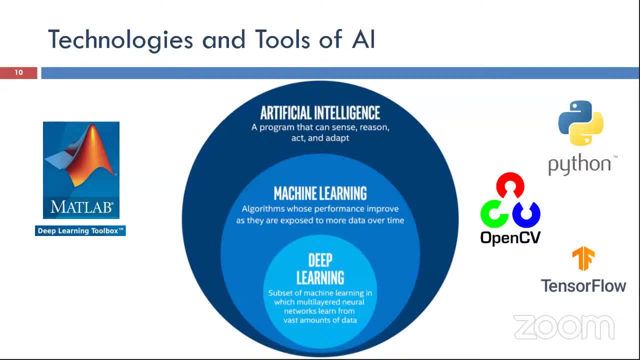 an application or product with artificial intelligence that really does something unique. Otherwise, people are convinced that something like artificial intelligence has achieved its potential. Okay, So you always expect people to be skeptical, especially in the medical field, because there is always skepticism among doctors. 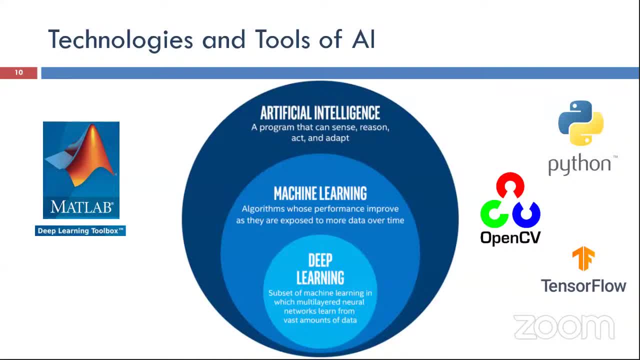 I mean, they always have resistance to new technologies. despite the fact that doctors nowadays are not doctors of the past, Doctors nowadays are actually leaders in artificial intelligence. Some of them are really leaders. Doctors of the past can tell you, for example, the CAT scan. 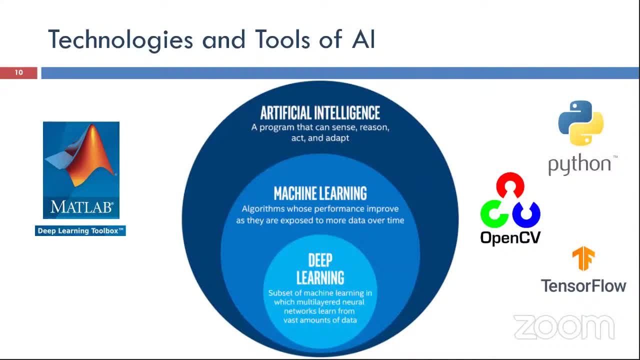 when it came out, the computer tomography. when it came out, people were satisfied and doctors were satisfied. They said that this is not useful. Okay, If you were convinced. okay, Basically, people at that time, of course, their resolution. 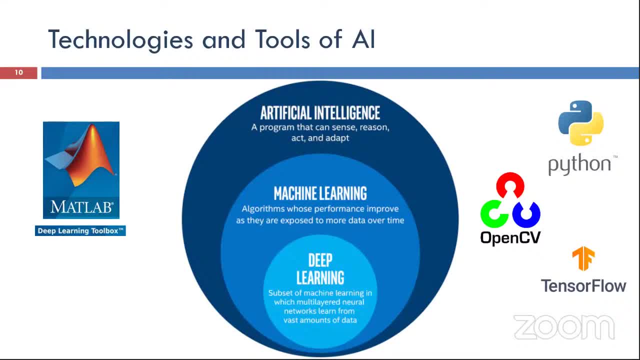 was not high, but their potential was not visible at all. People did not want to change from plain x-ray to computer tomography, So be careful when you talk about something like AI. AI is a concept because people talked about it in fictional fields. 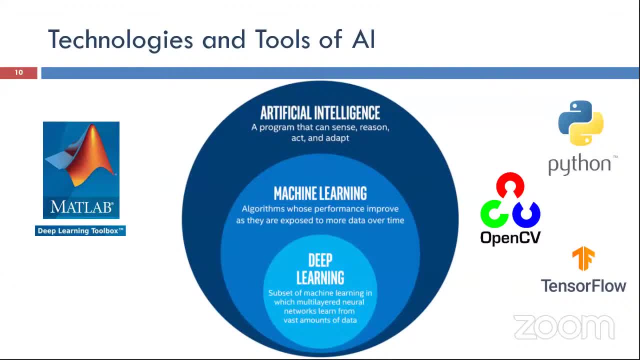 Basically, people became a little worried about it. When someone tells you to do something with artificial intelligence, people expect that this man is probably a hypocrite. Okay, So people started doing artificial intelligence and did not think about actual products. So 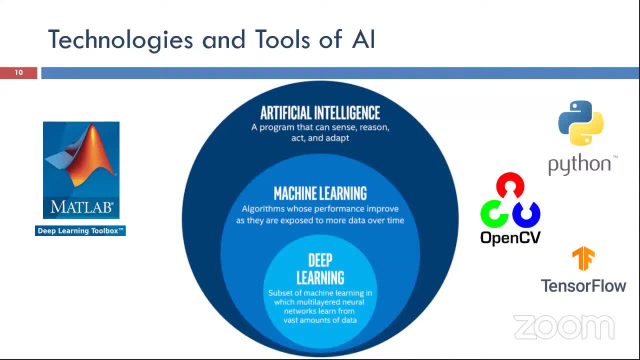 the solution to continue is that the first thing to do is to look at the actual applications that artificial intelligence can be useful in the hype. Then we start to use products or even tools to use artificial intelligence to help healthcare patients in a real environment. 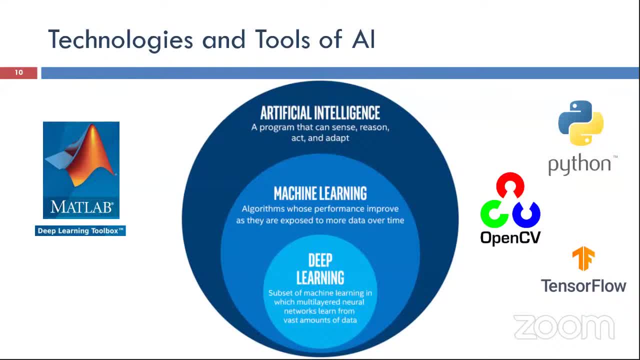 In fact, artificial intelligence is a product that is very successful in the world of artificial intelligence. So, in the world of AI, artificial intelligence is the most useful and the most useful tool for experimenting with artificial intelligence. In fact, artificial intelligence is a very 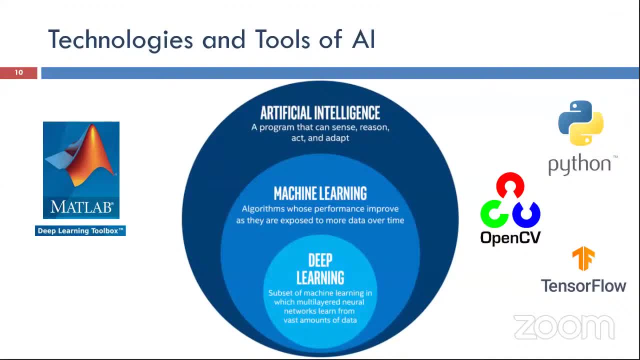 useful tool to So you can enter it alone on the AI system, picture by picture, and you will have a real-time identification. But at that time you are talking about what I saw in terms of ultrasound. people usually don't use the video to enter the AI. 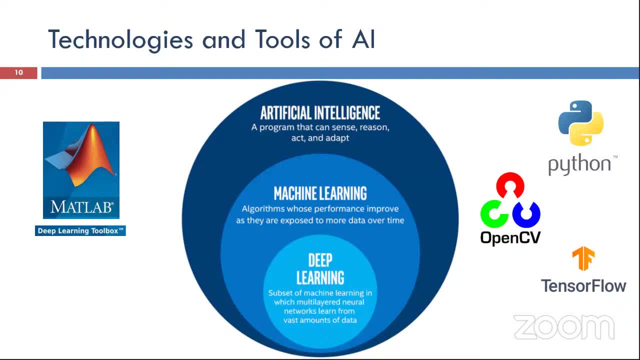 There are still many applications for this. Especially, as I said before, you have a sensitivity to learning with the settings of the device. Imagine that the doctor in the ultrasound holds the probe and goes to the patient's stomach to get pictures from different places in different situations. 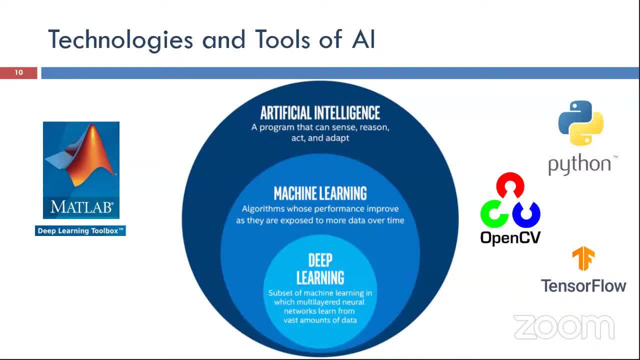 Therefore, in order to standardize the position of the probe, in order to give you the picture that your device teaches you, that your AI teaches you, it is not a logical idea. So what is present now is that you take pictures, taken with standardized positioning, and then enter them on the AI system. 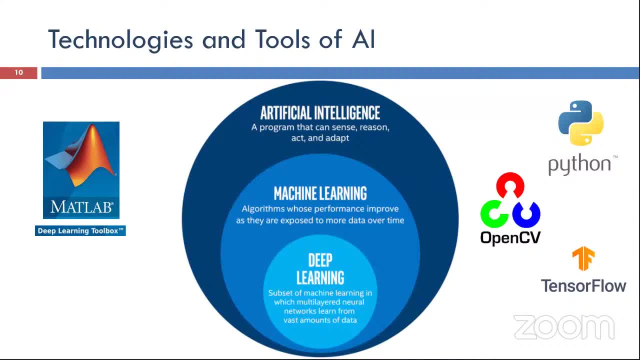 When the AI system reaches a stage where it creates a model, you train it in 3D, that is, you take a 3D model of the human abdomen, for example, and teach it. This is very difficult because you have to collect its data. 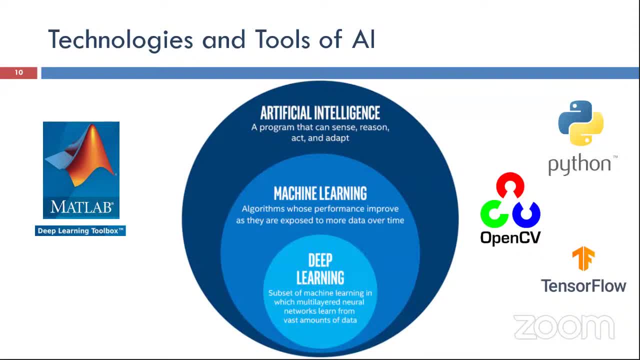 because you have to train it in 3D. that is, you have to train it in 3D. you have to train it for the learning of the Artificial Intelligent System. If you reach this stage, its quality will not be different. 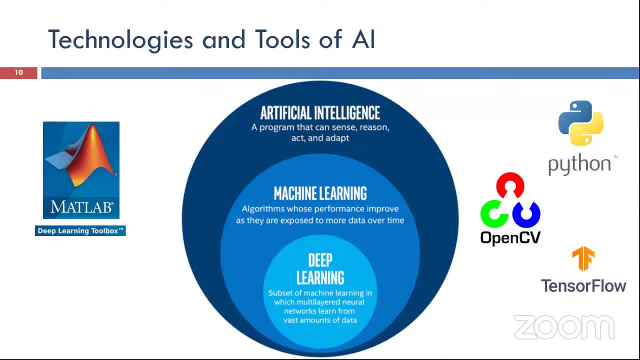 Its quality means you're able to take any position and even make a video and can take different positions and also check any frame in it properly. Thank you, prof. thank you for asking for the invitation and thank you for your time. also the tutors that I gave you the email.